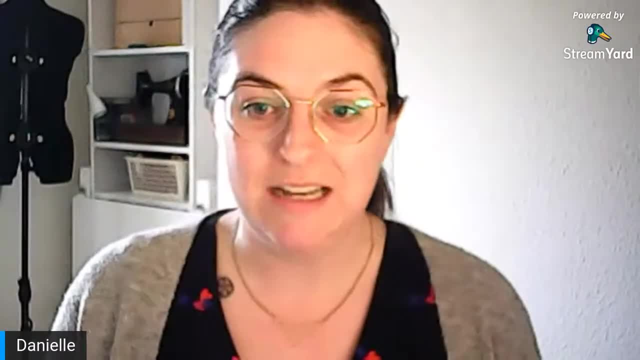 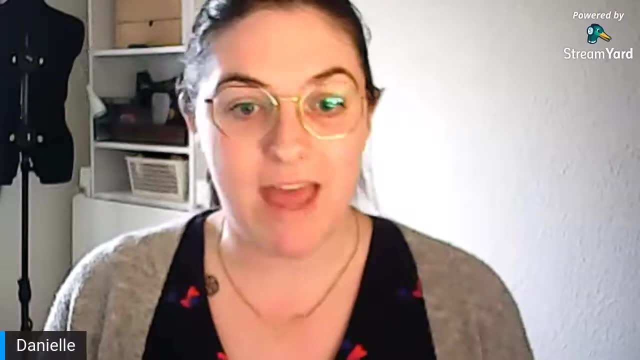 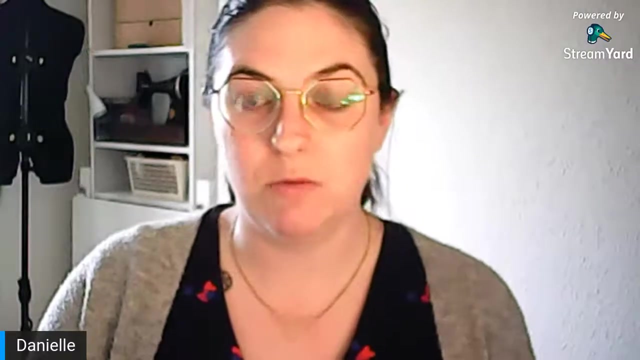 able to squeeze one final live streamed event in. We're busy trying to find a speaker at the moment. it's quite last minute. We normally book about a year in advance, So if any of you out there in internet land have got any suggestions for someone who you've seen speak and think was really great, 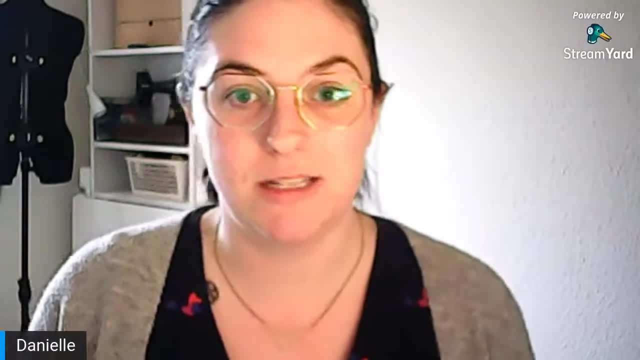 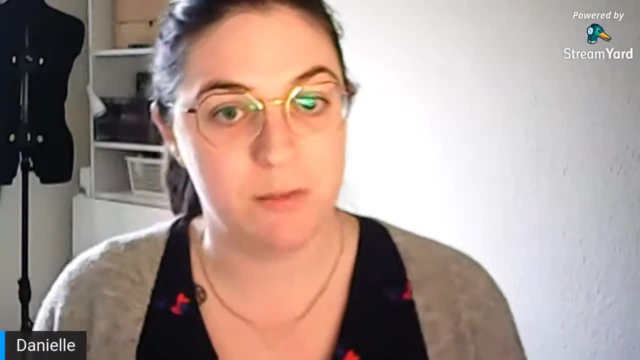 for our Society. please, please, get in touch and let us know and we'll try and see if they're free. Additionally, obviously, the festival is still going ahead in a much, much, much reduced format as usual. So it will be the 11th to 13th of June and they're really keen to get people involved. 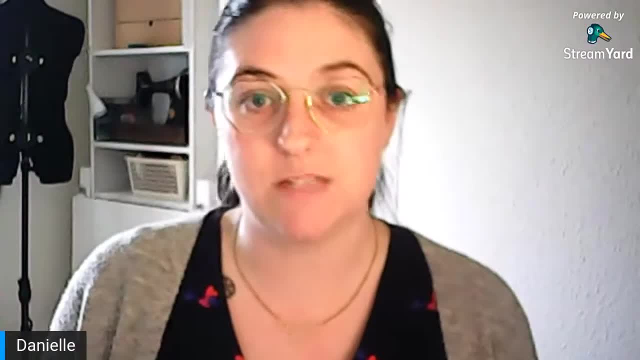 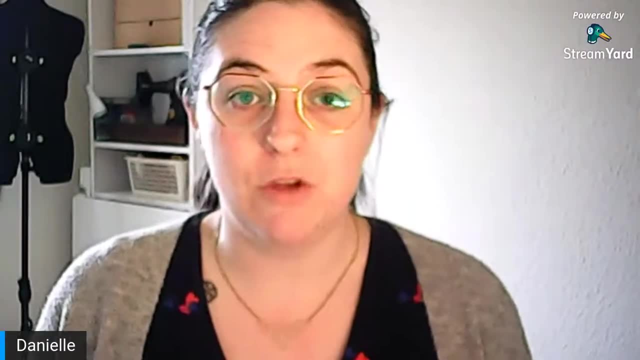 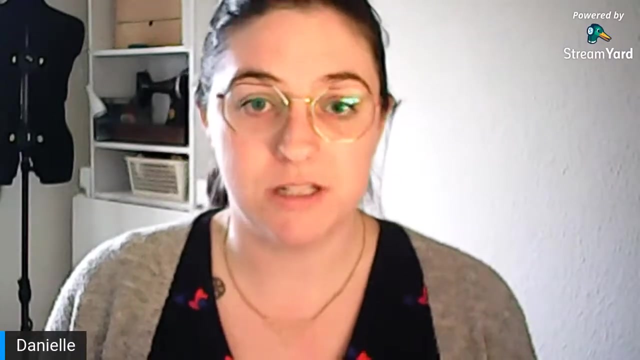 with their Psycash event. So head on over to the Atom Festival website, take a look at that and see if you want to get involved with that And similarly, if you would like to volunteer, please get in touch with myself or Susan to register your interest for any volunteering. 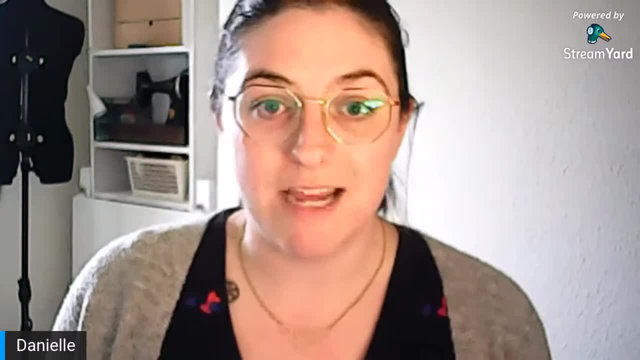 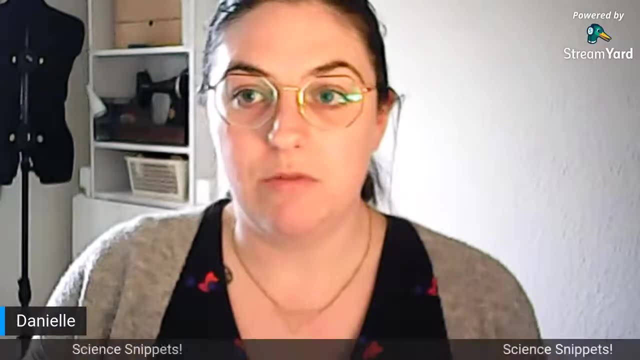 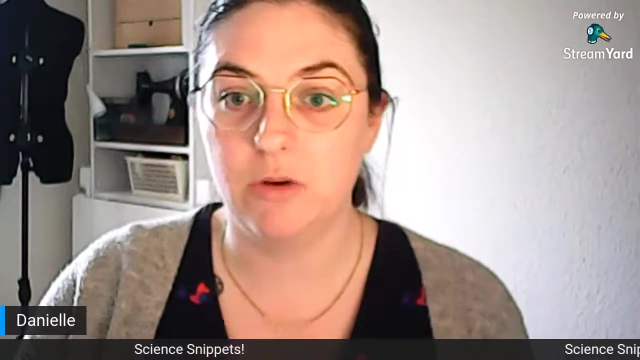 That may be required, and Susan will be able to let you know if you'll be needed. Okay, so before we move on to the main event, it is, of course, time for this month's science snippets. So if you have any snippets lined up for us, please do let us know. I've got one myself, but I know. 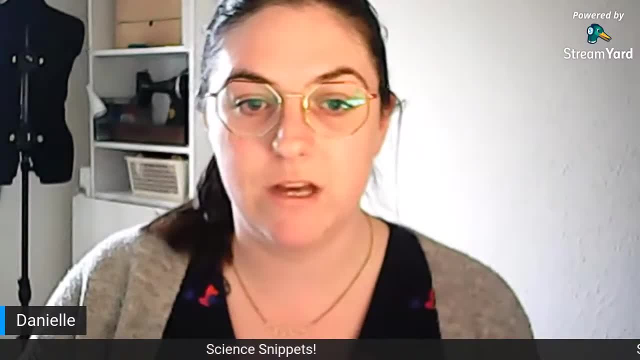 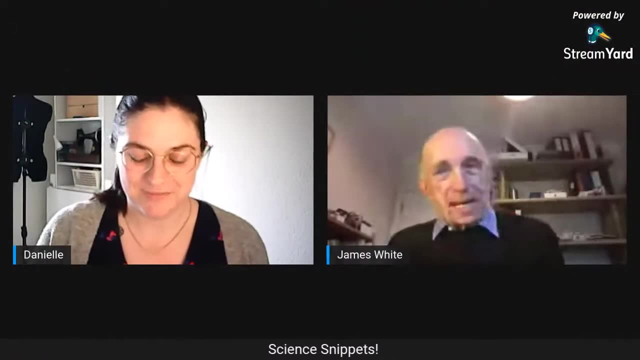 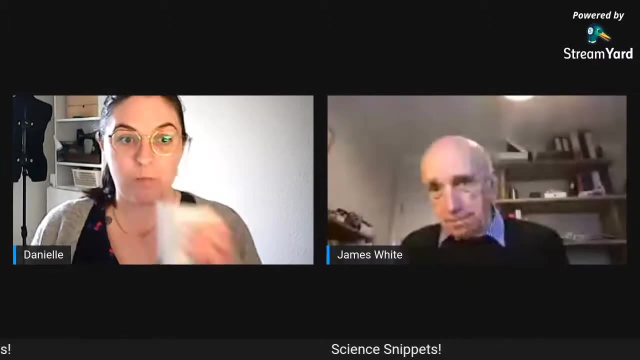 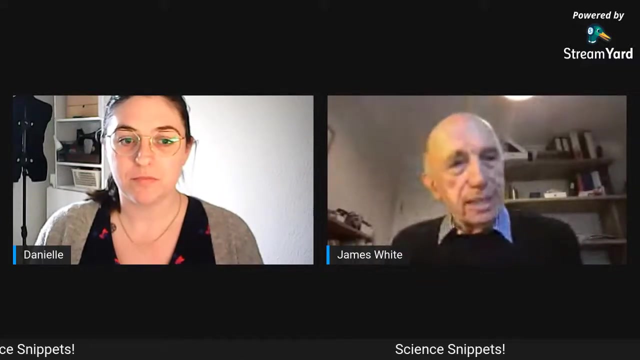 that James has got a couple, so I'll bring him in first. James, what have you got for us? Yes, hello everybody. I've got a couple of snippets for you today. One is from Japan and one is from Sweden. Let's have all the genes one. It's associated with science, but not quite involving a scientist. 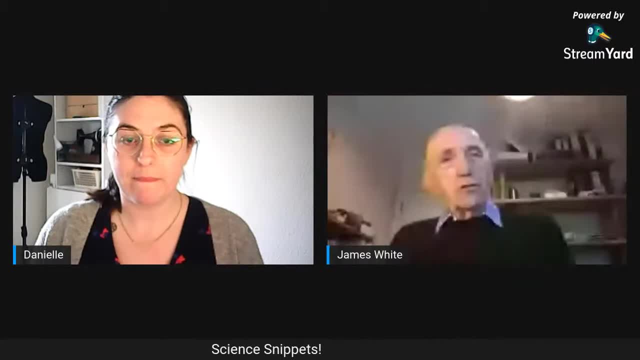 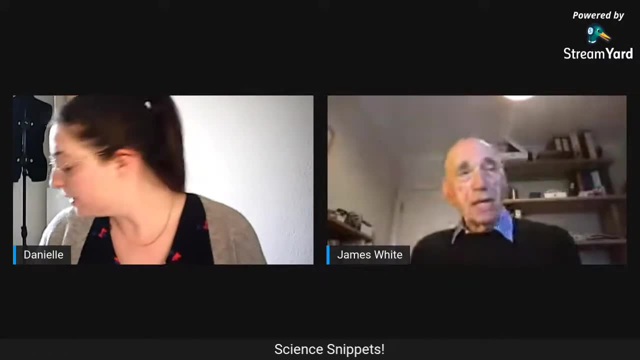 Anyway, there's a philosopher and writer in Japan called Yokio Hirose, who has an office overlooking a village square or town square in Japan- somewhere I'm not quite sure where it is, And overlooking the square. in the square there are a number of statues, mainly bronze. 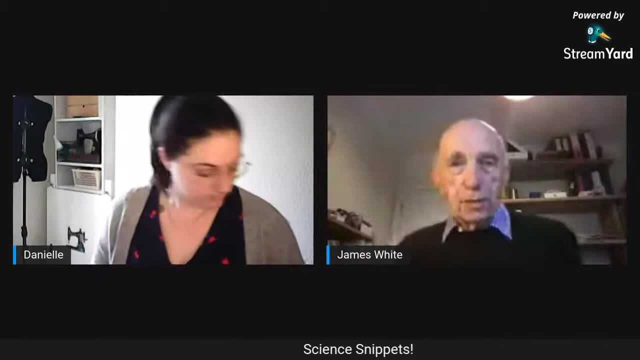 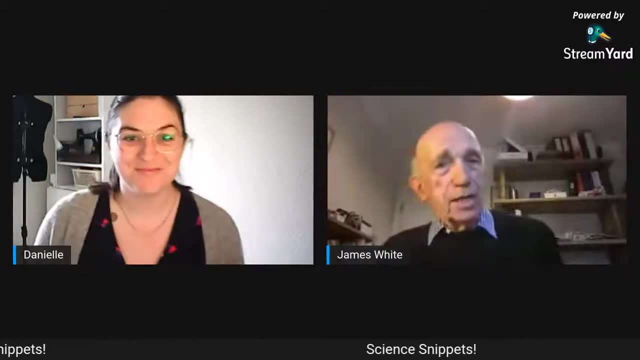 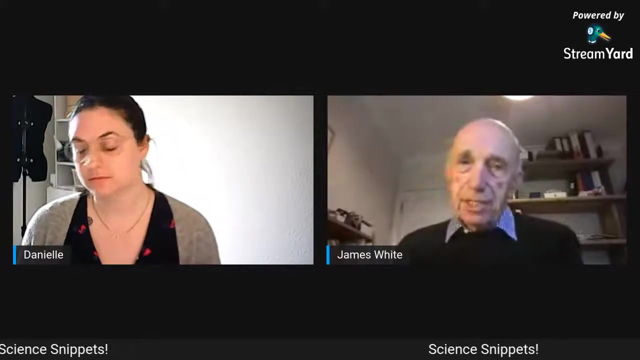 statues And he noticed that all the statues bar one were covered with pigeon droppings. He wondered why the one that wasn't covered wasn't covered. So he had a friend who was a physicist or chemist rather, and they managed to get a sample of the material that the statue was made from and 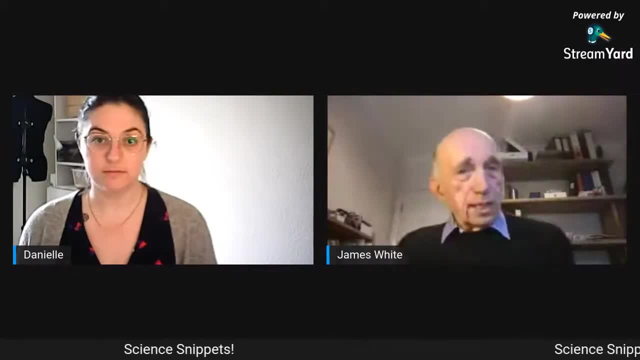 tested it And they found that, as well as the normal copper and tin bronze consists of, it also had about a five percent content of arsenic. They thought, oh, this is interesting. And they knew a sculptor who'd been commissioned to make another new statue for the same square And they got in touch with him and said: look. 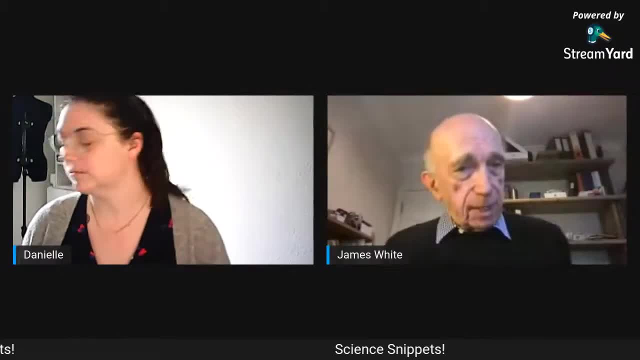 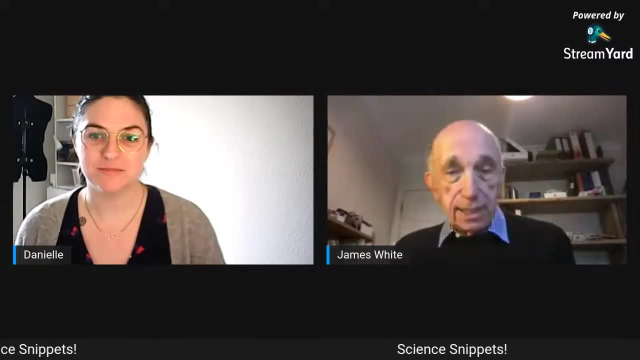 when you make this thing, would you put some arsenic into the mix And let's boost it up a little bit? So they put 10 percent of arsenic into the mix to make this new bronze statue, And they did, and the statue was erected and not a single pigeon sat on it. 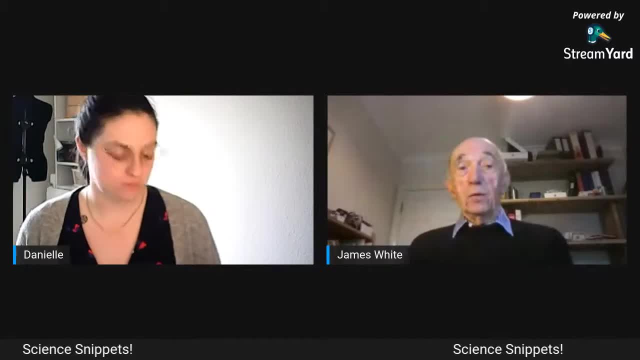 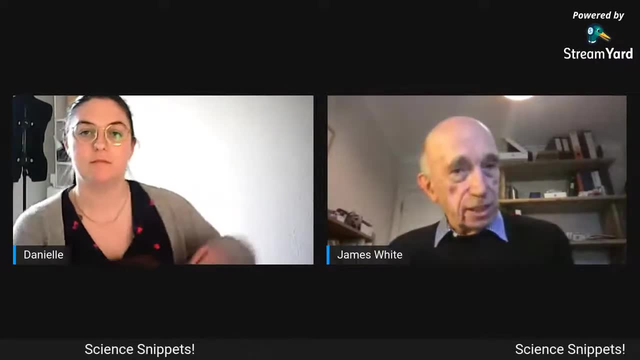 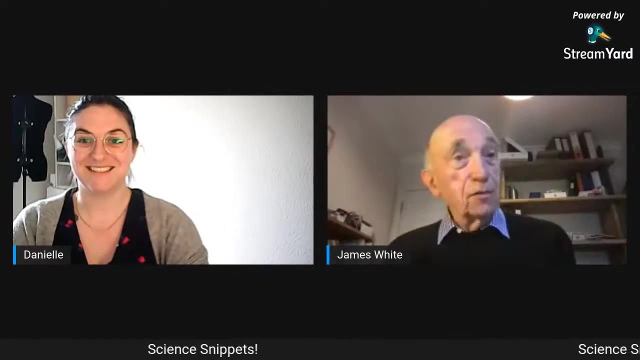 So it obviously worked. So well did it work, that the local authority decided that they would now commission all future sculptures in the town made of bronze to have this content of arsenic. So my advice is, if you're going to go to Japan and see some statues, don't touch them. What if you do? 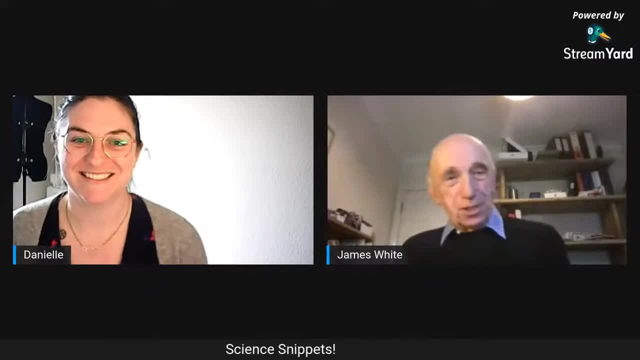 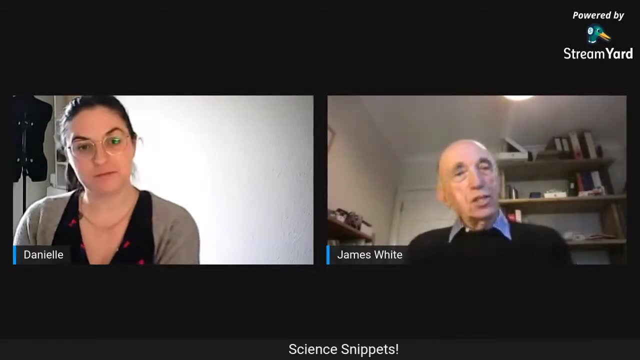 No licking of statues. My second one is more zoological and this is to do with Lund University. some researchers in Lund University, and that's one that appealed to me. They were researching into the communication between certain animals, In this case it was crocodiles. 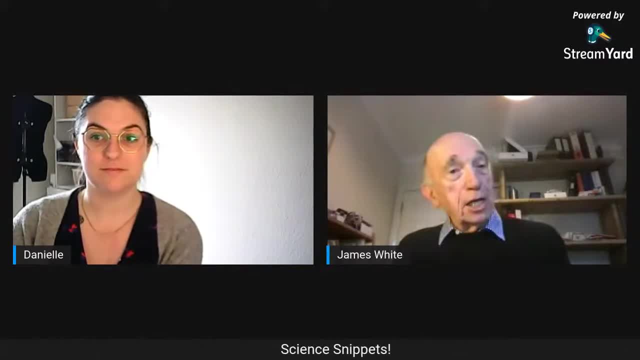 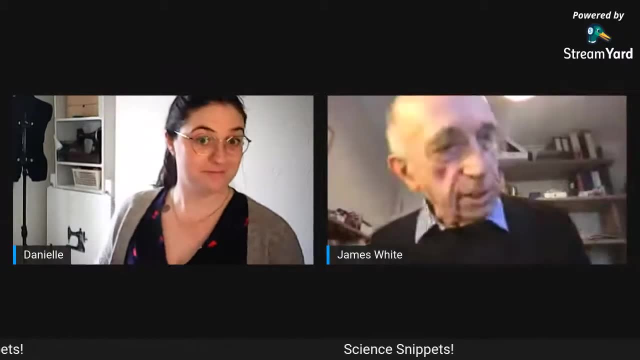 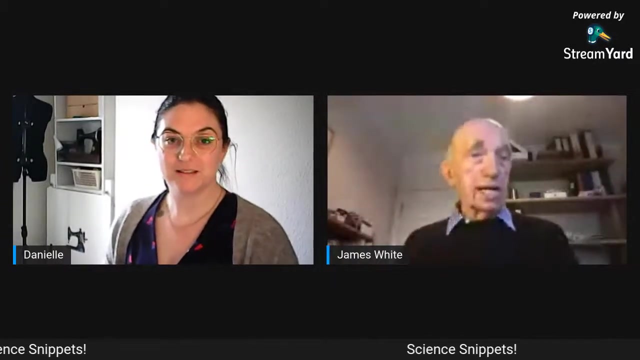 I wanted to see whether they had a feeling that the depth of the sound of a male crocodile- in wooing moods, shall we say- may have an effect upon the females. And so they got hold of a male, put him in a large tank with a recording device, and they first of all filled the tank with air. 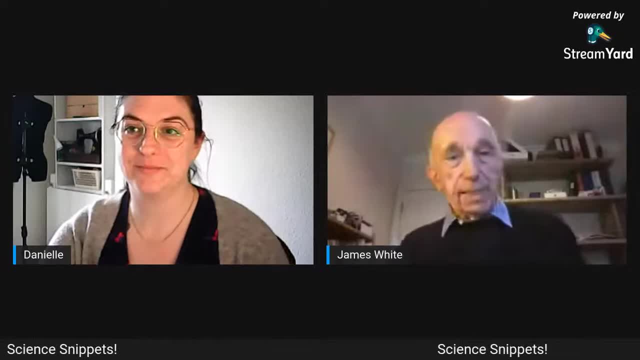 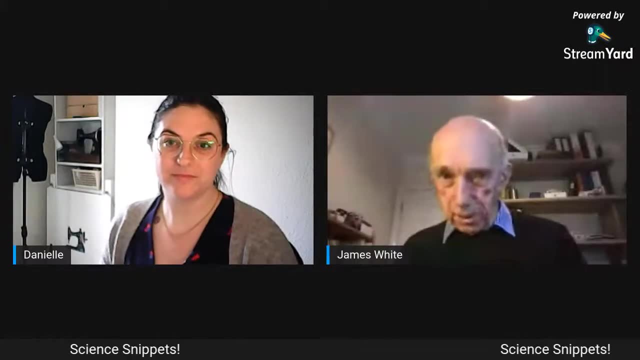 ordinary air and they recorded his voice. Then they put in a ten percent mixture of helium into the tank. You know, if you breathe in helium your voice gets a bit squeaky. You've probably tried it some time or another, And so it was with the crocodile. 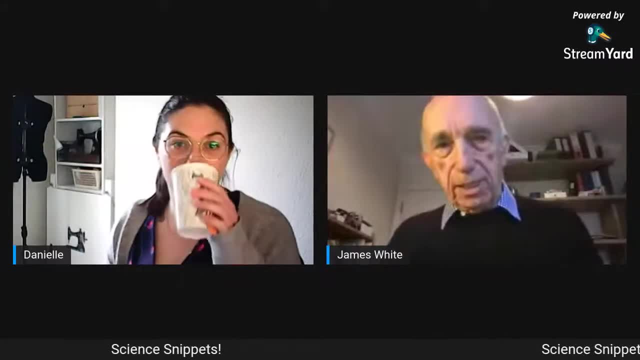 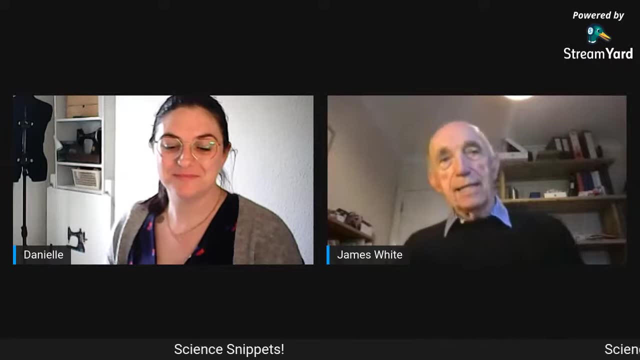 So this big bald crocodile, now with the helium mixed in his lungs, made a slightly squeakier croaking sound, raw, and they recorded that as well. Then they let him go, I suppose, and they played recordings of both the normal voice and the squeaky voice. 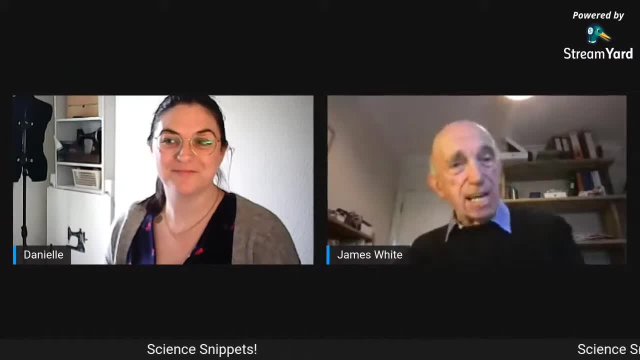 to a bunch of female crocodiles in a zoo, expecting, of course, that the females would prefer the deep throaty roar of the big male. They got exactly the opposite result: They preferred the squeaky voice. So if any of you men out there are feeling amorous, 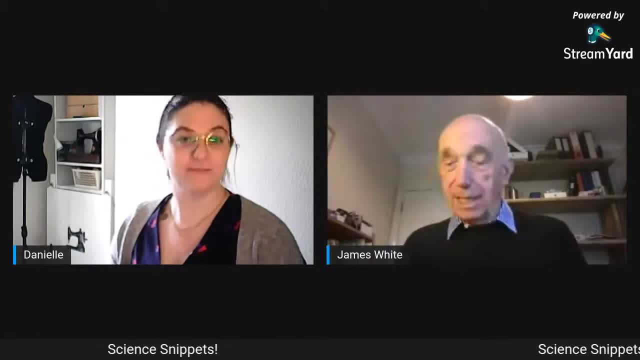 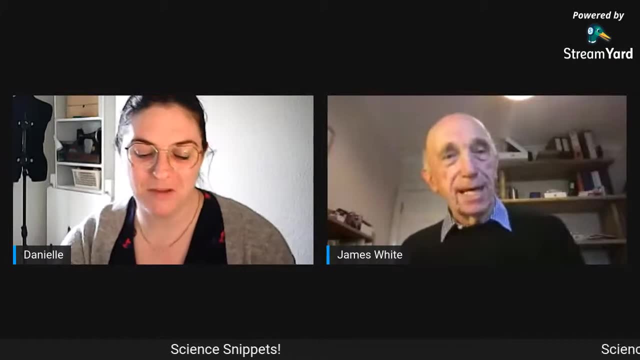 and you've got a squeaky voice. don't worry, you'll be fine. Okay, that's it, So back to you. Thank you very much, James. That was great. We haven't got any time. Bye, Bye. 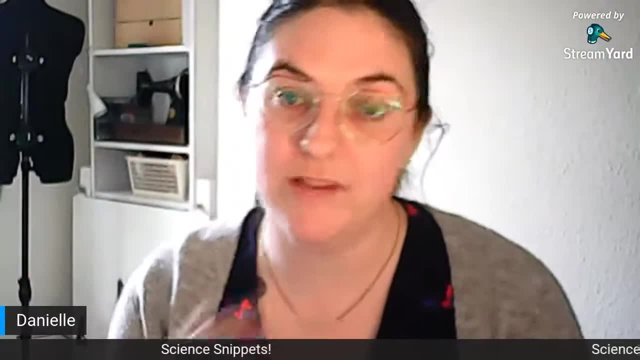 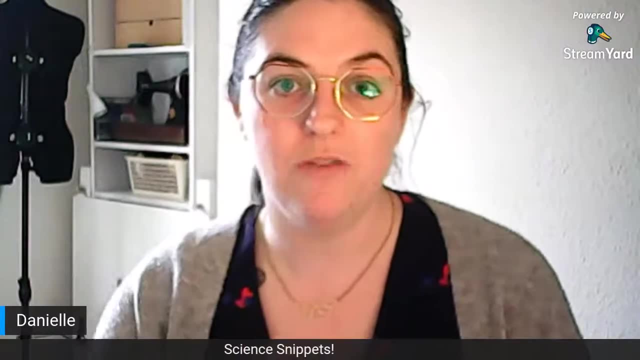 We haven't got any coming through on the chat just yet. If you do have any and you don't make it through, I'll try and come back to you later today. I do have one myself, Obviously. the events of the past year have highlighted 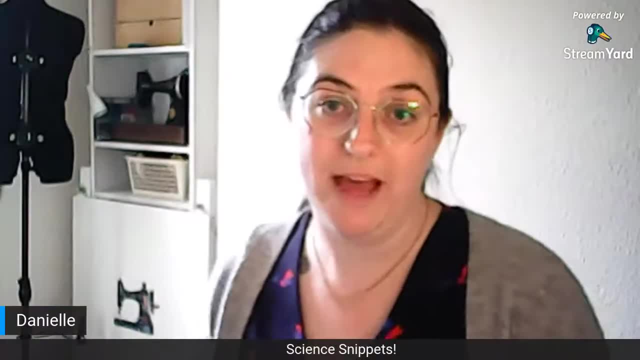 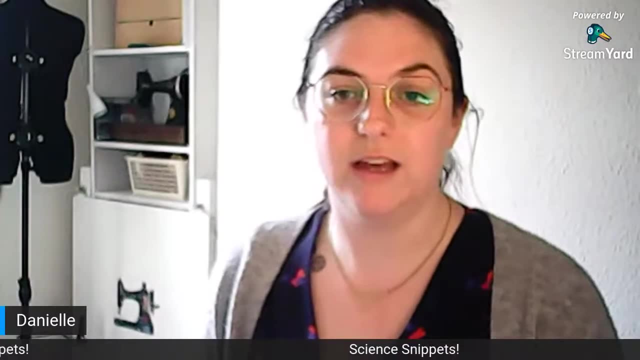 a particular hospital procedure to a lot of us that we maybe hadn't thought about before, and that would be ventilation, So a process to help someone breathe when they're having lung difficulties. But the process of ventilation is quite, quite violent actually. 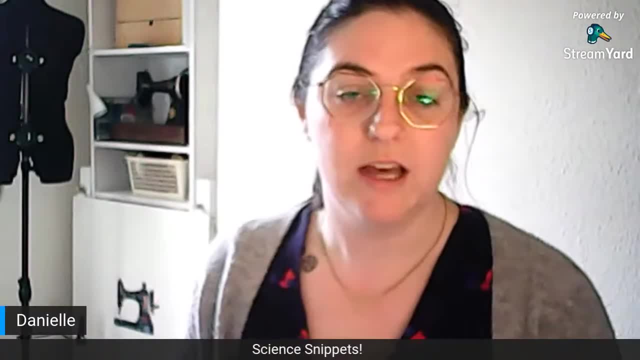 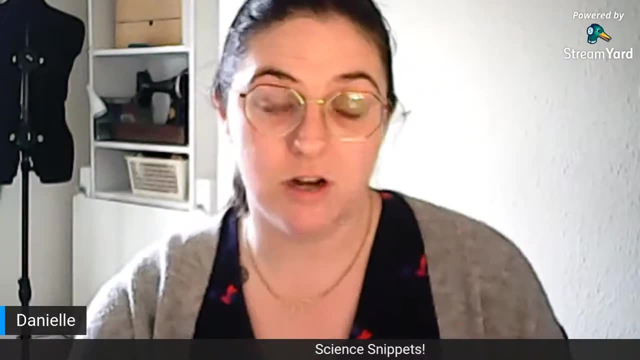 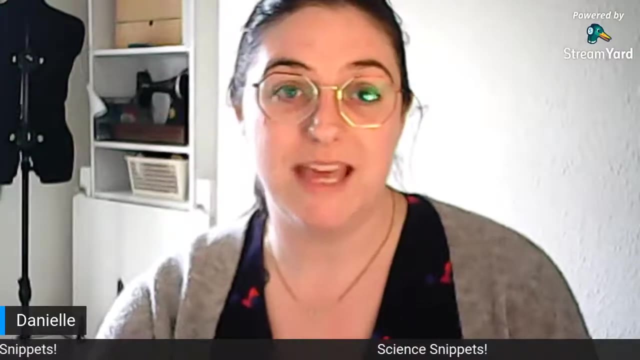 and it can be very damaging to what is otherwise very sensitive lung tissue. Now researchers in Tokyo think that they may have found an alternative way to get oxygen into our system. They have discovered something in pigs that they think may also work in humans. 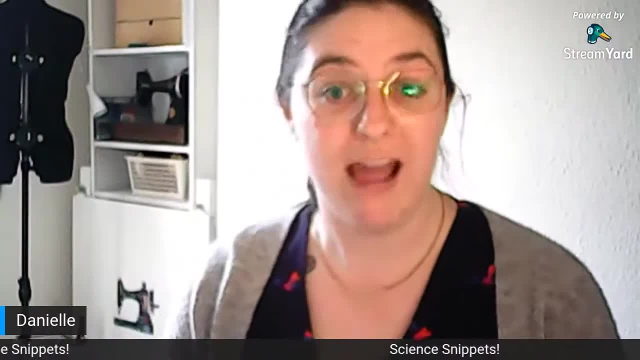 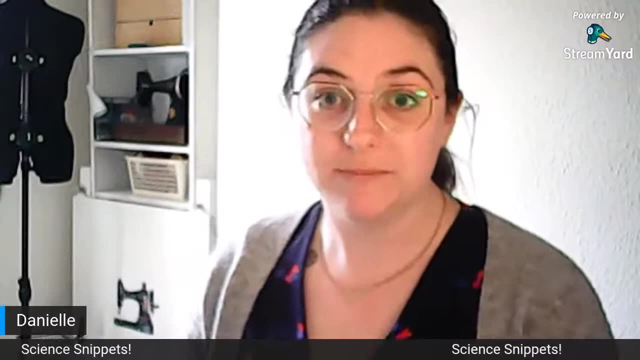 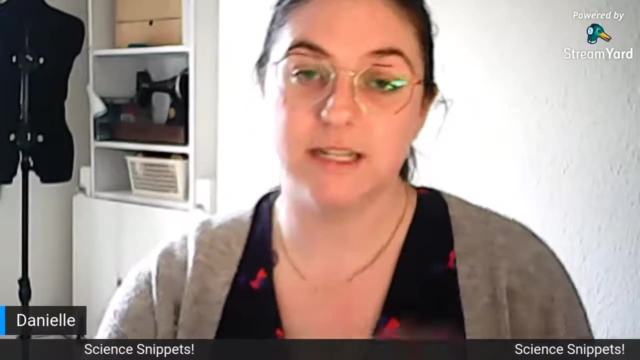 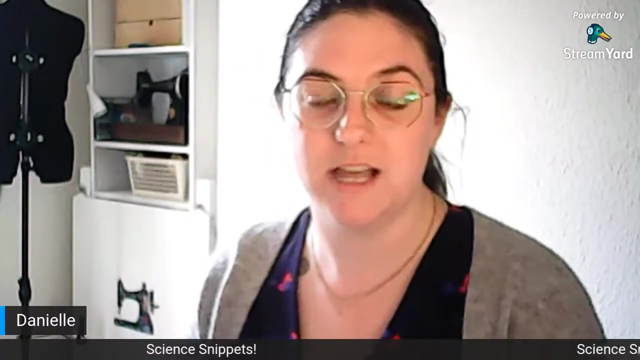 and that is, they are able to breathe through their rectum. So with the A they're made of an oxygen-rich liquid. They submerge the back end of these pigs in this liquid and then they decreased the oxygen available to them via their nasal passages in their lungs. 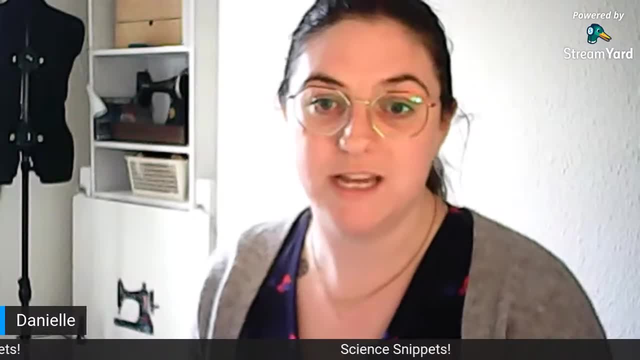 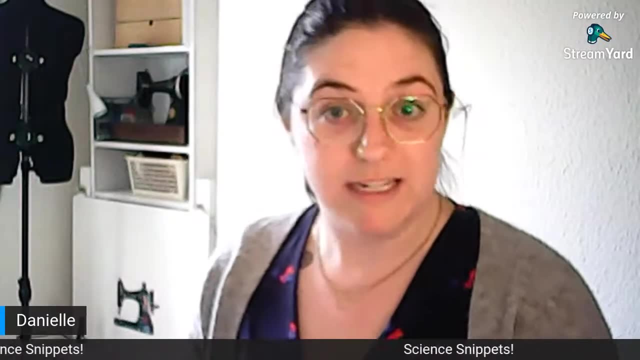 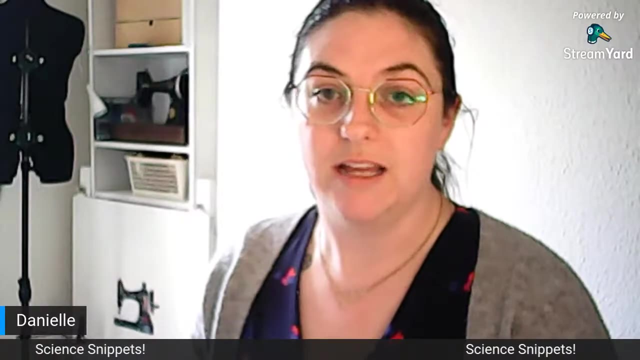 and they found that the pigs were able to get the oxygen they needed from this liquid through an alternative orifice. It's very early days as to whether this would be applicable for humans, But yeah, an interesting insight. Oh, I'm getting something through. 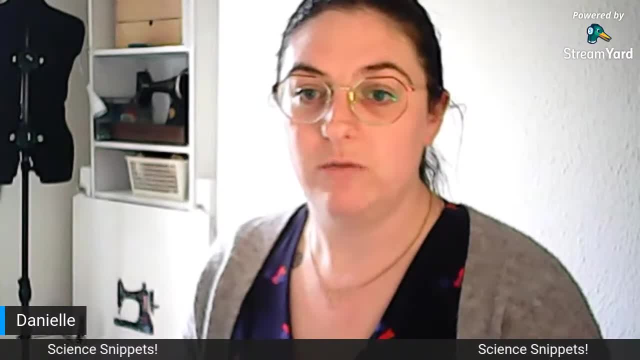 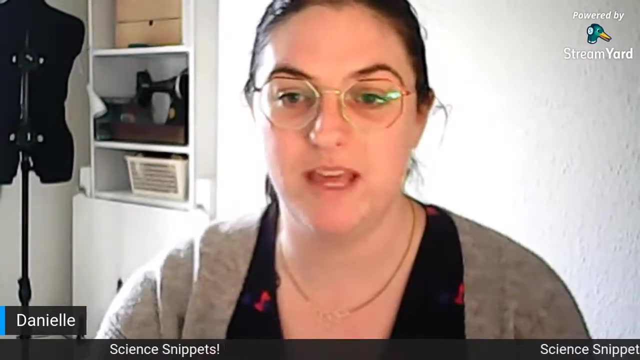 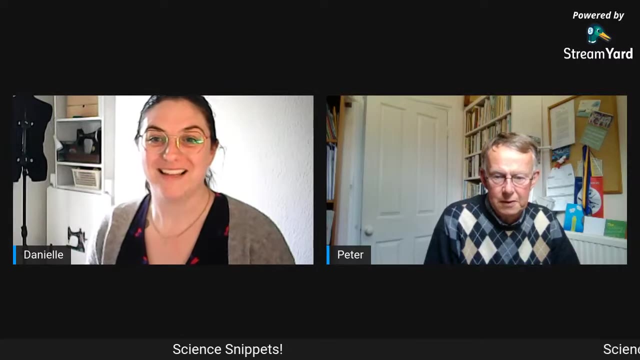 Peter, do you have a snippet? Do you have one you wanted to share with us? Wave, if you have one, Okay. so Peter also has a snippet. Just bear with me, There we go, Hello, Hello. Okay, let me see where I can do this. 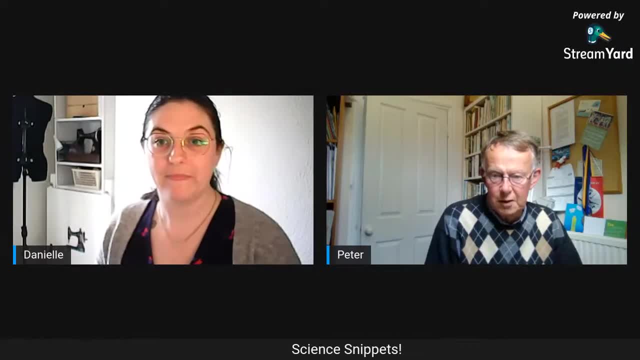 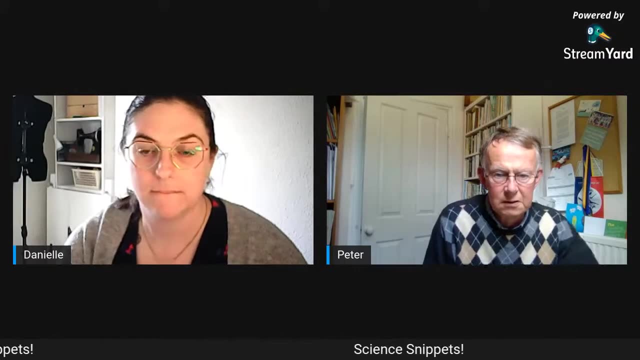 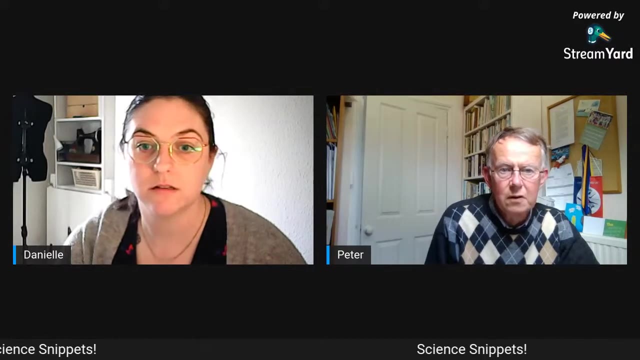 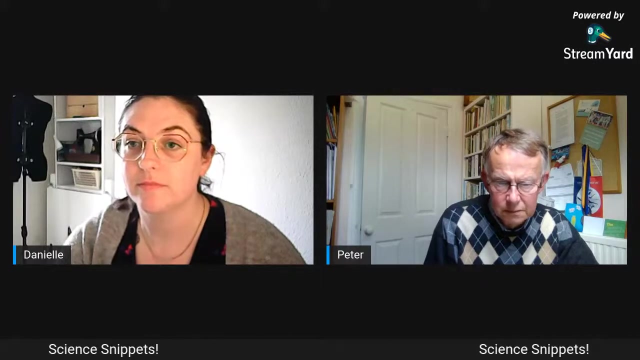 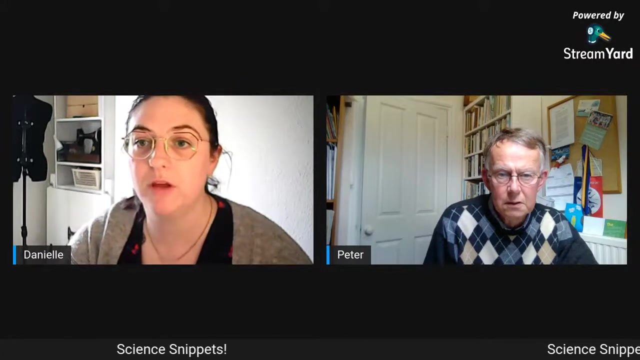 Right, I hope people can see that You're not sharing your screen, Peter. Oh, okay, I don't know what I want, Right? All right, Just while Peter locates his screen, I've had something come through from Bob. 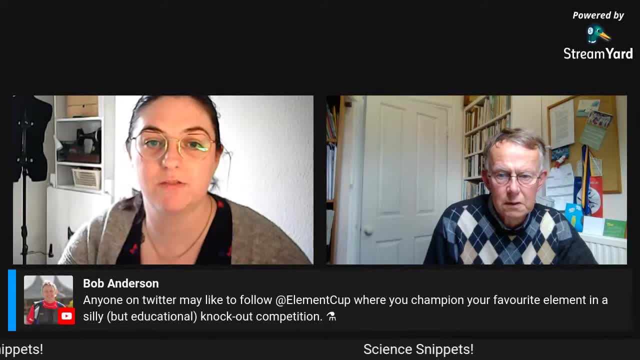 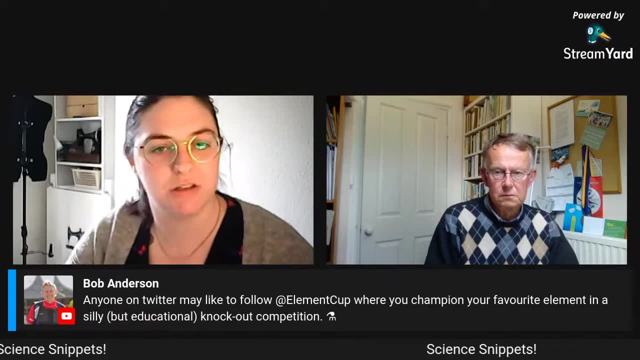 who says that anyone who is on Twitter may like to follow Element Cup at Element Cup, where you can champion your favourite element in a silly but educational lockout competition. That sounds quite fun. Okay, Peter, I have your screen now. There we go. 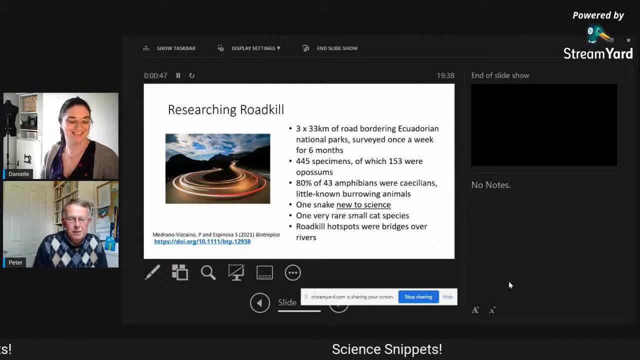 Okay, yep, yep. So this is slightly gruesome, but I did notice this short article from a couple of researchers in Ecuador, also zoological. They were um surveying these sections of road alongside a national park, a couple of national parks. 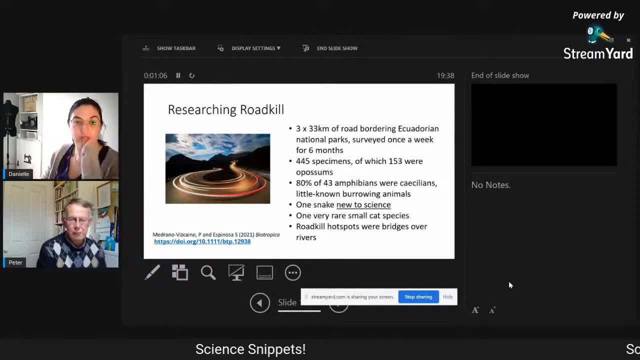 And although that's not a very random way of sampling, they identified all the roadkill that they found. About a third of the specimens were actually opossums. I don't know if you know, but in New Zealand opossums are an invasive species. 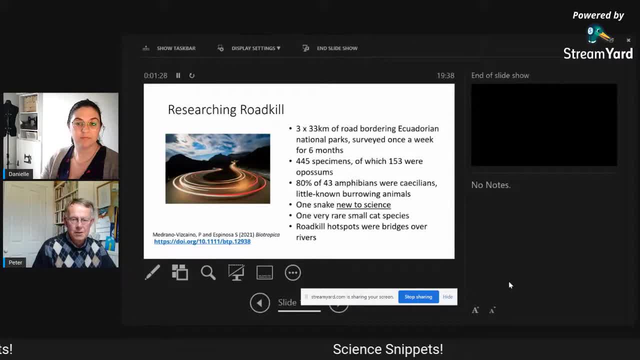 which are widely disliked because of their tendency to rob birds' eggs and everything else. Indeed, there are chocolate sweets in New Zealand called posh possums, which are shaped like a possum which has met its end under a car. They also found these little-known Sicilians. 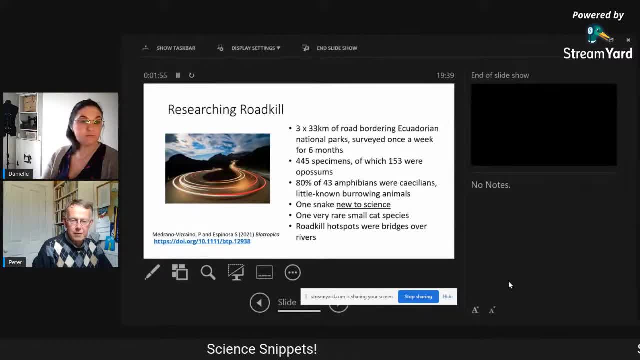 which are. They're actually amphibians, but they don't look like other types of amphibian because they don't have any legs And actually it's quite difficult to tell which way they're moving, because they look like shiny earthworms. 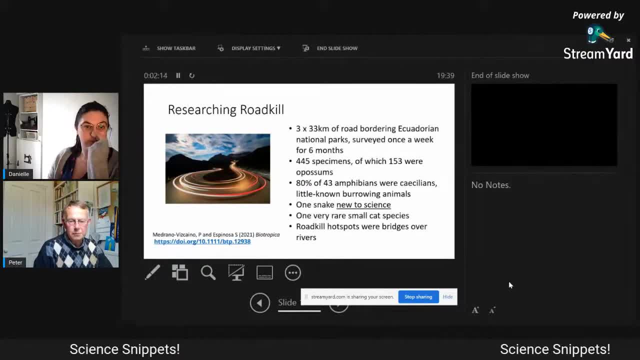 They also identified or made a discovery of this snake that was new to science beside the road. One unfortunate demise was a very small but rare cat from that part of the Ecuadorian jungle, And so they thought about some ways of trying to reduce the effect of the road. 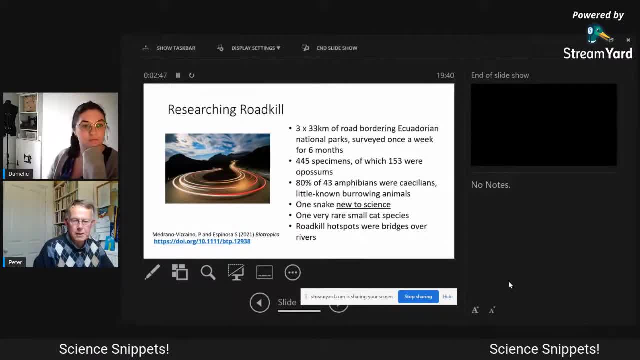 on the local fauna. but unfortunately, the places where the roadkills were most common was indeed the bridges over rivers, So it seemed likely that the animals were using those bridges to get across rivers they wouldn't otherwise be able to cross. So the research continues. 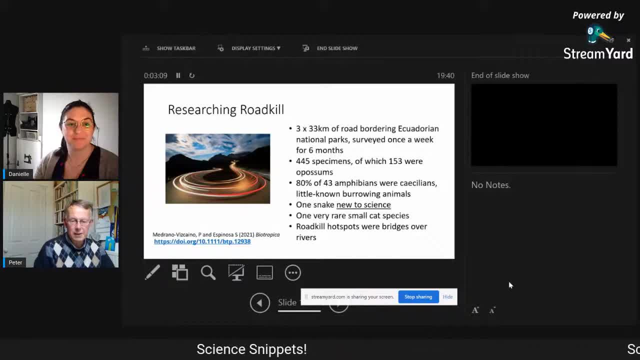 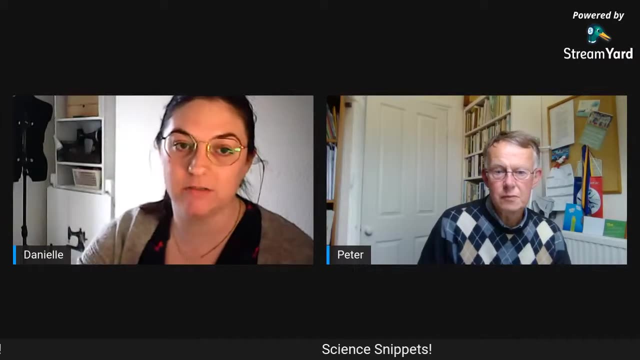 to find out other ways in which they could mitigate the effect of rushing cars, I'll stop sharing and hand over to someone else. Thank you very much, Peter. I know I quite like the little, the little subways that you can get under roads. 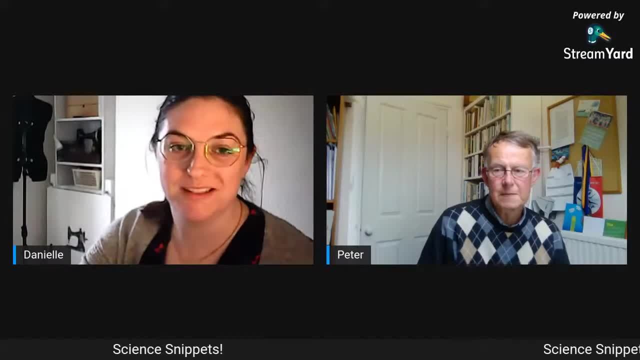 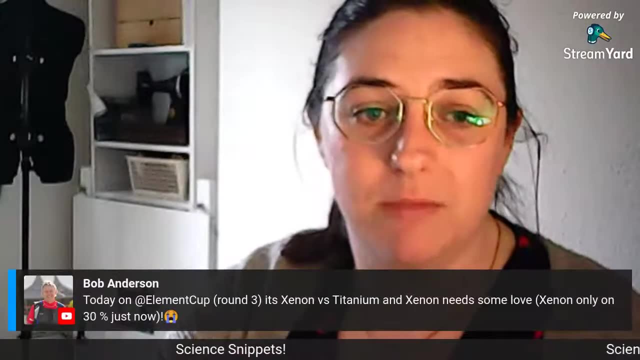 for badgers and hedgehogs and things. They tend to work quite well, But I'm sure the research is up on it. Thank you very much. Just following up from Bob's recommendation for at Element Cup, He says that it's round three today. 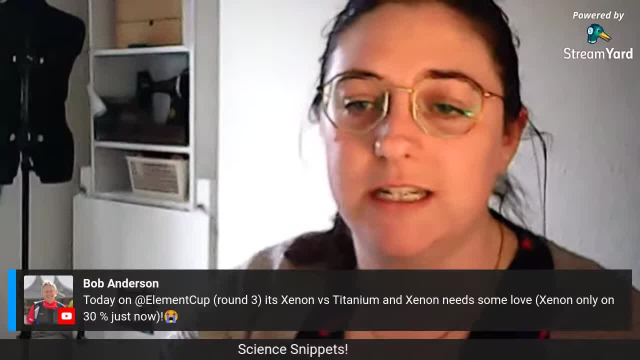 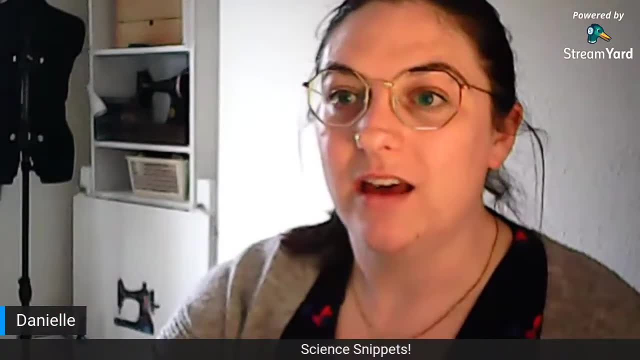 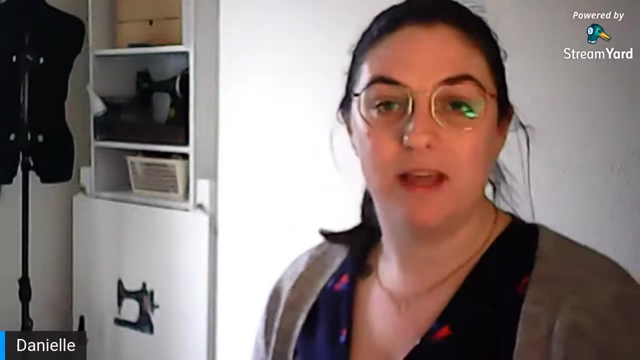 It's xenon versus titanium, and xenon needs some love, So you guys need to go over and vote for xenon. Okay, So without further ado, we will move on to the main event. So yes, this evening we have a really, really interesting talk. 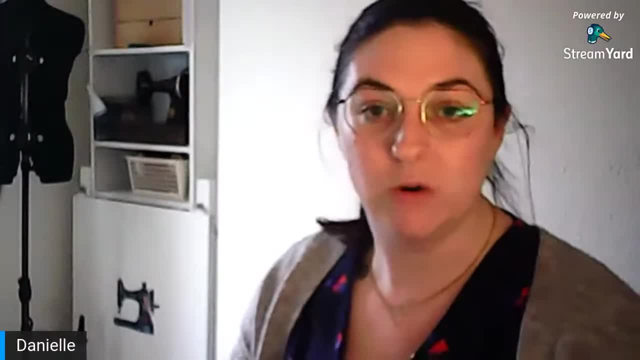 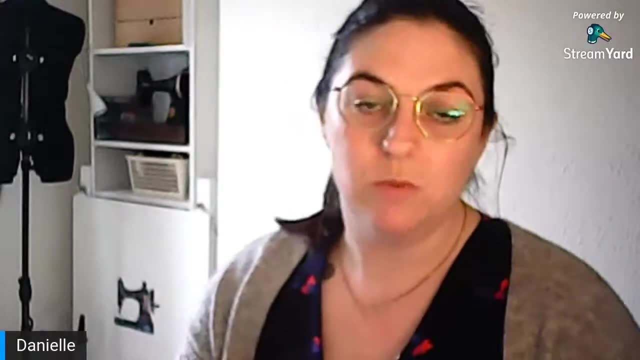 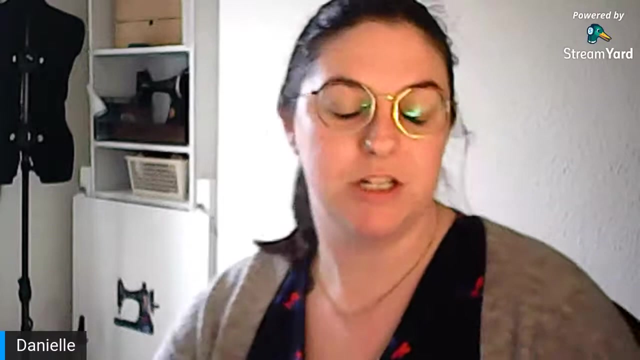 lined up from Professor Nick Hawes. Professor Nick Hawes is coming from us as an associate professor with the Oxford Robotics Institute as well as a tutorial fellow at Pembroke College. He completed his PhD in artificial intelligence at the University of Birmingham before going on to have. 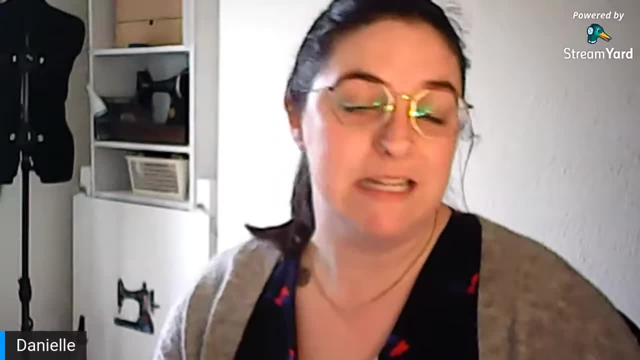 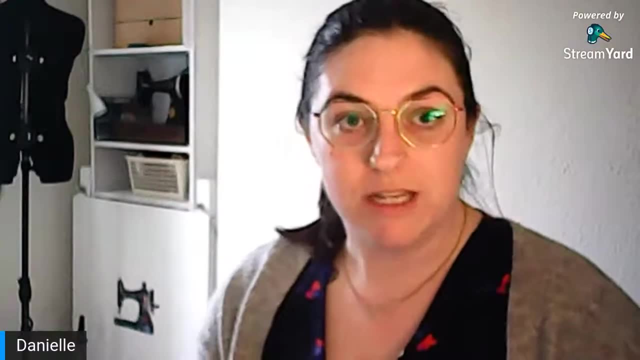 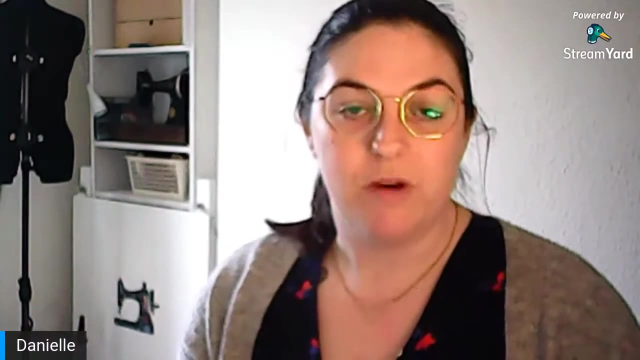 post-op positions both at the media, MIT's Media Lab Europe, and then at the School of Computer Science at Birmingham, And he has led his own team since 2009,, researching artificial intelligence as applied to robotics, before heading on over to Oxford in 2017.. 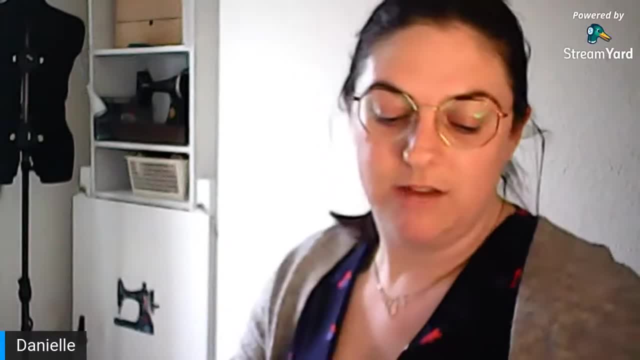 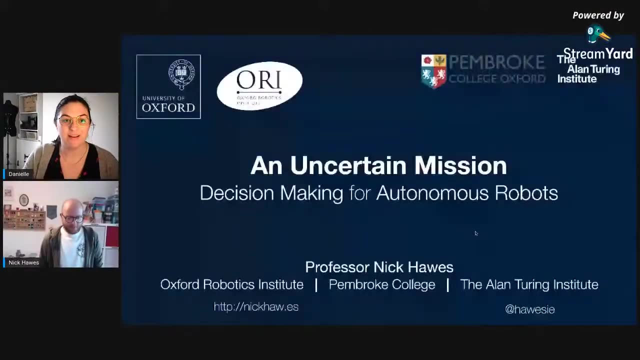 So we're really excited to hear his talk this evening on an uncertain mission: decision making for robots. I'm going to bring him into the screen now. There we go, And thank you very much, Nick. Hello, Cool, Awesome, Can you hear me? 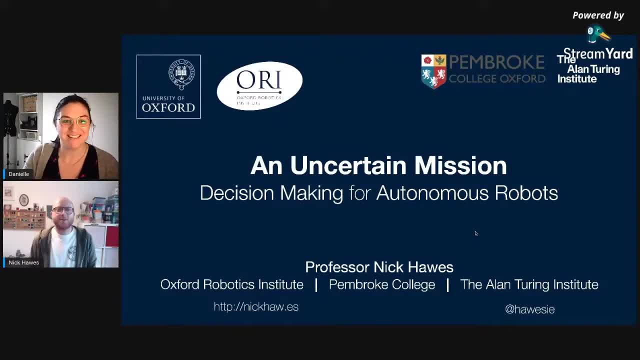 Is that working? Yes, it is working. Super exciting, Cool. Thank you for the introduction, Danielle, And it was awesome to hear all of those science snippets. So, yeah, my name is Nick. I'm an associate prof in the Oxford Robotics Institute. 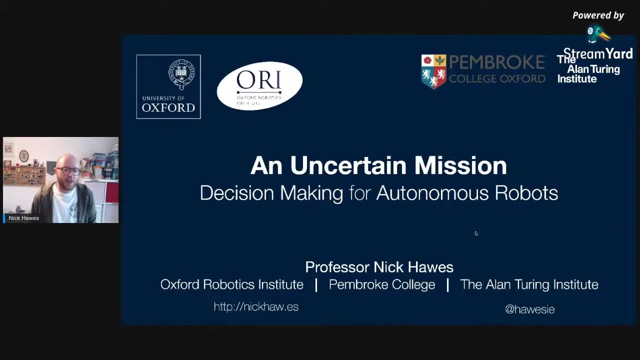 where I lead a group that does research on decision making for robots. I'll say a little bit more about that when I get to it. I should also warn you that I'm using you all as a bit of a sort of a test run. 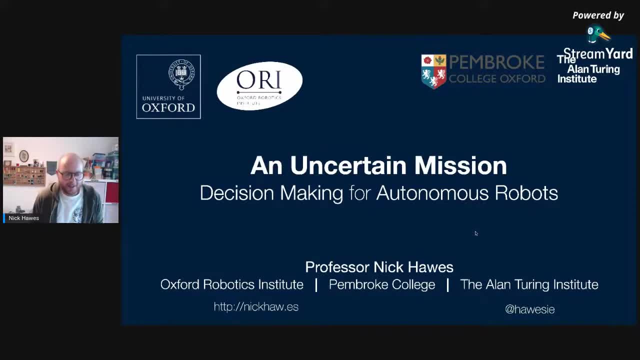 So this is the first time I've given this talk to anyone really, So it might be a bit rough around the edges, but I thought you'd seem like a friendly bunch to sort of try something slightly new with. So yeah, I'll be interesting. 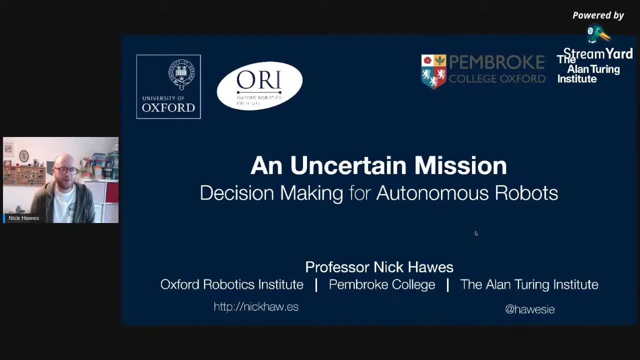 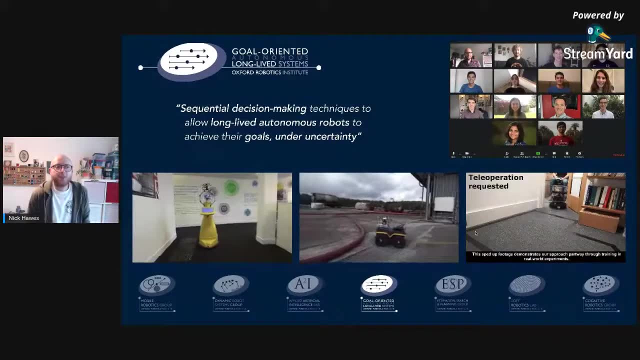 to hear your feedback towards the end, And I'm happy to take questions kind of as and when you've got them. So I work in a leader group that works on what we call sequential decision making. So that means we have a set of tasks. 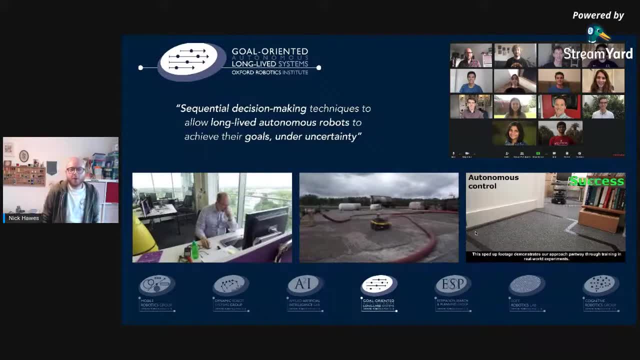 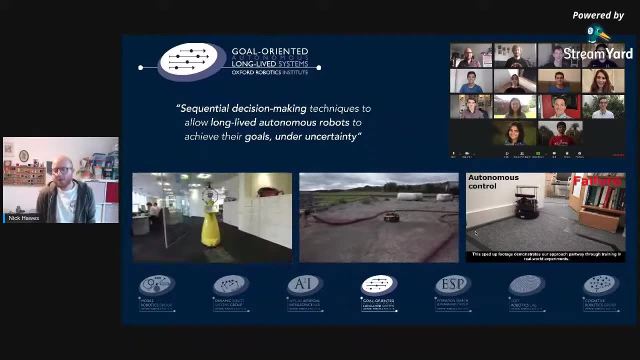 that we have to do, And the way to think about that is: we want to control our autonomous robots to solve problems and complete tasks for us humans, And to do that, a robot typically needs a sequence of actions it can perform in order to achieve a goal. 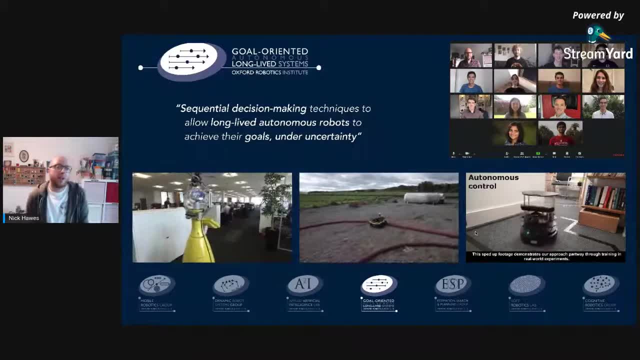 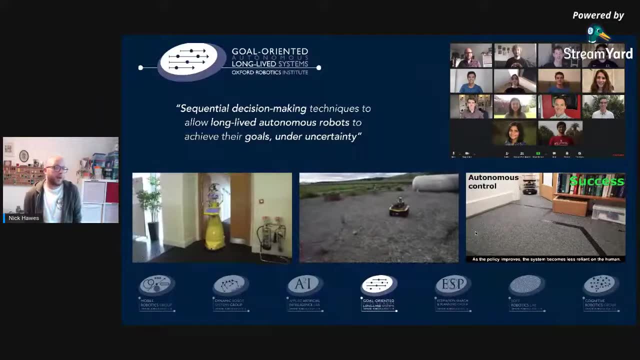 So we give a robot a goal. It comes up with a sequence of actions in order to move it, to change the world, to navigate around, to interact with things, in order to achieve that goal, And that's a field we call typically in the AI community. 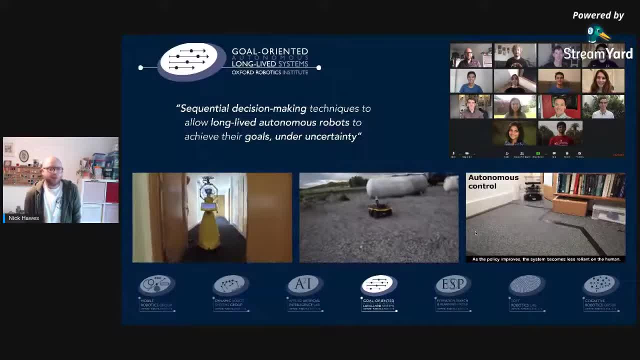 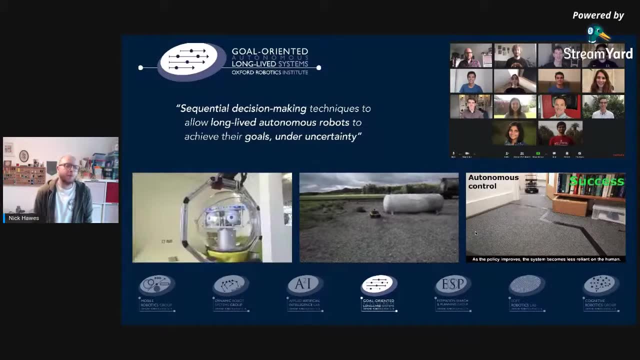 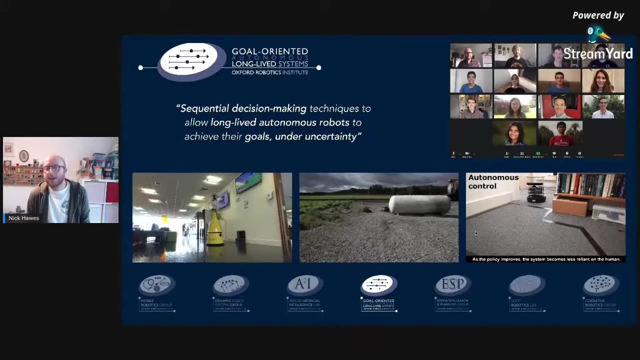 sequential decision making, And so my group research is a variety of algorithms, methods for sequential decision making for robots, So you can do a sequential decision making for kind of voice assistance. You can do sequential decision making for other kinds of computer programs. But I'm particularly interested 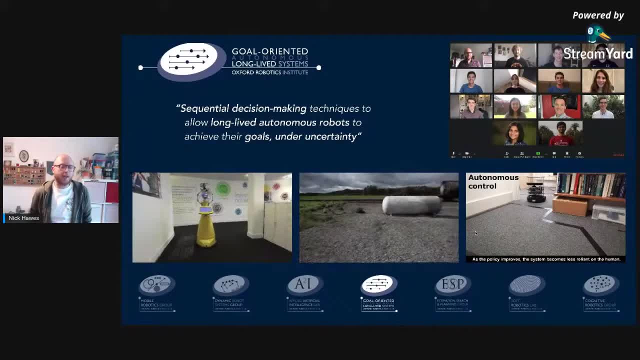 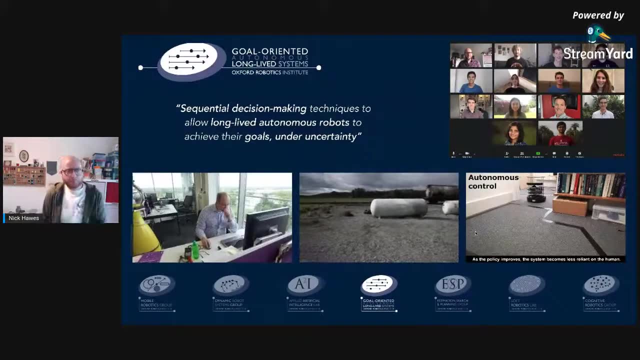 in doing this for robots, And I'll explain why in a little bit, And on here you can see a couple of videos of robots that we've worked with over the years and they'll reoccur And, of course, I put a link. 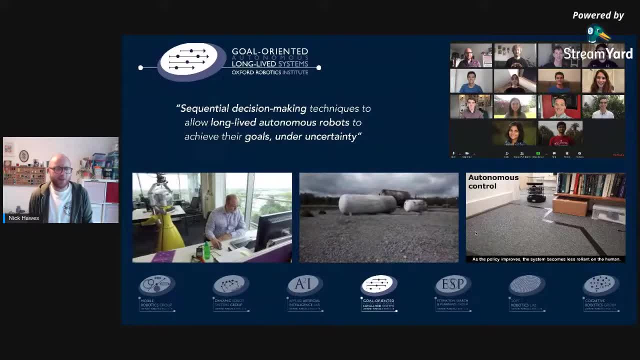 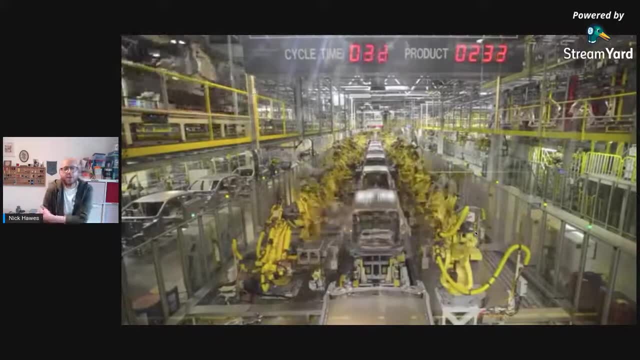 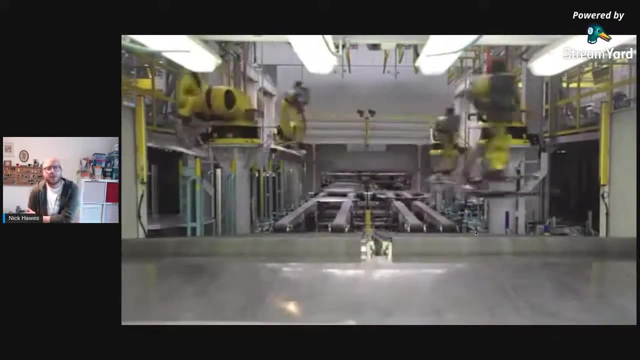 in the top corner is a picture of my fantastic group and all the lovely individuals in that. So I want to start by, I guess, frame, trying to frame the talk around- what is interesting and what is challenging in robotics. So if you think, 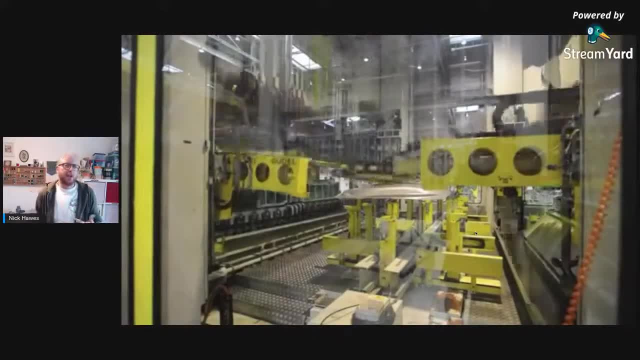 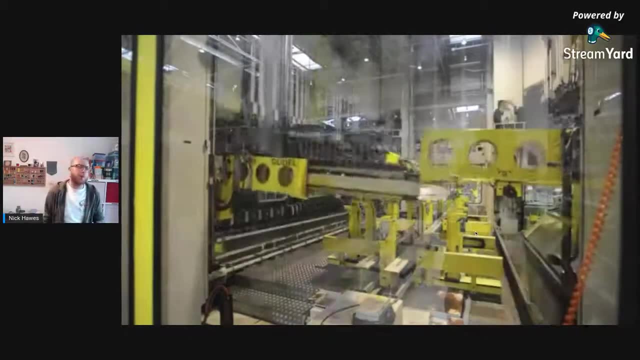 you know, often, certainly 10 years ago, if someone said kind of robots operating for businesses or companies using robots, I think everyone's mind would have jumped to manufacturing, where we had a huge robotics revolution from sort of the 70s, 80s onwards. 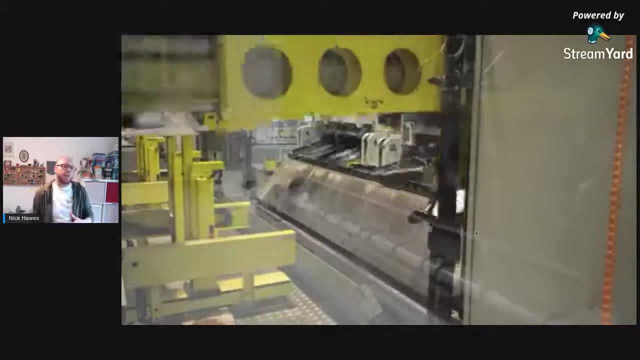 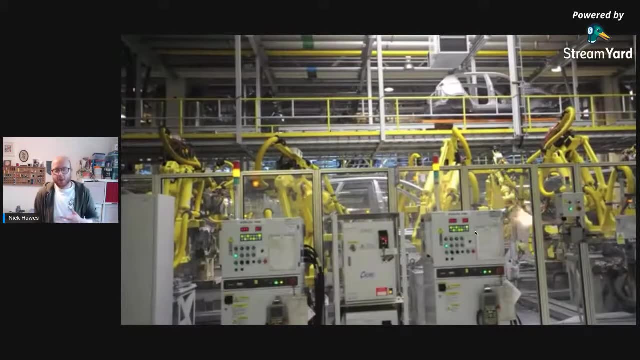 And these robots are incredibly impressive pieces of engineering, But in terms of artificial intelligence, in terms of autonomy, they're very limited, very restricted. So robots in a manufacturing setting are simply machines that repeat a fixed script with very, very high precision. 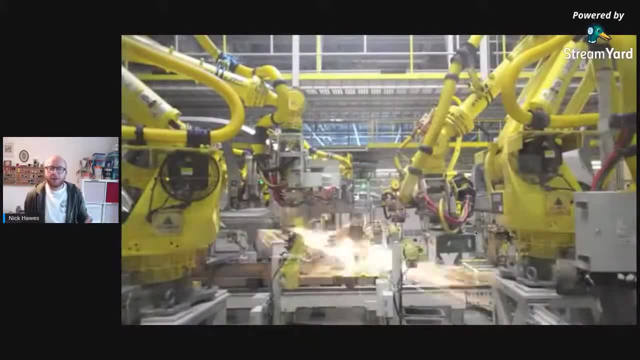 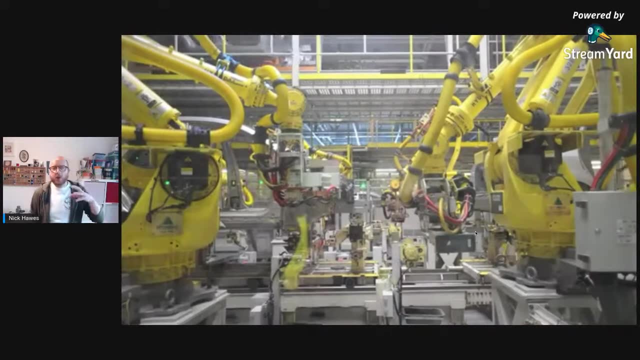 potentially very, very high speeds. And the reason they can just repeat this fixed script, this fixed sequence of actions, is because all the you know, you know all the dynamics, all the things that can change the world are kept out of these settings. 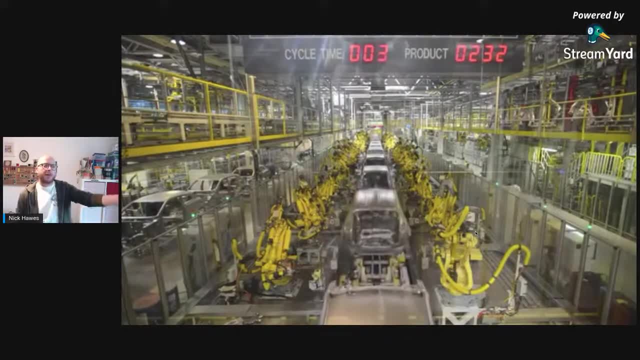 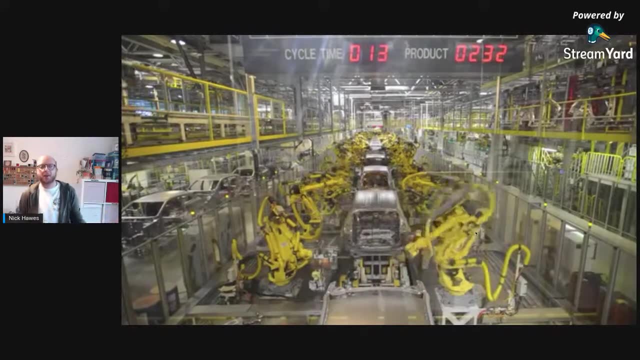 So in this, you know, we often think of humans being kept out of these factories to protect them from being squished by the big machines. In reality, the reason humans are kept away from production lines is because they interfere with the processes and stop the work. 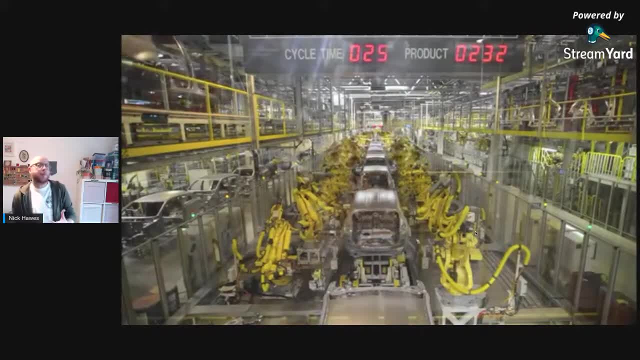 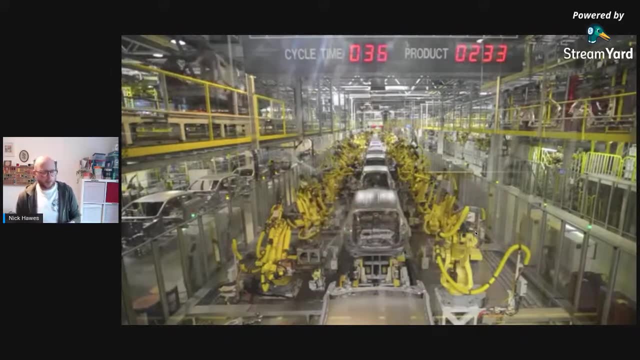 the robot's world being entirely predictable, And that's what we typically need to automate something: this entire predictability, And then we can automate a task such as manufacturing car and manufacturing industrial robots. So this is kind of maybe the history of robotics or part of history. 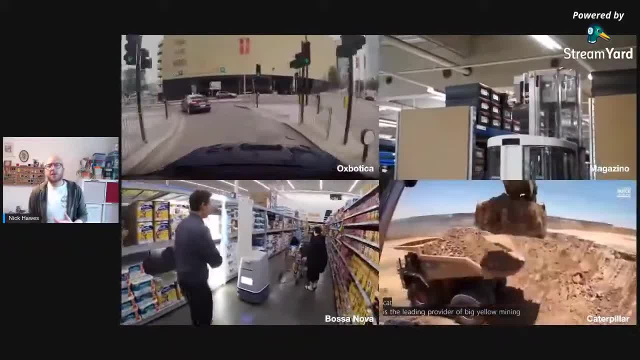 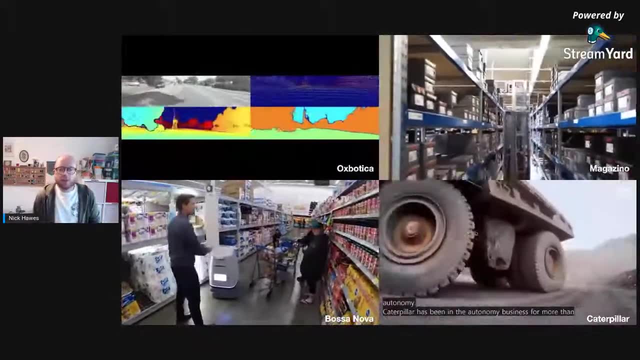 of robotics. I think what's interesting now is to think about where we want to go with autonomous robots and autonomous systems in the well, in the kind of near term and in the future. So, whereas you know, 10 years ago, 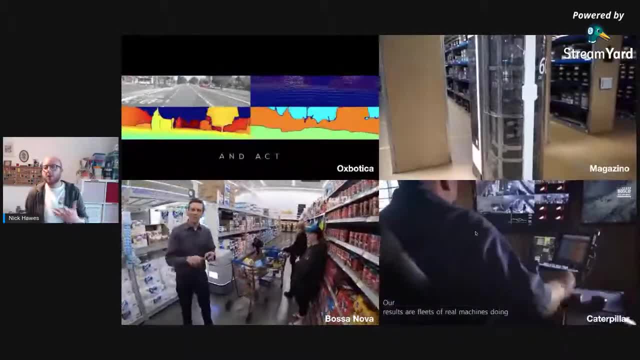 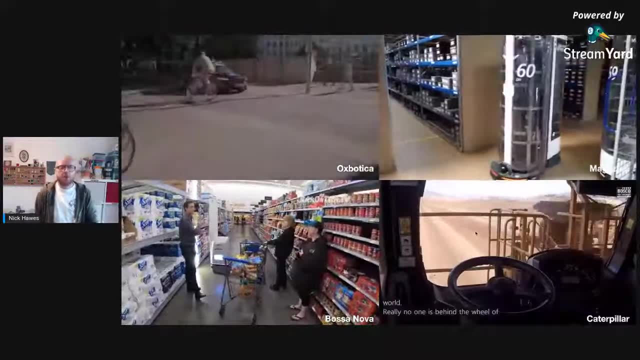 I might have said robots and people that thought manufacturing. Now we have a, you know, autonomous robots in a wide range of shapes and sizes and applications, So from autonomous cars, vehicles, robots in supermarkets that you can see in the bottom left here. 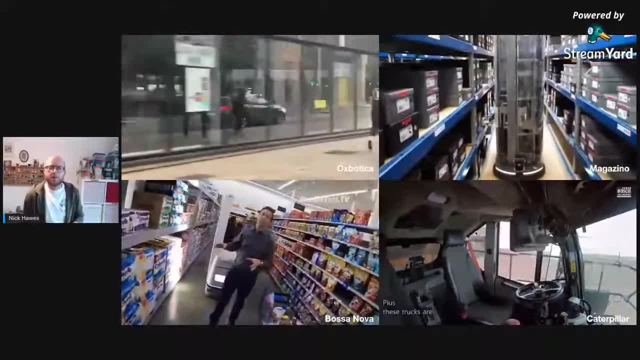 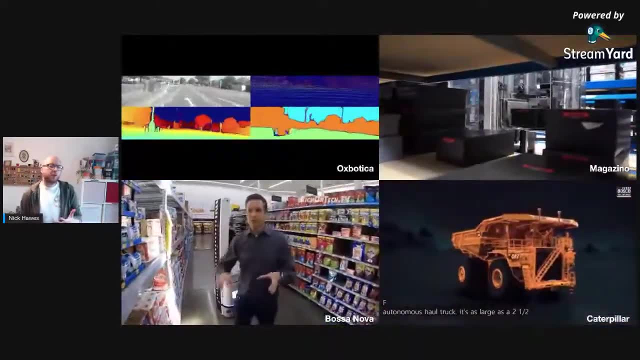 with a robot doing stock. take robots working in warehouses and shoe stores, And all these robots are autonomous, And they're autonomous, And what we mean by autonomous is that they can control their own behavior in order to achieve a task. So autonomy generally means 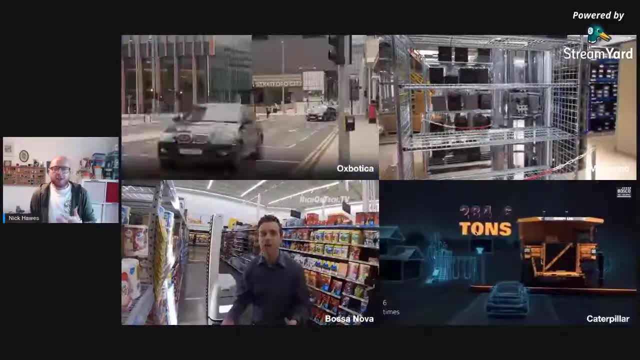 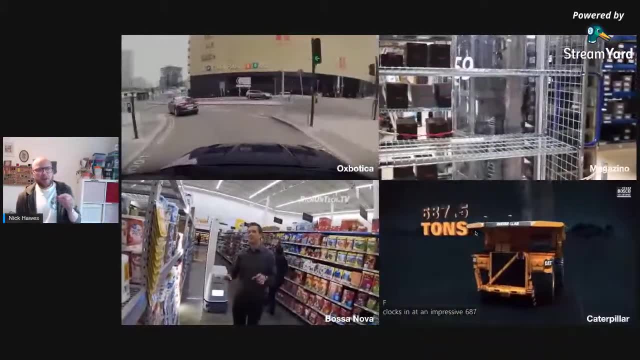 some ability to control your own destiny, And for a robot that destiny is very limited. But the thing that's interesting about autonomous robots is that they can control their own destiny. But the thing that's interesting here is the contrast to the factory setting. 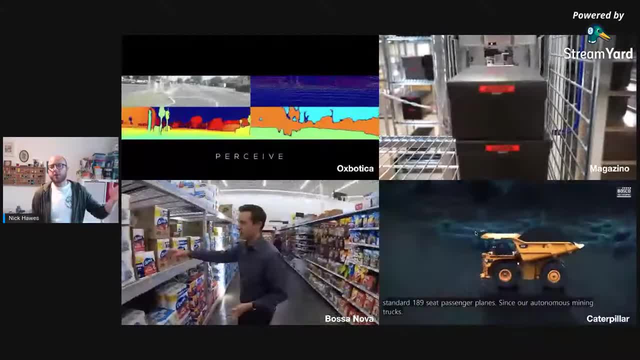 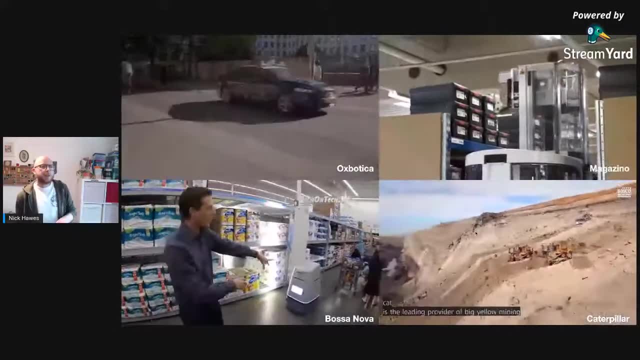 So in the factory setting, the world is entirely predictable, entirely fixed In all the examples I'm showing you here. I might just jump back to the slide and run again All the examples I'm showing here. the world is dynamic, There's variation. 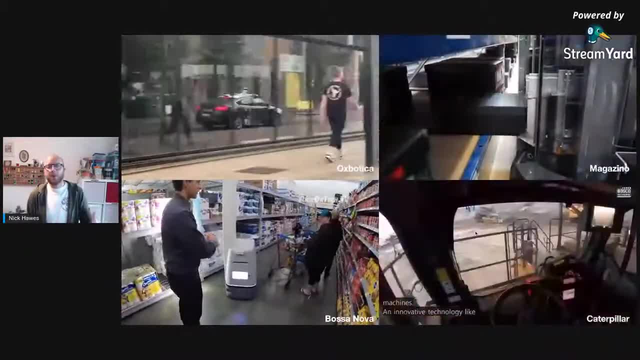 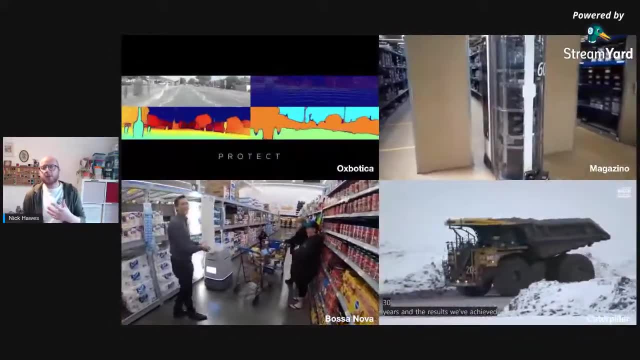 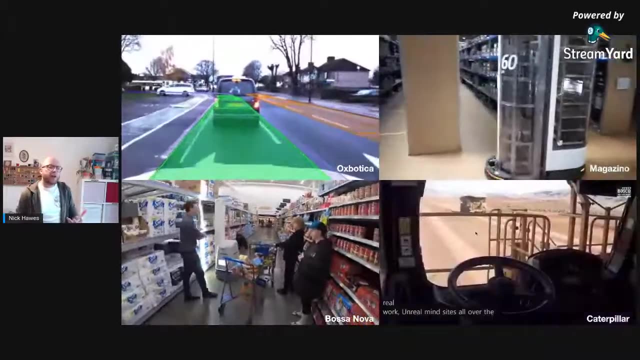 That variation may come from pedestrians, from people in a supermarket, from variations in the ground, from the way the boxes have been stacked on shelves. All of these are things that a robot does not know about in advance and can only know about by perceiving. 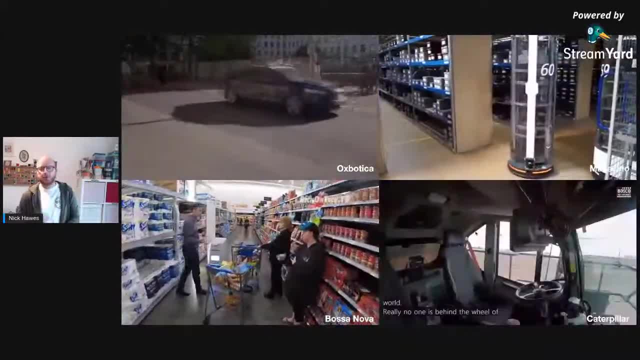 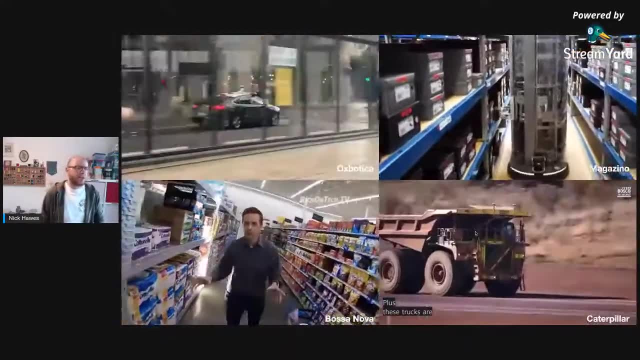 the environment with a collection of sensors. So this is where things become interesting for autonomous systems. They have to perceive their world using cameras and laser scanners and radar and sonar and all things like this, And they have to make decisions on how to act. 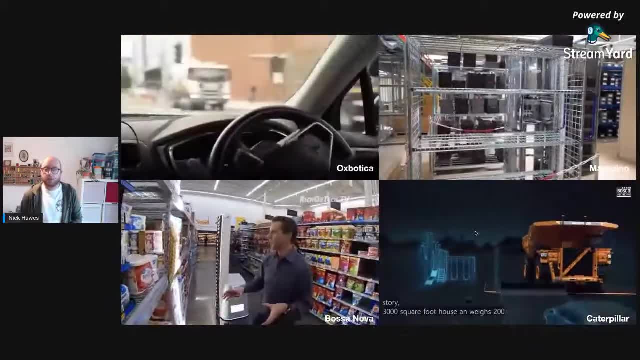 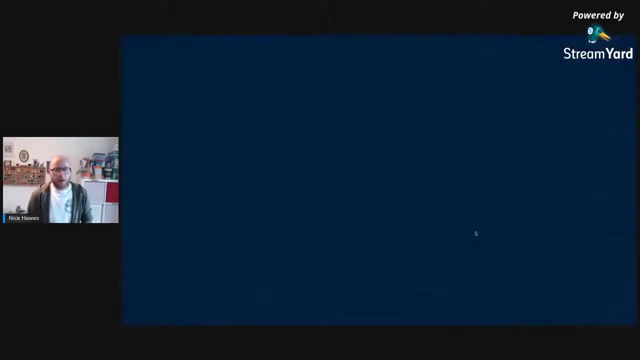 how to move, how to interact with the world, based on the results of those sensing processes. So autonomy is interesting to deal with the variation in the real world. So what does that mean? Well, an autonomous robot has limited sensors, It's only got. 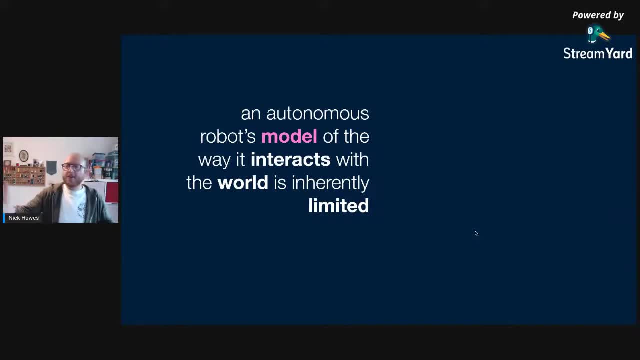 a range of a couple of meters to tens of meters for its sensors and it can't fully perceive the world at any time, any instant. And what that means is we have to write computer software and algorithms that sit inside the robot that models the way. 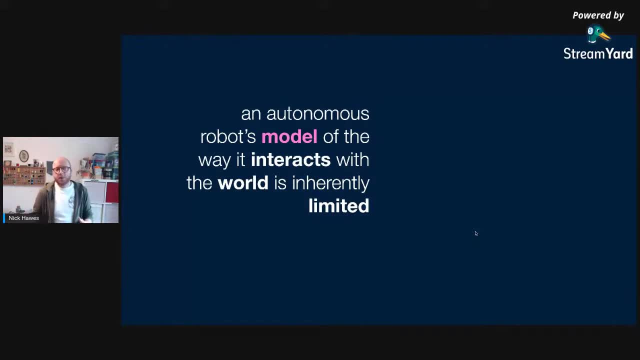 the robot will change the world in the future and just predict the dynamics of the world. So an autonomous robot, all autonomous robots, have some kind of model, and by model I mean a kind of computational artifact, a bit of software that sits inside the robot. 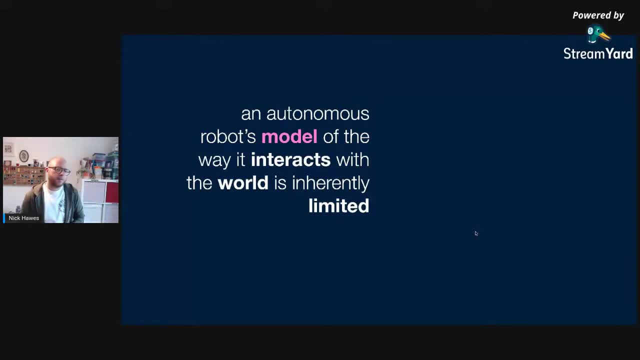 and the robot uses that to predict the way the world will change when it interacts with it. Now that model, for various reasons, is limited, it's restricted, it's not of importance to the world, because the world is stochastic. dynamic moves in three dimensions. 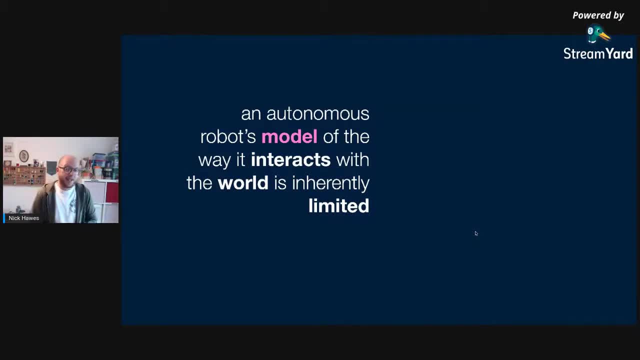 and is continuous and all these kind of things. A robot can't model that exactly in its head, in its software. So that means that model is limited. it can't accurately predict the way the whole world changes. And what that means is when we think. 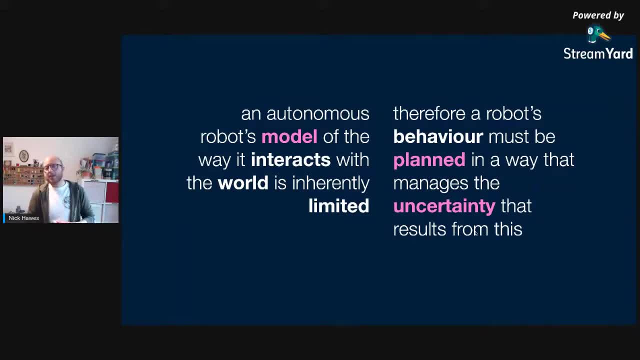 about how a robot should change its own behavior, should plan sequences of actions in order to change the way the world is. well, that behavior has to reflect the uncertainty that the robot has, And that's where this talk is motivated from A robot. 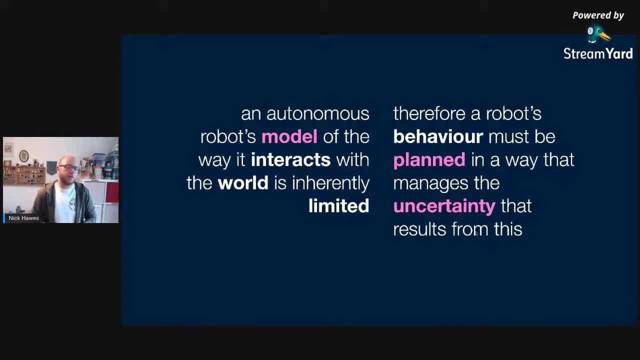 is inherently limited in its ability to perceive and predict its world, and that limitation means that the future of the world, when the robot acts in it, has some uncertainty. And what I want to talk about today is the methods we use to deal with that uncertainty and plan robot. 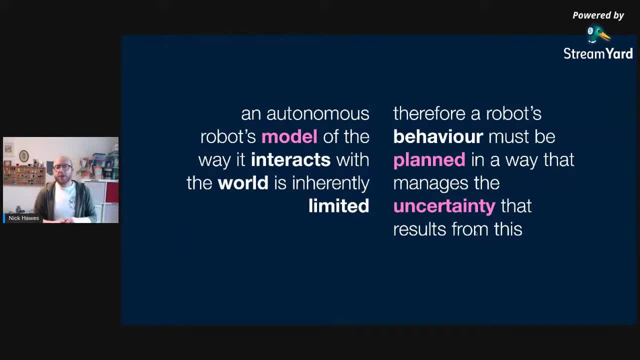 behaviors to reflect that uncertainty, And I'm going to talk about this from a perspective of long sequences of robot actions. Other people in robotics work on control, so how you would literally move the arm of a robot or steer a car for a meter. 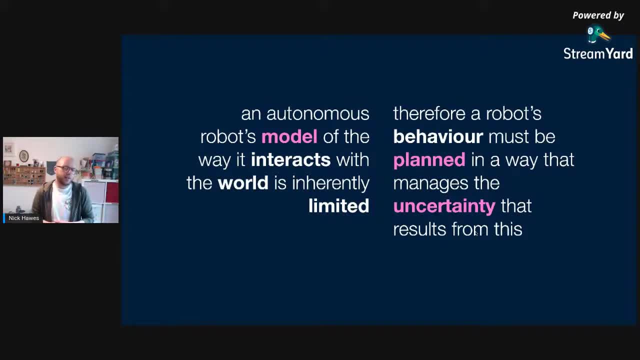 And that's one sense of action that requires you to manage uncertainty, But I'm interested in long sequences of actions that might take hours or days to complete, So I'm going to talk about the methods we use in AI and robotics to plan robot behavior. 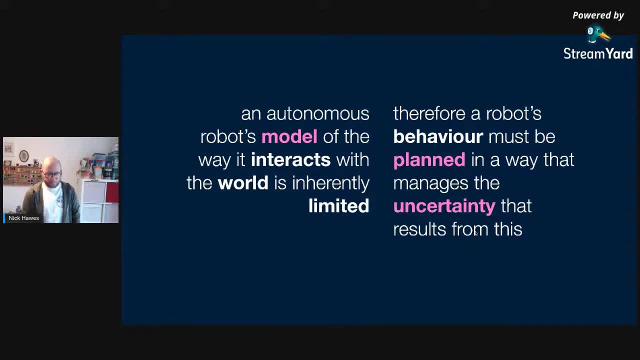 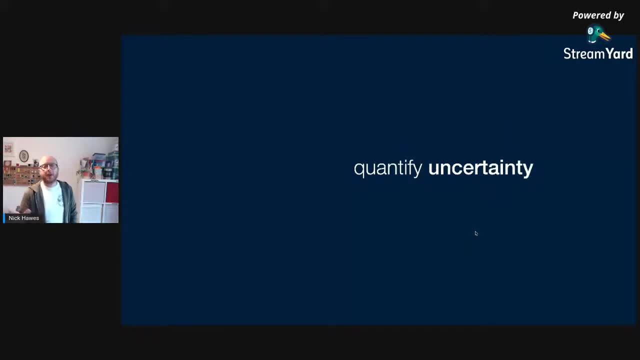 such that it can manage uncertainty. Okay, so how do we do that? Well, there's a kind of process that's very common to actually a huge amount of statistical modeling, maths, AI, robotics, And that starts with understanding where the uncertainty 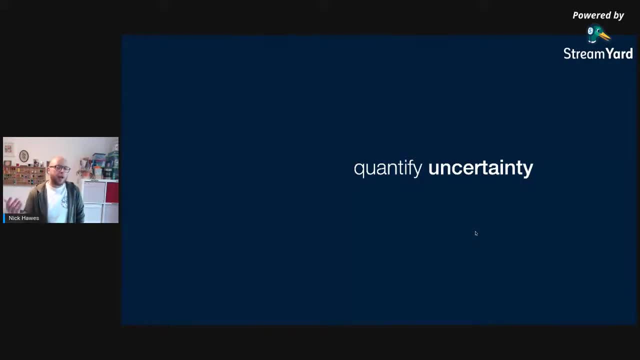 is in an AI process, in a robotic process, And we need to measure that and model it mathematically. So we're going to use probability to do that And a huge amount of robotics and AI is founded on probability theory And we're going 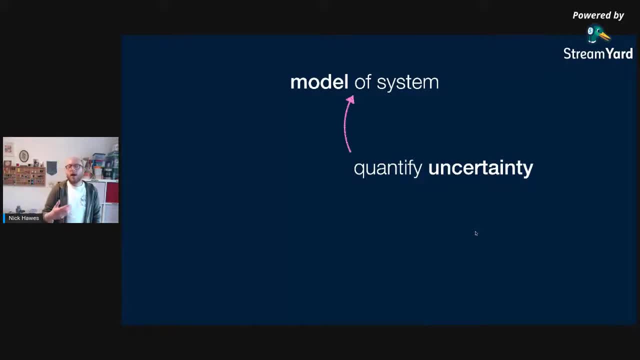 to factor that uncertainty into a model of our system. So, in particular, we're going to model the actions a robot is trying to achieve. Then we're going to write down what we call a formal specification, a specification of what the robot is trying. 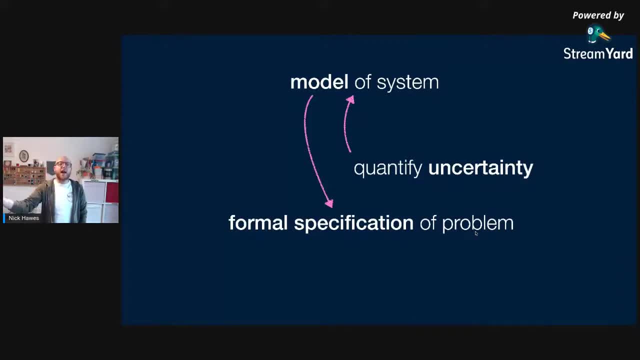 to achieve. So, if the robot is trying to move from A to B, a formal specification might be: the robot is at location B, or the robot is at location B at time, at 3 o'clock, for example. So we'll write down some kind. 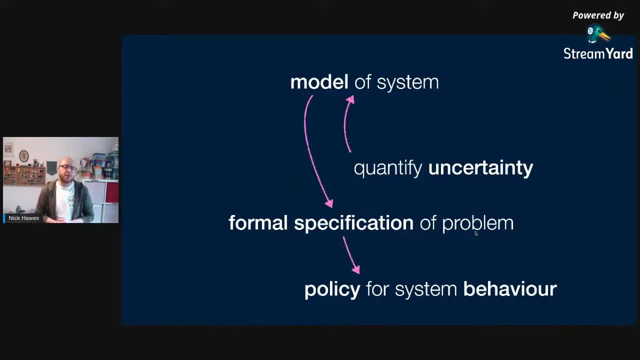 of a formal specification And we're going to take that collection of a model, a formal specification, and we're going to solve it for what we call a policy. So a policy is simply kind of a set of instructions that the robot can follow. 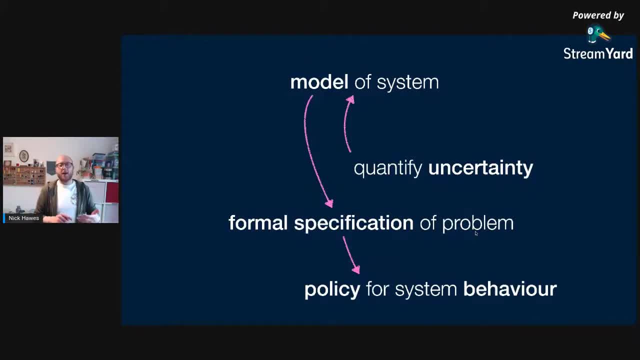 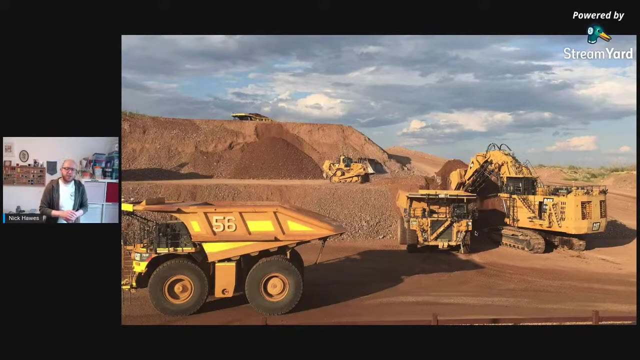 when acting in the world. You can think of it as a plan. the robot follows step by step, or even something like a lookup table, where the robot is not going to be able to see the robot and the robot is not going to see the robot. 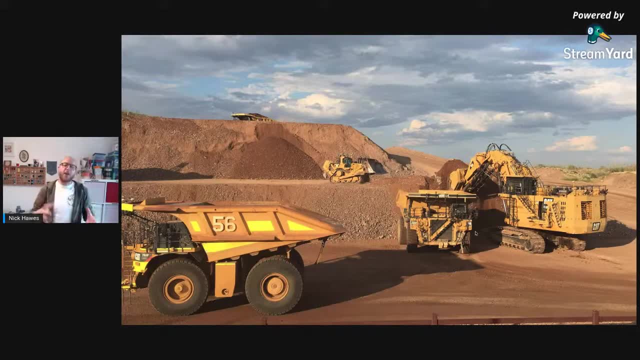 So I'm going to start probably the chunk of the majority of this talk trying to motivate the problem and give you an example of the kind of way we think about it And after some work we've done with these particular robots. but we have thought about 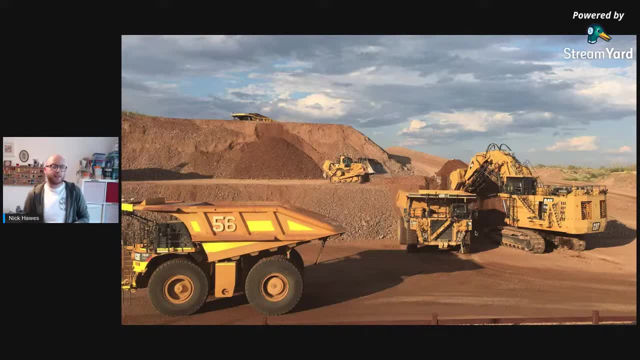 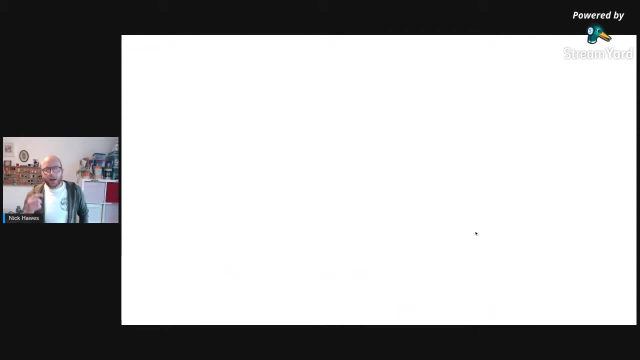 this problem from a planning perspective which is moving all around in a mining setting. So one of the big consumers of autonomy, of autonomous vehicles, is the mining industry, because it's incredibly hazardous, dangerous and they've also got a lot of money so they can afford to. 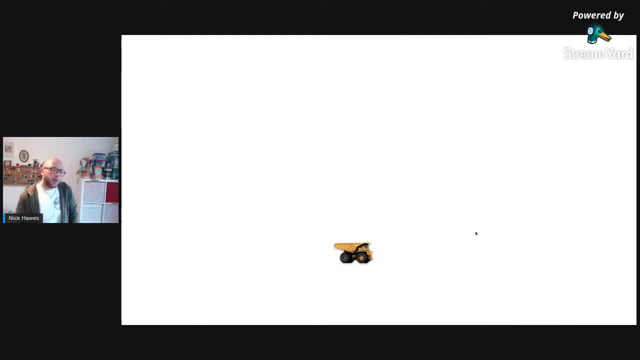 spend a lot of money on the mining industry. So what we're going to do is we're going to try to optimize the amount of ore that you can move with a single truck, And the problem starts with what we're going to call the primary. 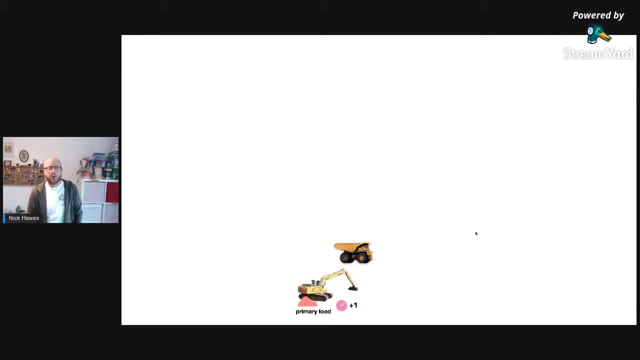 loader. So the primary loader is going to use our ore into whatever truck is there and we're going to actually model the world and have some time. So every time the truck gets loaded that's going to take one unit of time and that's a fairly 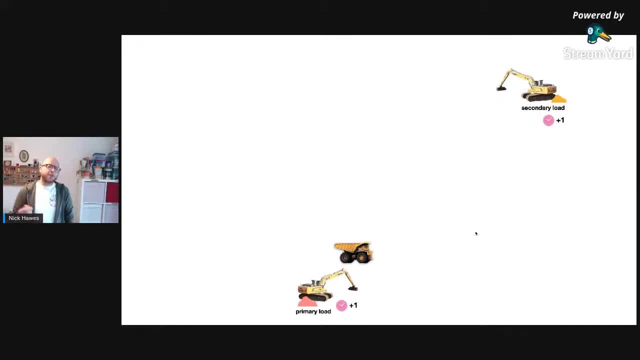 standard way to think about these problems. We might divide the world up into extra ore and again that takes some time and maybe this is a manual process. So if the robot goes there it can get a secondary load, but it doesn't have to go there. 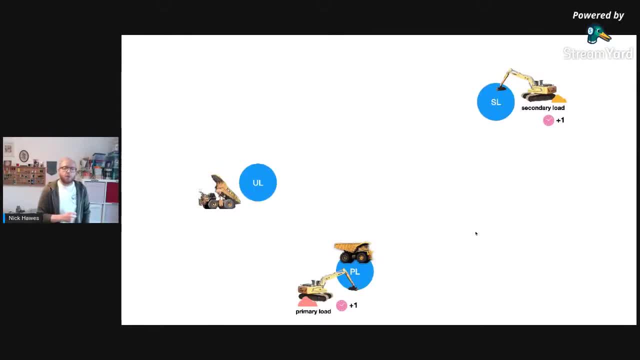 And then we're going to have a location where the robot can unload. So it's collected, it's loads at various locations And because we're a business in this example, we're going to get some money For every load we unload. we get some. 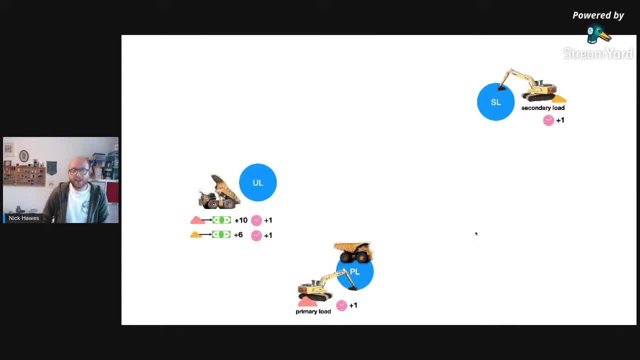 reward is what we call it in an AI planning process. We can think of this as linked to utility, think about rational decision making, But we'll refer to this as a reward And we have some kind of map of the world. So this map- 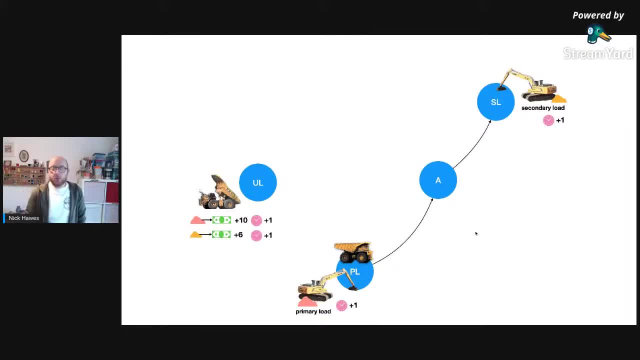 represents places the robot can drive and the connections between these places represent routes the robot can safely navigate. So I showed you some examples when the videos are running of robots moving around in the real world and this just kind of demonstrates this is a thing they can do. 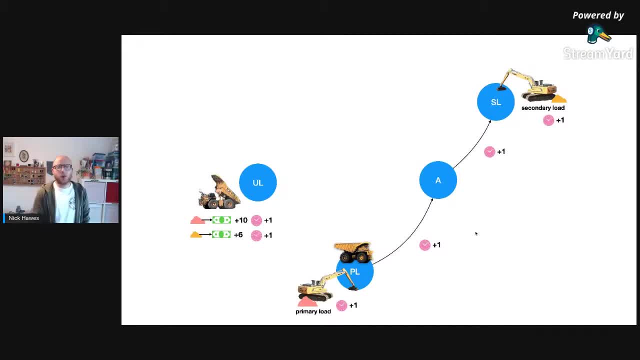 So in this case we're going to make life easy and say everything takes one unit, But now we're going to introduce the planning problem, the decision-making problem. So the robot has a map that allows it to navigate back to the unloading spot and it 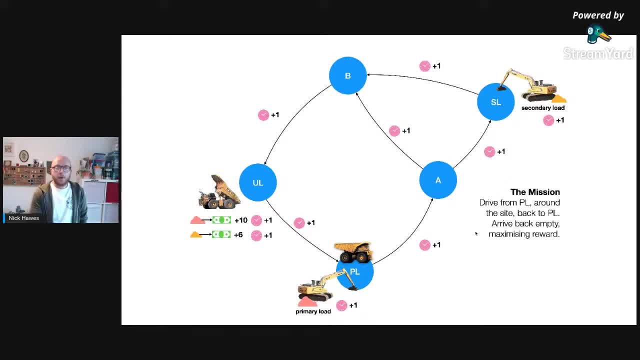 can make a choice. Does it visit the secondary loader or not? That's going to be the answer in a formal language. The robot's goal is to get back to the starting point. So go around this, get back to the primary loader and to be. 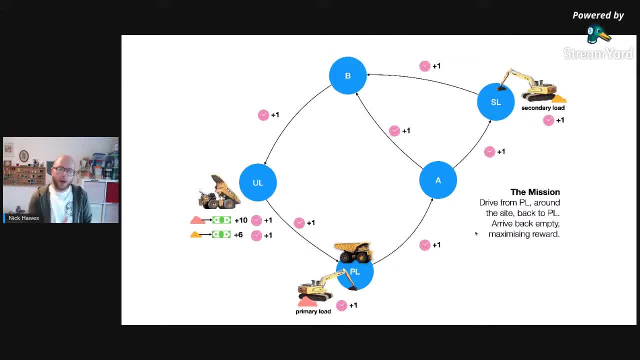 empty. So it has to unload, which in this case is the only option it has. So it has to stop at the unloader to unload. It can't go back to the primary load full of all, And our goal is to maximise or 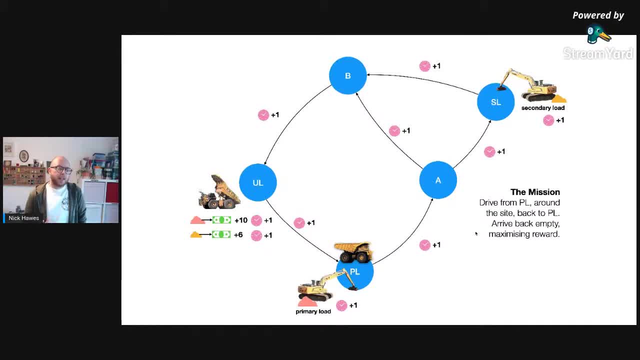 minimise is the amount of reward we get from a mission. So we can think about the reward we get as the number of banknotes we get. So we might be able to get ten, we might be able to get six, We could also try to. 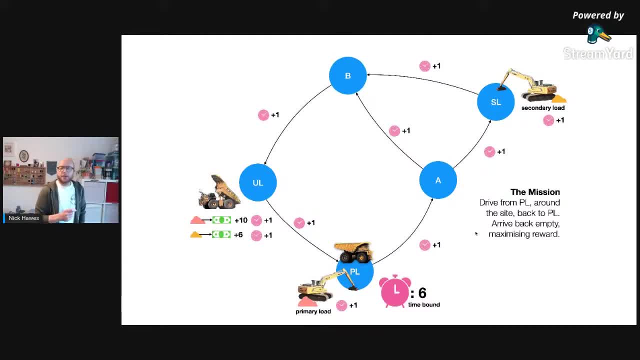 get none if we make some mistake and forget to unload or something. So this is what we can do. So we have a deadline to get back by. You can think about this deadline as a configuration parameter on the first loader. We can say that that 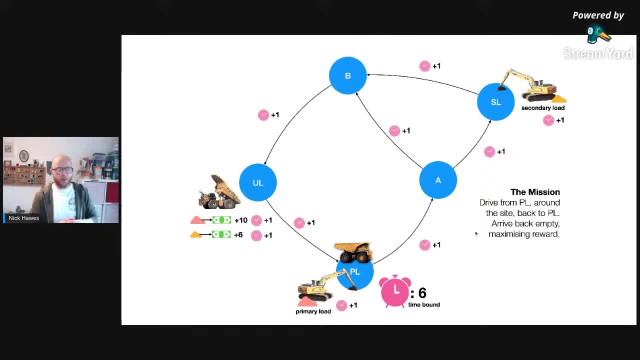 loader is a machine that every six time steps spews out rock in front of it. It's a lot cheaper to build a machine that can do that than one that has to do six time steps. So this is a very kind of typical logistics planning. 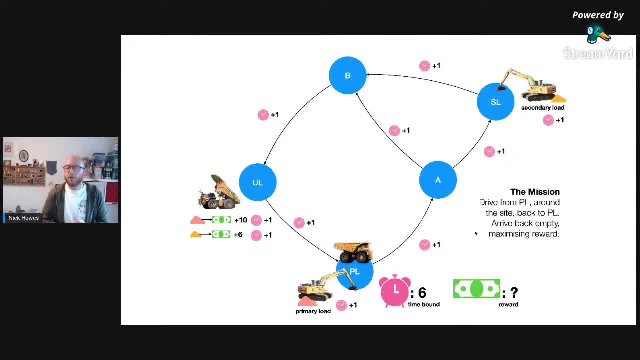 problem And the question we might want to ask ourselves is: how much reward can we get from one mission of the robot? And the answer is: if our time band is six, then we can get a reward of ten. I will just give you the. 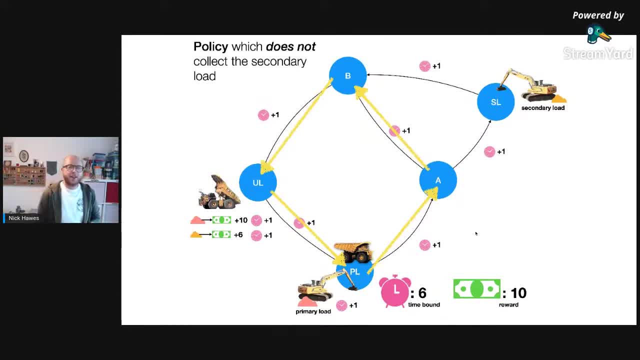 answer myself, So we can get ten reward for executing this policy. So I said policy was the thing we're going to create and that's what these yellow arrows represent. So the policy of the robot is simply to follow the yellow arrows and of. 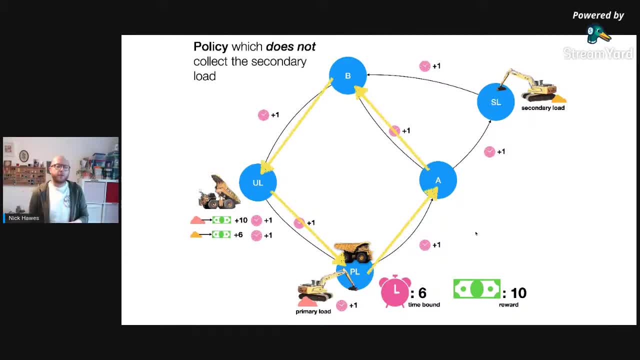 course, unload and load where they're required. So if our time band is six, we would have an algorithm that would produce this policy and that would say that policy gives you a reward of ten If we had a time band of nine. 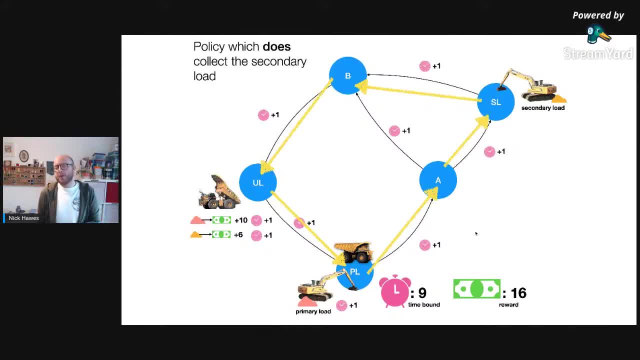 then with this problem, we could always go and get the secondary load. So if we run this process, we could get the secondary load. So this is where things start to get interesting, because we could introduce uncertainty, The task of driving around in a 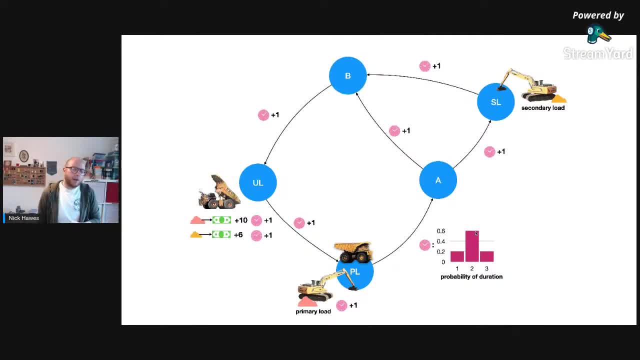 mine like the ones we pictured previously is actually fairly uncertain because of the gravel underneath of traffic. if another person is driving around in a mine like this, then we would have a reward of ten. So we would have a reward of ten, So we. 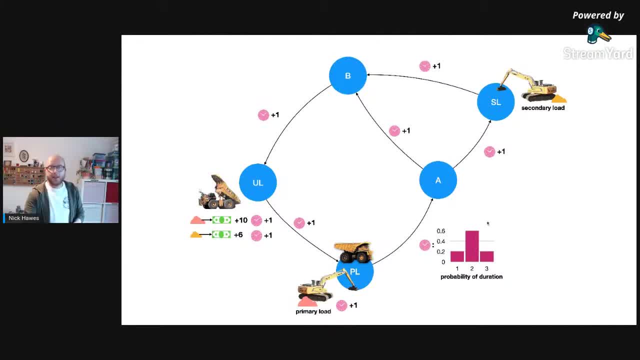 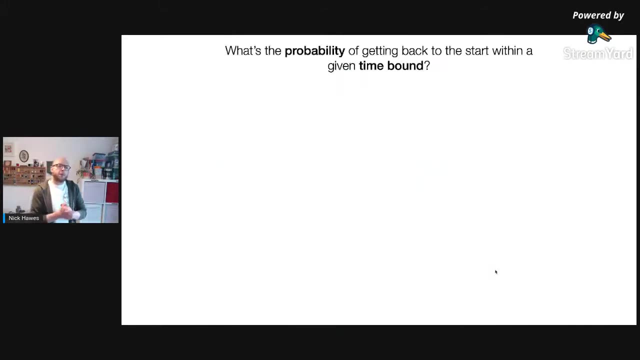 would have a reward of ten. So we would have a reward of ten, And once we start adding uncertainty, the decision about what the robot should do gets a little bit more complicated. So typically we want to start thinking about the probability of meeting the mission. 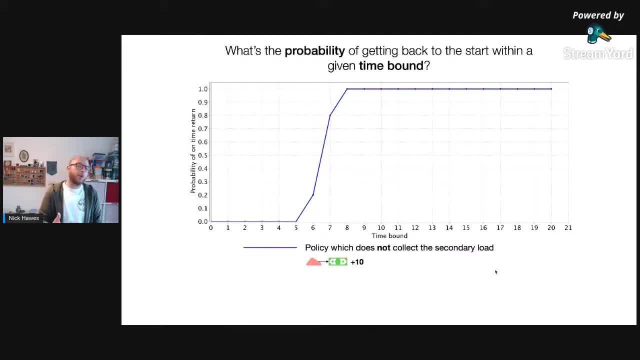 specification. So my group works on algorithms that solve these kinds of problems, So I'm going to show you the probability of the robot getting back within that time bound. So this plot shows as the time bound gets longer across the x-axis on the 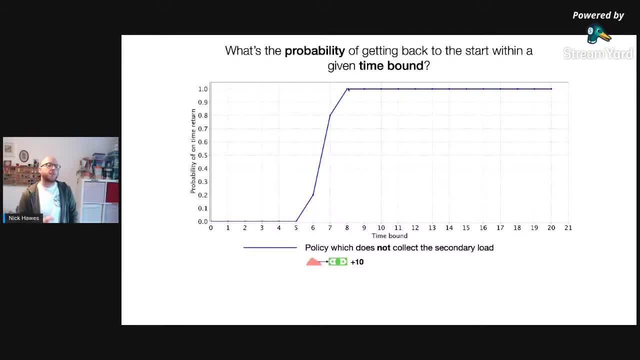 y-axis we can see the probability of the robot getting back within the time bound. So this time bound makes the robot 100% safe or the problem 100% safe, And I can also plot the policy which gets the secondary load. So this: 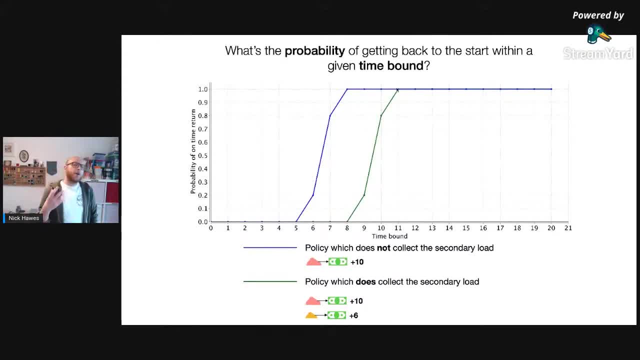 is a different type of robot behaviour. It goes the long way and we can see that if the time bound is below 8, then there's a chance we might not reach the goal entirely, And if the time bound is 11 or up. 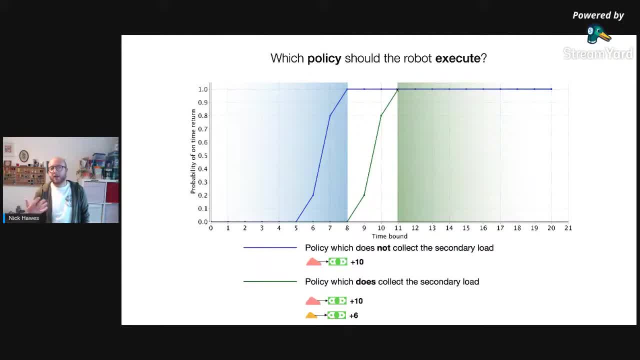 then we should definitely execute the policy that visits the robot. So what we do if the time bound is not somewhere in this region that's highlighted here, if the time bound is 9 or 10, what can our robot do? How can we create? 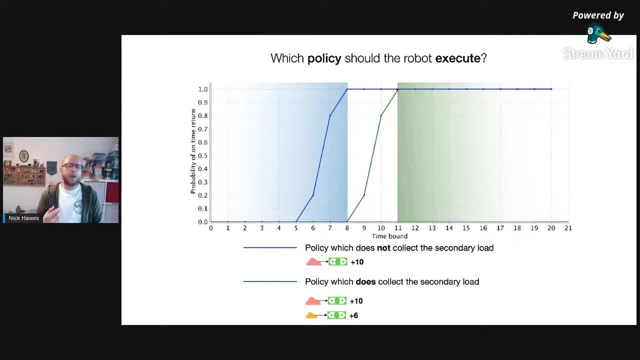 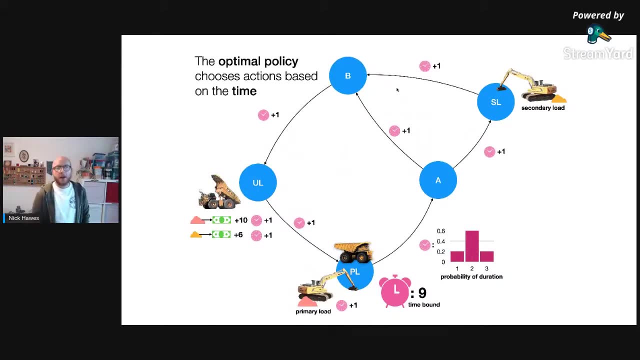 a policy that allows it to gather reward. We could just choose a time bound of 9, and that's what we really want in an autonomous robot situation: the policy to respond online. So the optimal policy, which is the best policy, makes a. 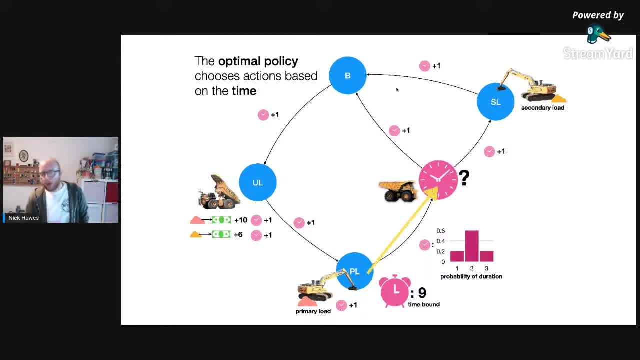 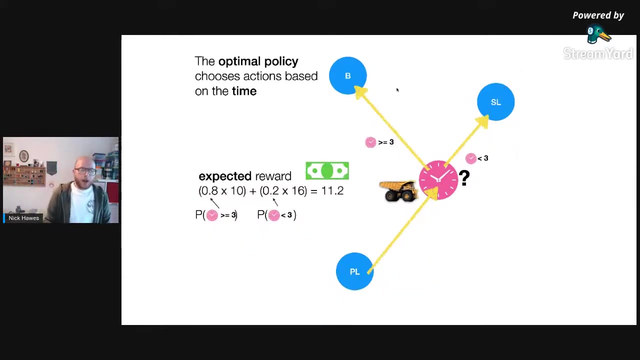 choice based on time. So say we've got a time bound of 9, if the duration is only 1 for that previous action, then we can go and get the secondary load. If the duration is longer, then make a different choice and 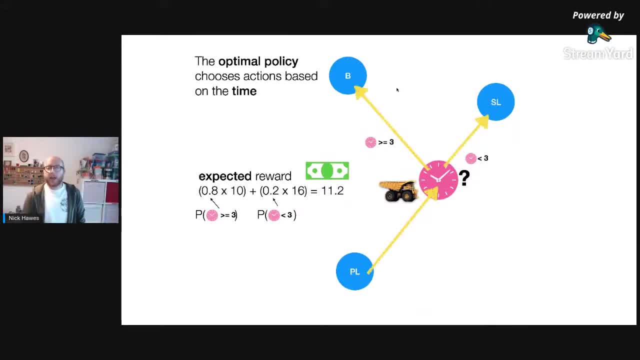 take the shorter route and then unload And, given that policy, we can talk rather about the reward we get in a particular outcome of a particular policy operating in a world or a model, And that expected reward is just the probability of an outcome multiplied by 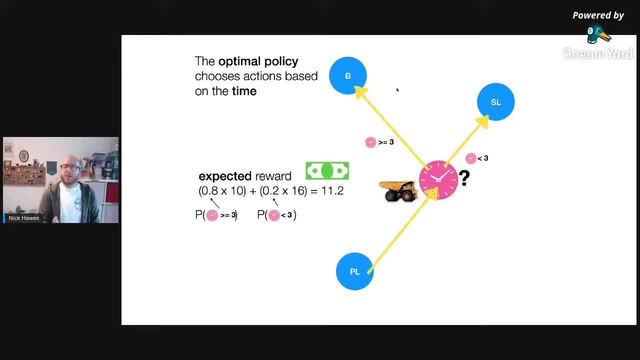 the reward it gets, the utility it gets, And we sum this for all the different outcomes. So there's one world in which we can get- I'm not sure these actually match up to the graph. We can only execute the policy that gets 10. 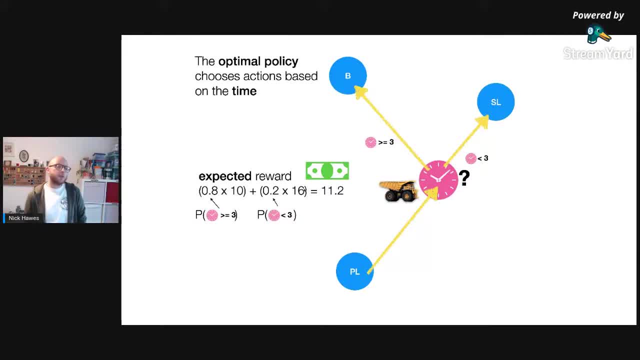 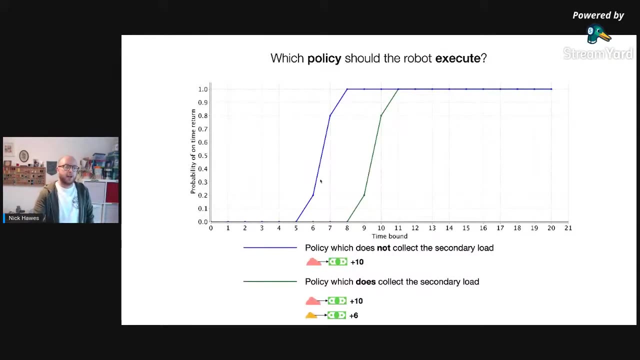 reward and 20% of the time we can execute the policy, that gets the 16 reward and we sum these together and we get an expected reward of 11.2.. And that's great because that means it's better than just being conservative and executing. 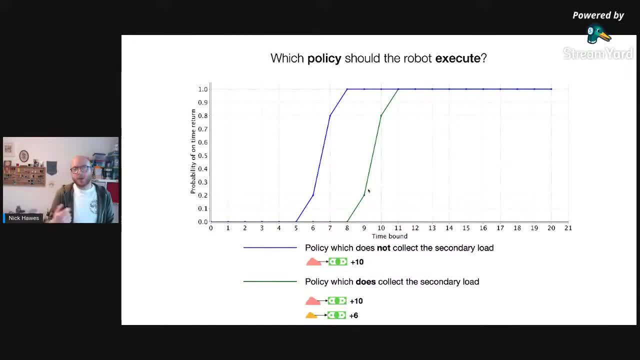 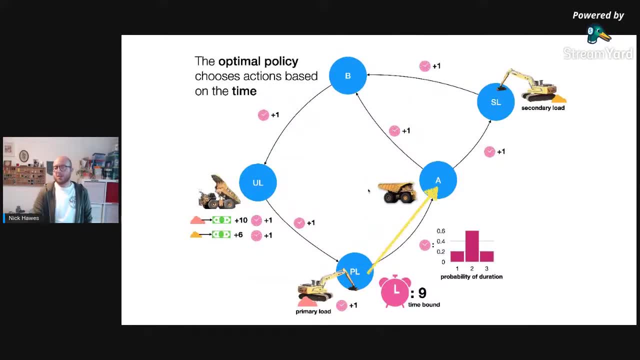 if I jump back, it's better than executing the policy that completely fails and messes up the system. So by having a policy that's adaptive or responsive to the changes in the environment, we're able to actually perform better than in either one of those. 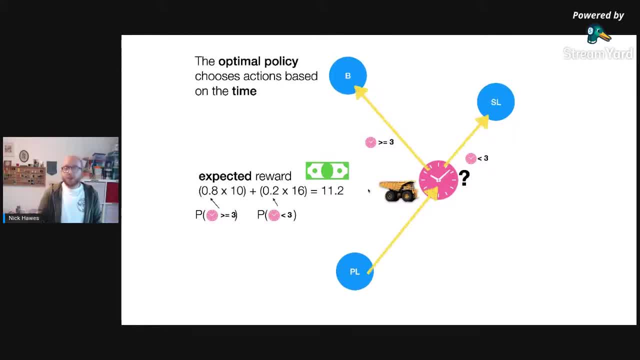 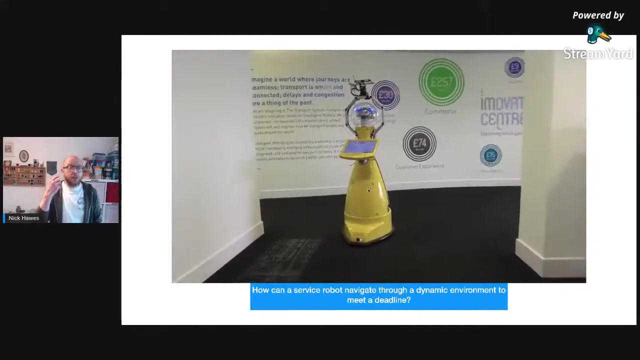 two cases, And that's exactly the way we think about planning for autonomous systems. We build these models, we model these models and we look at the probability of the robot having different outcomes when it acts. So we use that in a bunch of different. 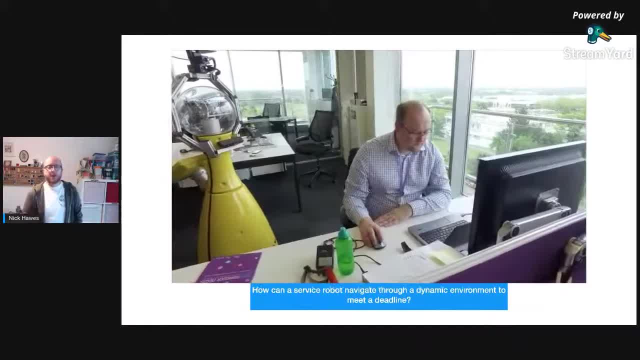 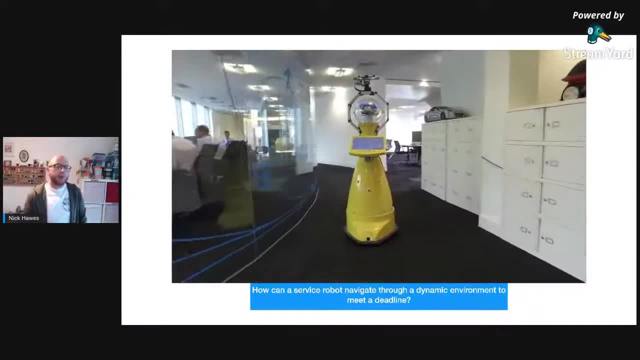 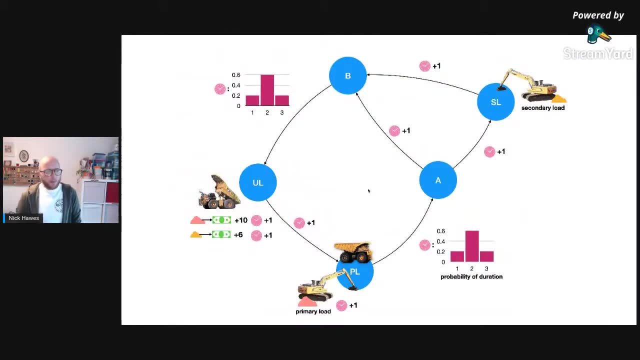 examples. One great example I'll talk about later on is using these models of time to plan how a robot can arrive in these environments, And we'll come back to that in a little bit. The other thing we can think of is what happens if 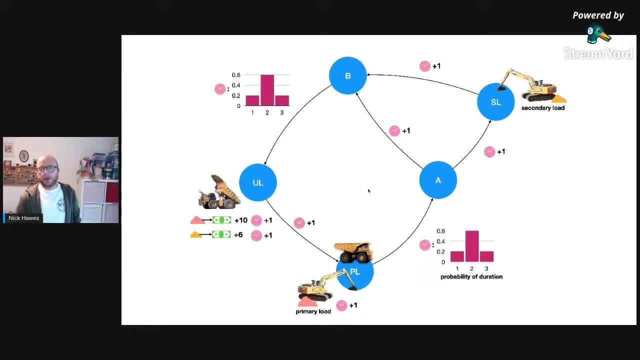 the world gets even more unforgiving. So in our previous example we had an uncertain transition at the start. The robot can make a choice after it. If we have an uncertain transition, the robot has to follow a fixed policy, And this means we. 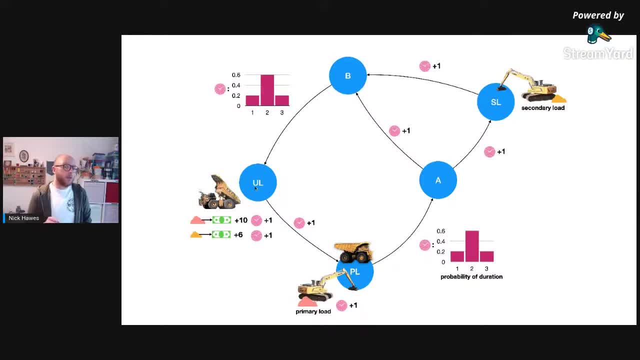 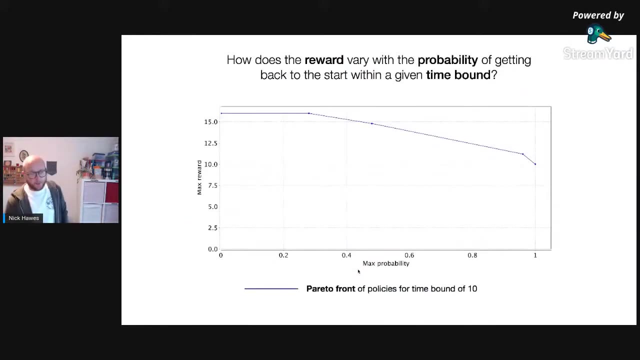 can no longer guarantee that the robot satisfies any mission specification, Because now in some worlds we will fail to reach our goal with almost any time bank. So we can think about the probability of the robot getting home safely, the robot getting home empty, against the 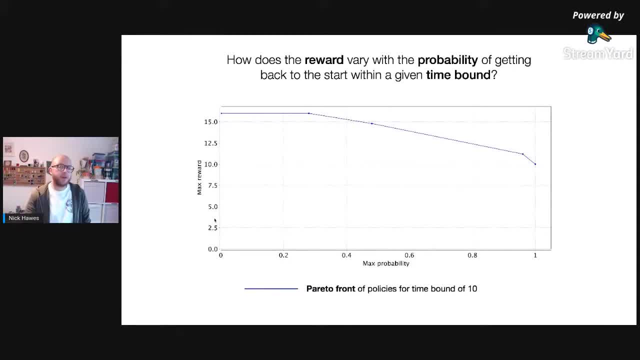 kind of reward it can gather from a different behaviour. And then the dots, the points on this graph, actually respond to different behaviour policies the robot can execute. So this is an example of what we can do, And I think most, I would argue. 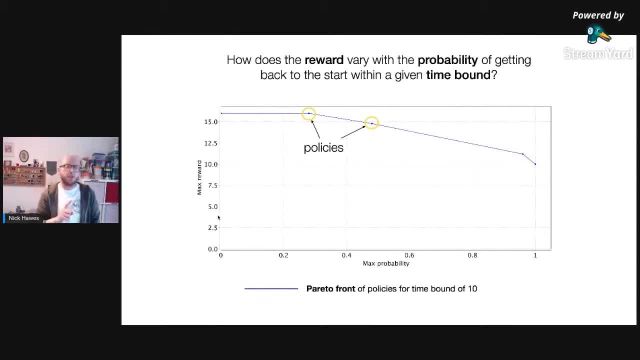 most interesting robotics problems have multiple objectives. In this case we have two objectives. One, we want to maximise reward. Two, we want to maximise the probability of getting the robot home safely, of unloading the robot back in, and we want to 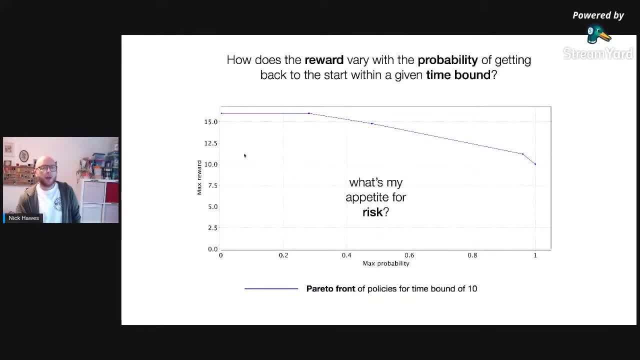 maximise reward. So we start off with coal. how do we choose the way to put it in the model Or how do we get this into the? Okay, I'm going to jump to that example in a minute So to kind of close off. that was. 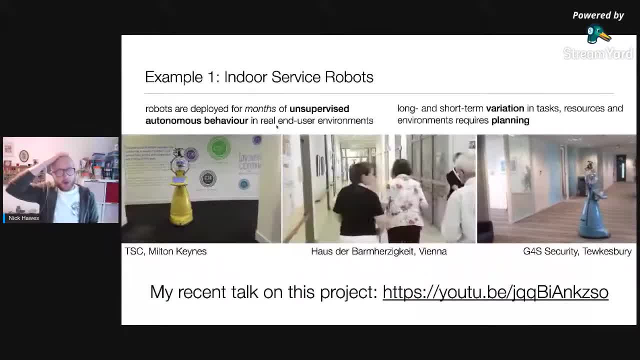 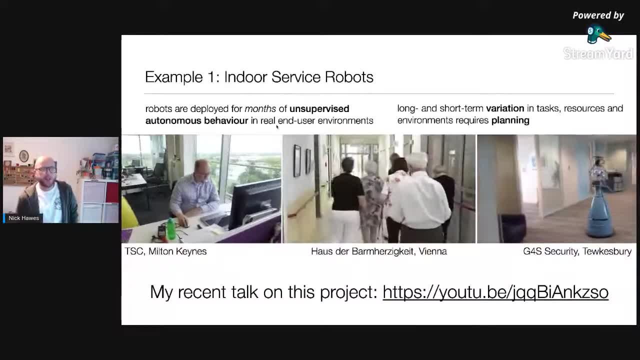 all very abstract. I want to talk about two specific projects we've been working on and just give you a rough idea of how some of those ideas fit in. So this is a project called the strands project. It was a European project. I ran from 2013 to 2017, so it's a 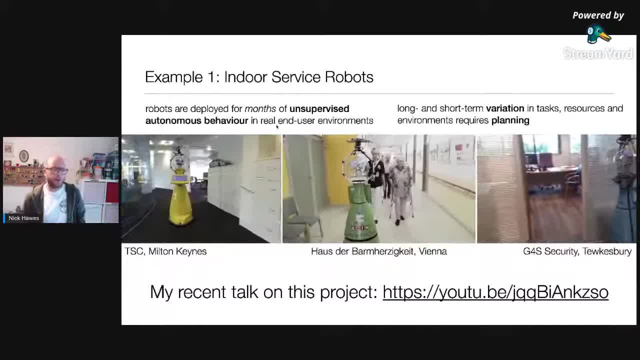 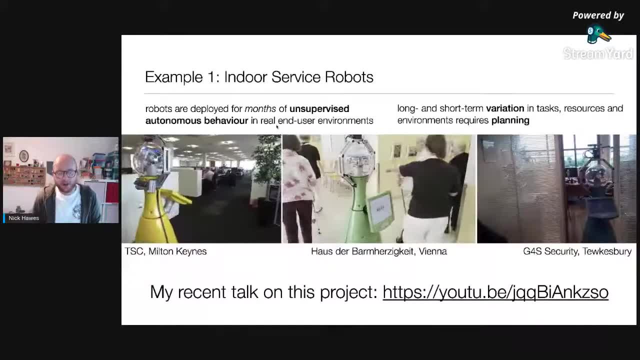 bit old now, but it was very exciting at the time. We put service robots such as the ones you see here into a range of care and kind of office environments. And if you want to see me give a slightly more academic talk on this project, then there's a link there. 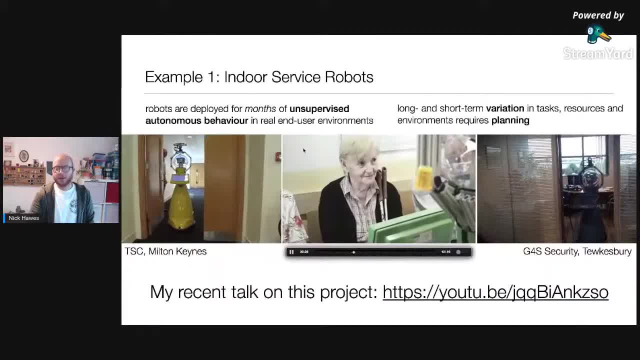 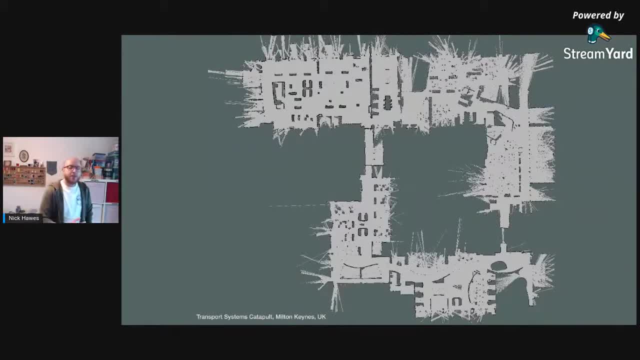 on the slides. You're not going to click it, but you can copy it down if you go back and watch this. And these robots were trying to be at particular locations by particular times, so we had to model the uncertainty in the duration of their action in the environment. 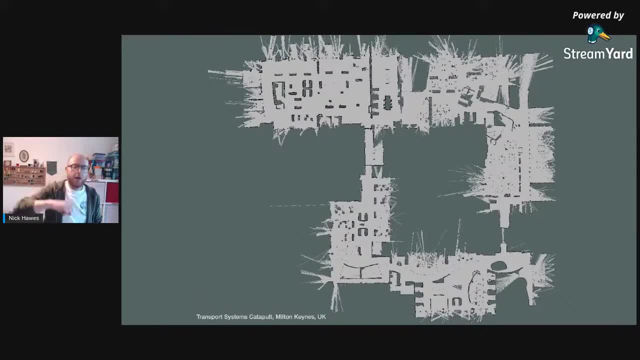 So a robot's world would look something like this. This is a top-down view of the two-dimensional map the robot operates in And we divide exactly as I showed you in that kind of toy example. we divide the world up into these locations the robot can visit, And each of 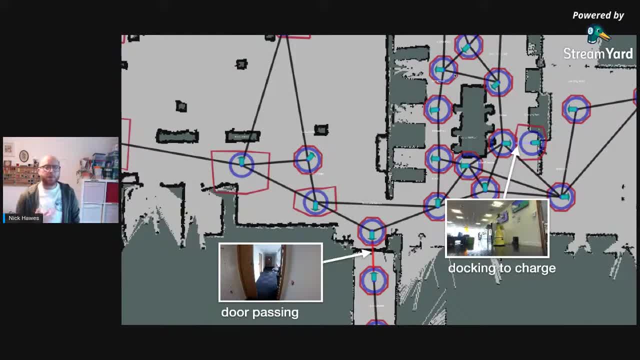 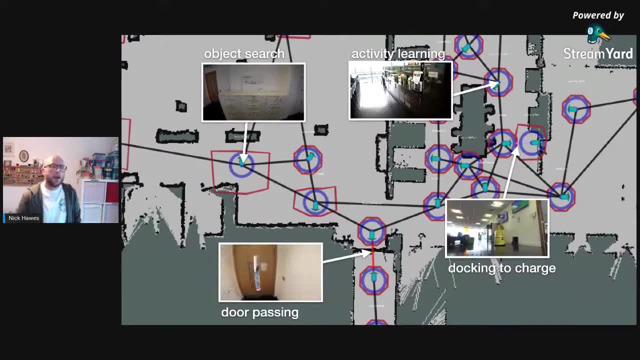 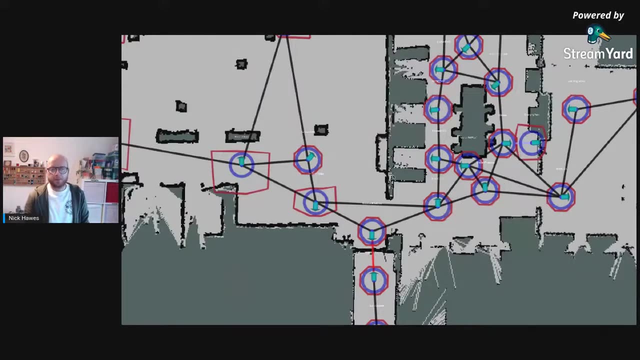 the edges or the lines between these locations represent particular actions the robot can perform, such as going through a doorway or docking onto a charging station to recharge its battery, And we also annotate these locations with things the robot can do, such as looking for objects or learning things about people. 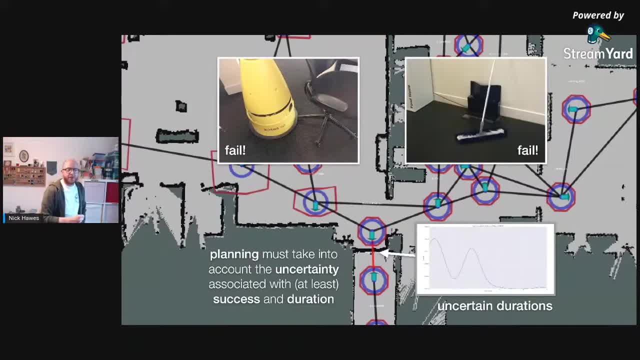 Now there's a huge amount of uncertainty for robots in these environments. The uncertainty comes from the fact that humans can move around, which causes all sorts of problems. Also, the robots can get stuck on features of the environment. They can get stuck on chairs. 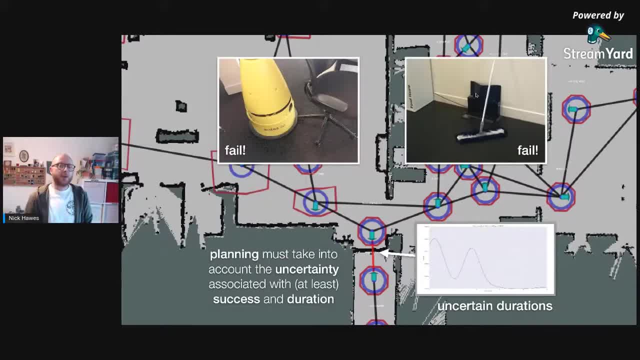 which is pressing the robot's bumper. here The robot can also fail because humans block its environment. So put up here on the right. here you can see a cleaning brush over the robot's charging stations. This is where the robot needs to dock, And if that's there, 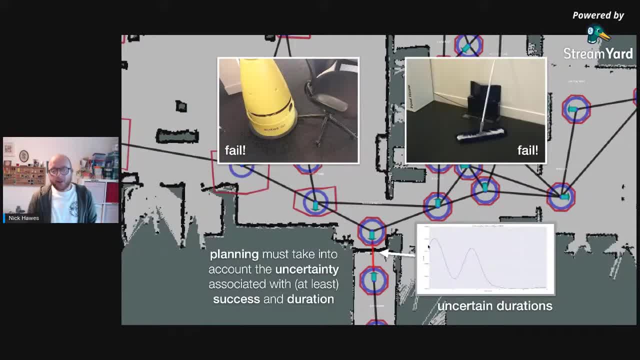 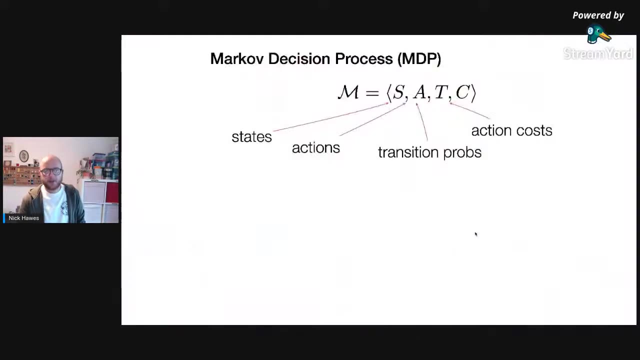 the robot can't navigate successfully. And finally, the robot passes through doorways and we can model the probability distribution of the robot having to wait for a particular duration for the human to open that doorway. So these are examples of uncertainty the robot faces in almost everyday situations. 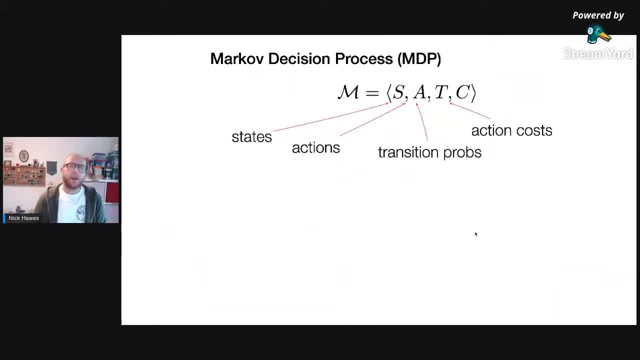 And the way we model that is called something called a Markov decision process. If I had a bit longer to talk, I would go through this in some detail. The rough idea, just to give you a high-level overview, is that we can. 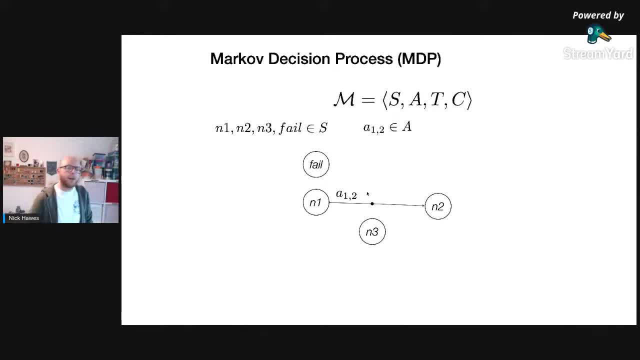 We can formally model the kind of state transitions I've been talking about as actions that transition between states, And we explicitly capture the uncertainty by putting this quantified uncertainty into transitions in this model, And then we can then annotate those transitions with things like costs, which might be time or might be energy usage, And we solve these. 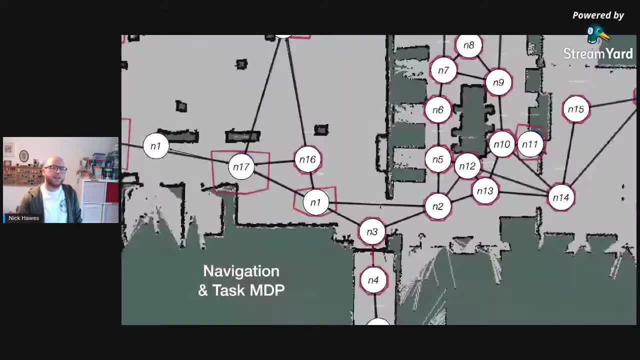 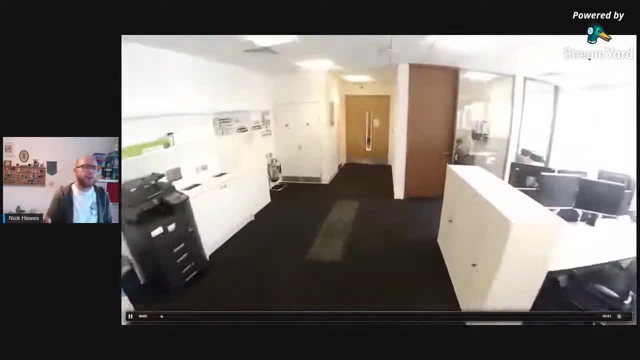 models to get us a policy, And the robot then executes these as it's driving around, And so that shows It shows you that it's this actual behavior that we've created from models like this which is driving the robot around, And that typically means it's adapting to the timings. 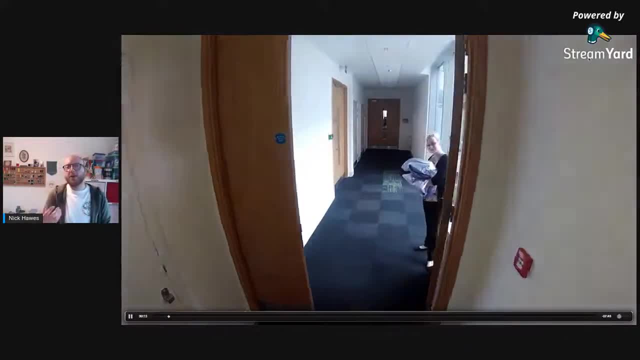 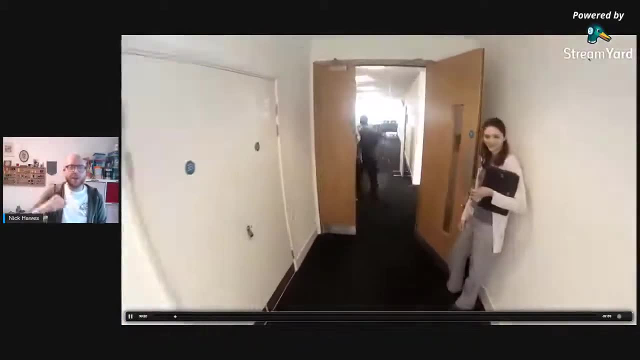 in its environment. So in this case the robot arrives at a doorway roughly when its model predicts there's a high probability of a human opening it, And in this case the robot. This is shot from a robot kind of robot-side view. And again we've got. 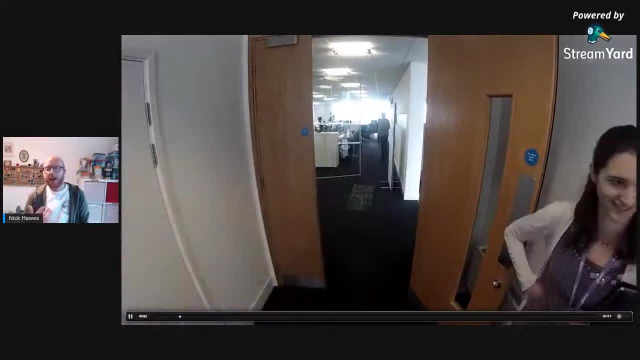 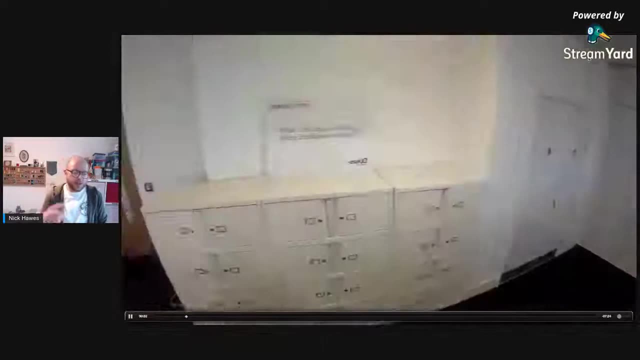 The robot is choosing, in this case, to navigate through the doorways at times when humans are more likely to be around to open the doorways. So it's modeling the uncertainty And then it's using that uncertainty to tell it when it should act in the world to maximize the 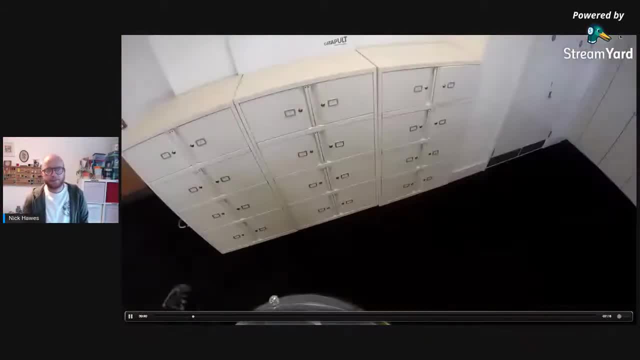 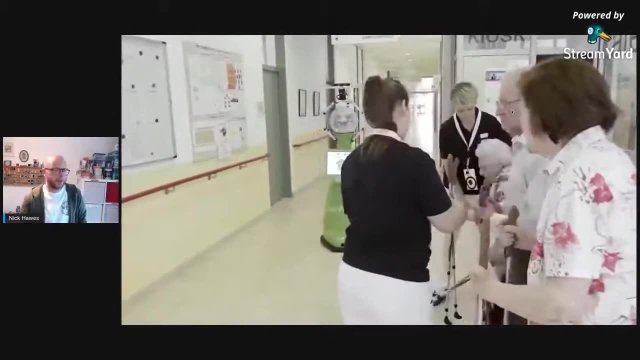 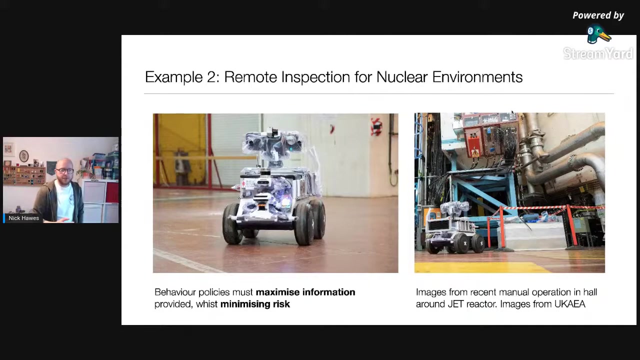 problem: Probability of successfully navigating through this setting. This is an example where the robot had to be somewhere on time to help some nurses walk some patients around in the care home as well. But I don't really have time for this example just yet, So I want to give you one other example from a slightly different context. 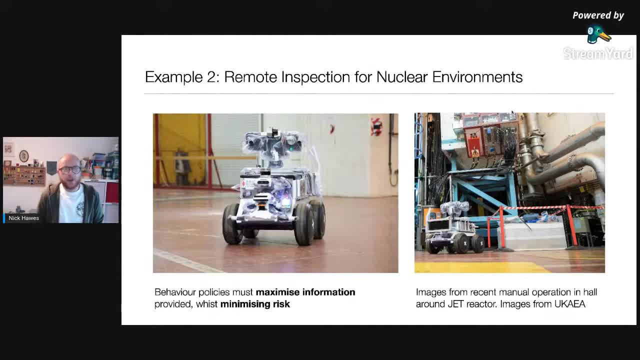 something reasonably close to home. We're working in a lot of nuclear inspection tasks where robots are inspecting nuclear equipment And, as I'm saying, a robot is running a kind nuclear facilities in areas that are very hazardous to humans. The pictures here are from a trial. we 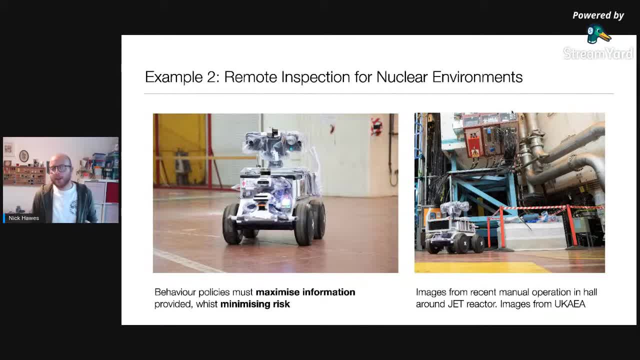 ran last week where we had a heavily customized robot operating. in this case it's kind of remote controlled- inspecting the hall around the jet fusion reactor in Cullinan And these kind of ideas where robots have to work in hazardous environments is something we've been thinking. 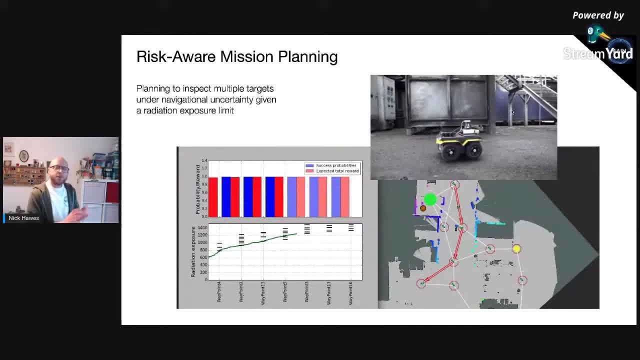 about a lot, So we have actually a slightly different problem. So this is a different setup and here we're using- we're kind of faking the radiation, but we've got this general idea of an inspection robot that must visit multiple targets to gather information without exceeding a radiation. 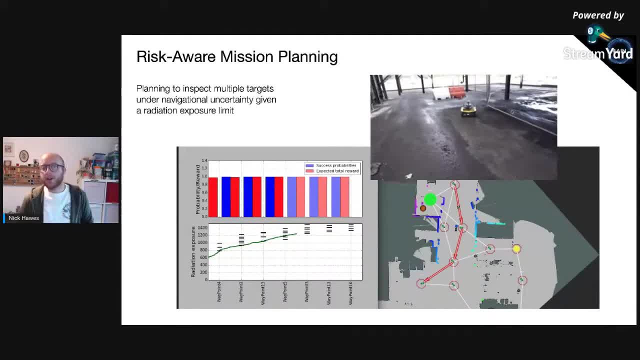 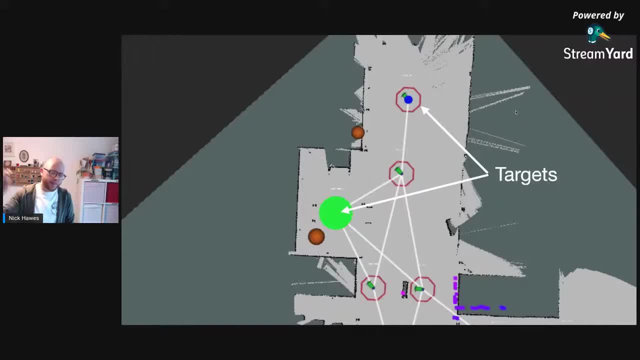 dose, because high radiation doses over time could degrade the components within a robot And we can model the environment a bit like this, So we're going to show you a similar map. So this is another top down view, And these colored disks represent the targets a robot should go and inspect. 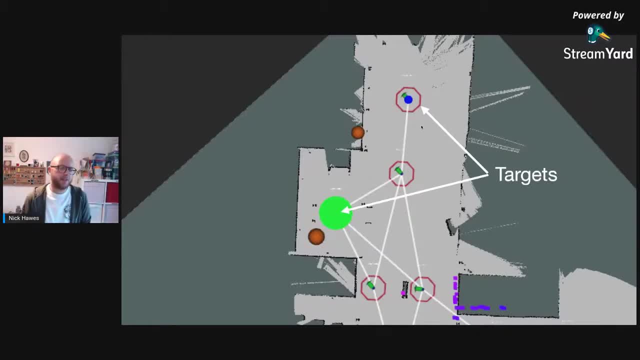 So this is a robot driving up to a location gathering some information. So this is a robot driving up to a location gathering some information on gamma activity, for example, But we've also got some radiation sources And this is a nice example of a multi-objective problem. 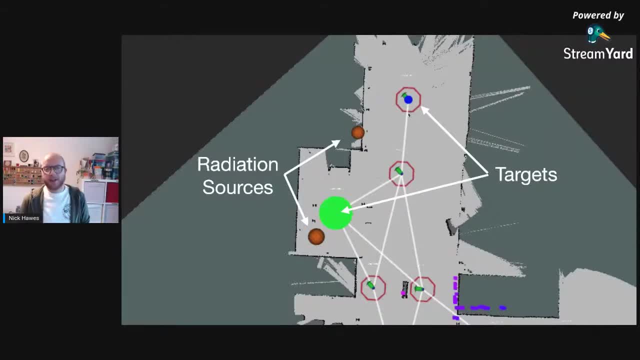 again. We want the robot to go to these colorful locations to get some information. but to go to these colorful locations it has to experience some hazard, It has to go near these radiation sources, And so we think about these in exactly the same way as this kind of multi-objective problem. 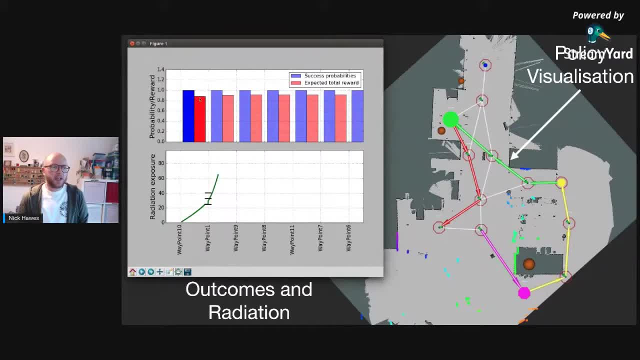 We want to trade off the probability of successfully completing the mission, which we can see in this blue bar chart. That means getting back to the start without exceeding a particular given dose of radiation. And then we can also think about the reward. So how many? 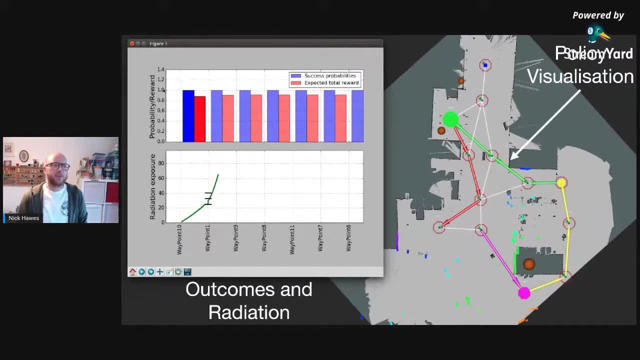 locations does the robot visit, And a reward- in this case normalized reward- of one means the robot can visit all those locations. And so we solve similar problems using the same techniques. We model each action not only as having a duration, but also having an expected dose of radiation And 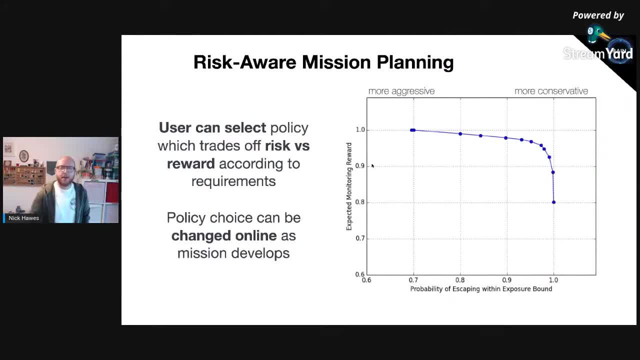 And then what we do is we can come up with one of these Pareto fronts again and we can choose policies from this front. On the left, we're more aggressive. So where my mouse is here, these are policies that visit more locations. 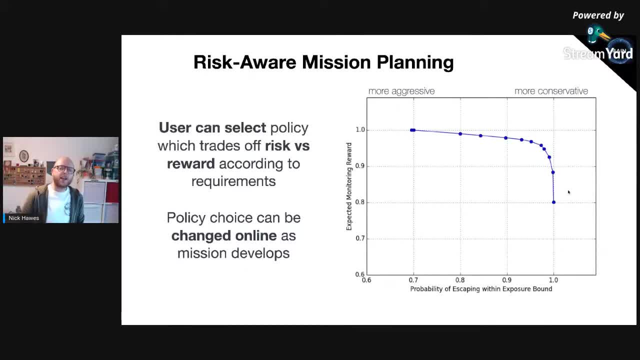 And on the right we're more conservative. So the robot experiences less radiation. But to get less radiation it's also getting less reward And we typically- it's a long conversation- We typically choose something like this, where the robot is getting less reward but still quite high probability. 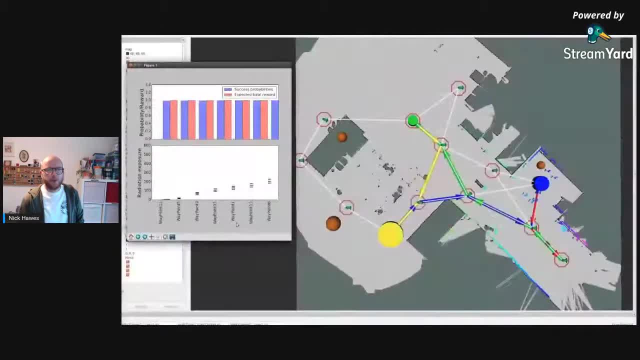 And I'm just going to let one of these. I'm not going to let this one show, I'm going to just run forward. This is an aggressive policy that the robot's running. This is a top down view of one of the examples where we saw the robot driving around in the environment previously. 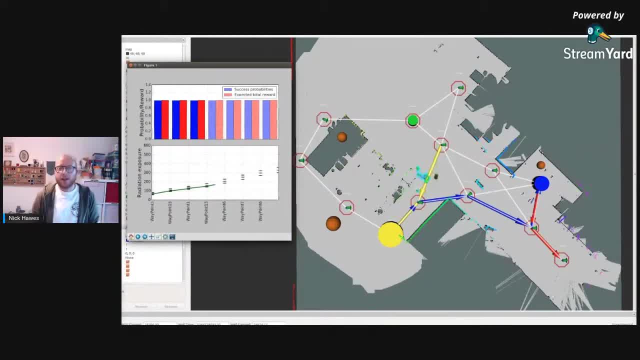 This is sped up 20 times, So the robot's zooming around. This is filmed up in Morton in Marsh, where there's a fire service training college, So this is actually a mock oil rigs- not in a real radiation example, But you can see here we've got some probabilities in this case, even though it's aggressive. 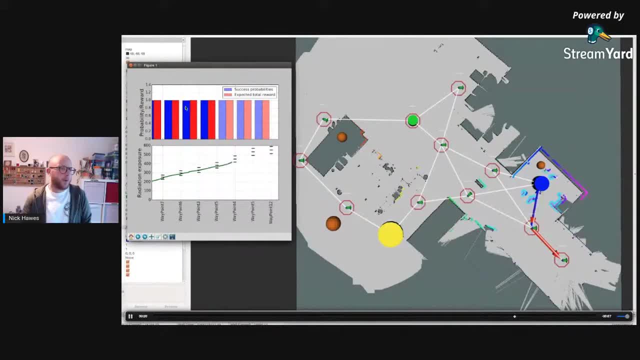 There's still a very high probability of success. So in fact, when I say we're just under one, but that's great, And you can see, here we're tracking a kind of simulated radiation dose. If that radiation does suddenly jumped up high or drop down low, then the robot would respond by changing its policy. 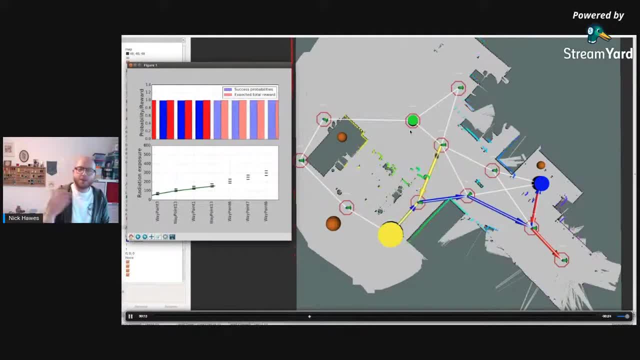 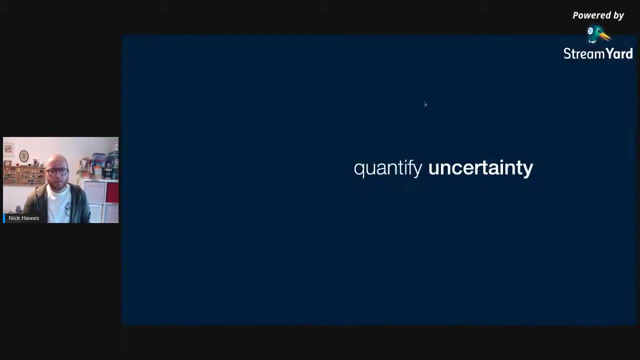 In fact you can see some of these arrows change slightly as the robots moving. That's adapting the policy to the observed radiation doses. There's not super visible on him. OK, so that was a massively quick dash through through the topics that are super close to my heart. 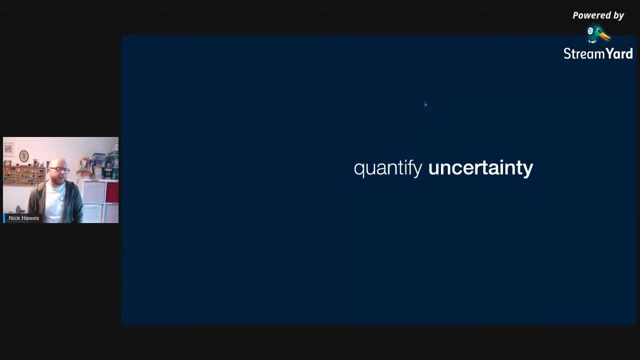 which is allowing autonomous robots to operate safely and successfully in the environment performing tasks for humans, And they do that by quantifying the uncertainty present in that environment. That uncertainty might be a delay in navigation due to it having to take a long time to navigate around humans. 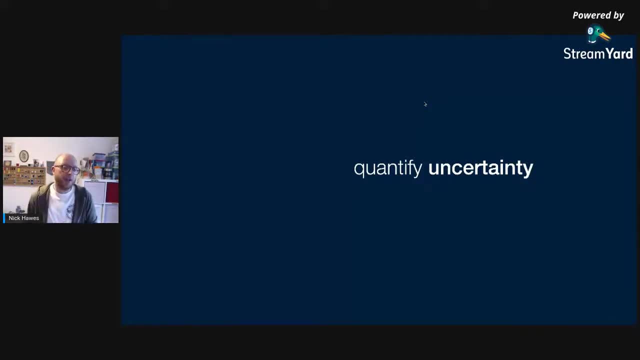 Or it could be the uncertainty could be due to the dose of radiation accumulates through a kind of a real stochastic process. We build models of the way the robots interact with the world. We build models of the systems that say: this is how we expect the world to change. 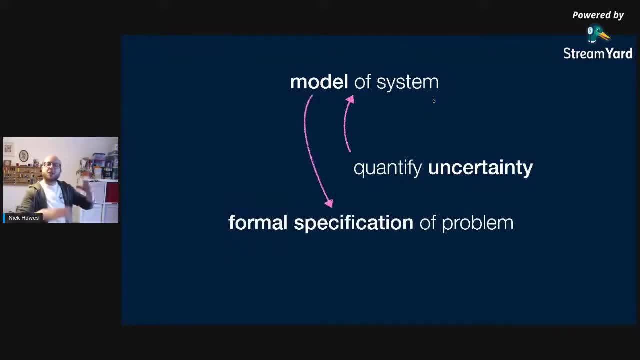 And we factor in that uncertainty and a whole space of things that I haven't talked about, are how we then specify the problem we want the robot to solve, such as maximizing the reward or trading off some information gathering against safety. And then most of the work I do, most of the work my group works on, 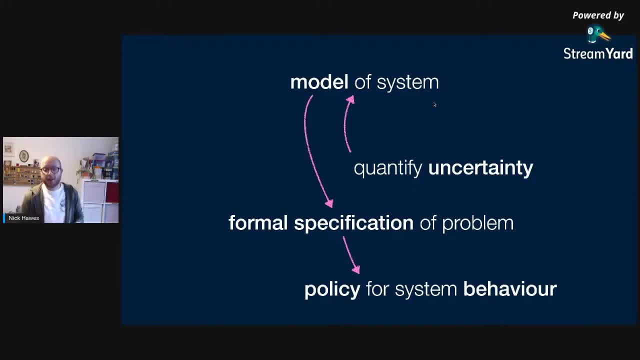 Is Actually writing algorithms that produce these kinds of policies. such the robot displays smart, intelligent behavior in pursuit of that specification. So most of the actual work we do is not about modeling the probability. It's about producing algorithms that solve these problems in order to control the robots at runtime. 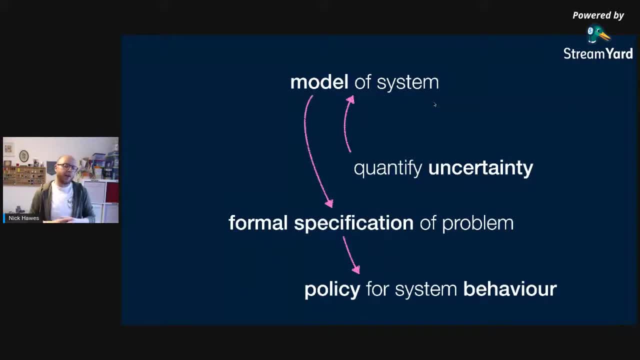 And that's where that's where the bulk of actually the interesting work is. But I think, in terms of understanding what autonomous robots are doing, what autonomous cars are doing when you see them moving around Is actually performing lookups in these kinds of policies to maximize some kind of reward as they move around around the world. 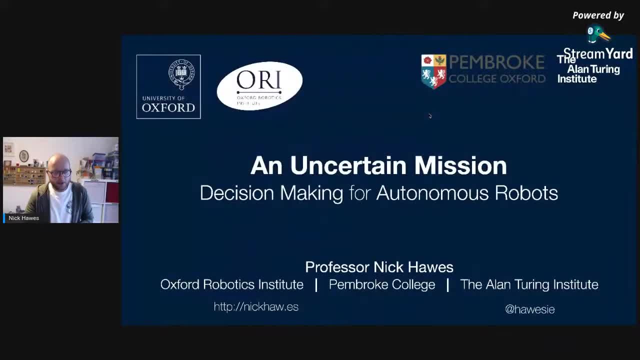 Okay, so that is me more or less done. Thank you very much for listening. I assume something like there is listening and sorry for rushing through it quickly, but I think it's better almost to get to the end and then sort of take questions and I can go back through some of it in a in a more directed way. 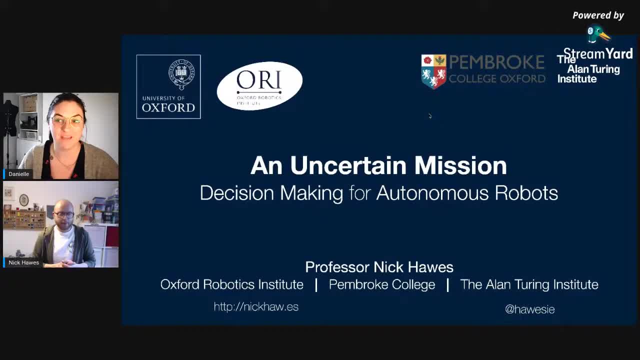 So thank you very much. Thank you very much, Nick, And I definitely was listening and we've still got people on the YouTube channel, So there are people out there that have been listening and yet really interesting And I'm sure you probably could have spoken for a couple of hours on there at least. 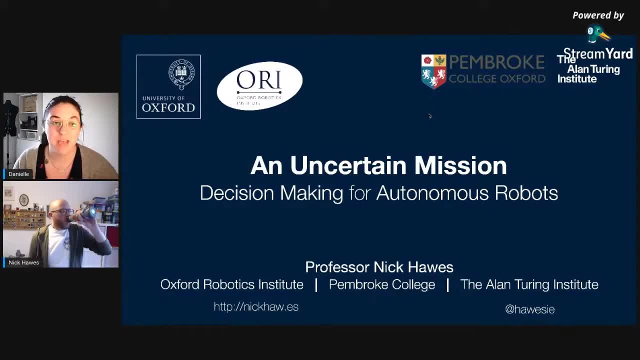 Yeah, that was really, really fascinating. So yeah, if anyone's got any questions, please pop them in the YouTube video. Yuta has already posted a question. She posted it while you were still talking And so I can- I can bring hers up now. 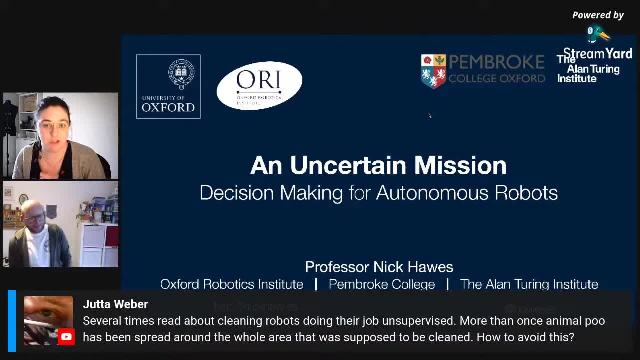 So she says she's read several times about cleaning robots doing their job unsupervised and more than once animal poo has been spread around that was supposed to be clean. So how would you avoid that? Cool, And so I mean that there's there's two, as well as many, answers to that. 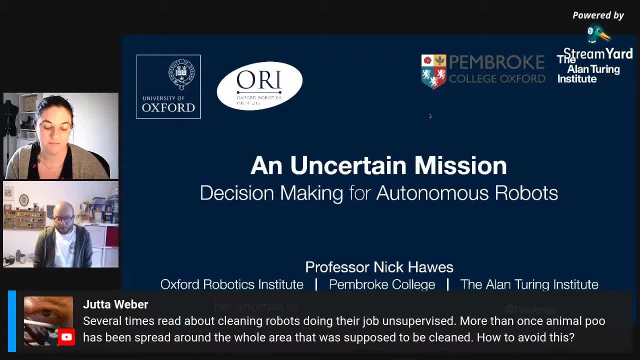 So it's a that's typically a perception problem, So the robot needs to have sensors that allow it to detect There is something on the floor that it shouldn't be driving into. But what's particularly interesting is- I'll ask this from a different perspective, which is I talked about a robot having a model of the world- 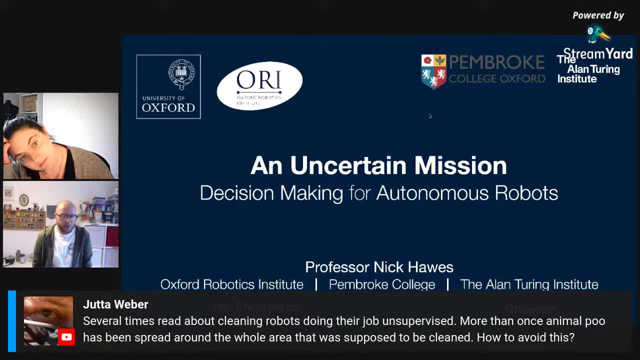 And so when you, when you develop or design an autonomous system, if you want it to be able to use sensors to perceive something and then respond to that thing, you have to include the description of the thing you want it to know about in its model. 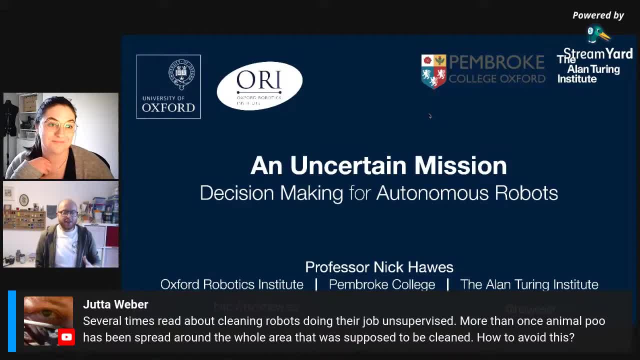 So in this case you have to include the dog poo- Well, the cat poo, In the internal model, in the software of that cleaning robot, and that kind of sounds fairly sensible. but then you start raising the question: where do you stop? 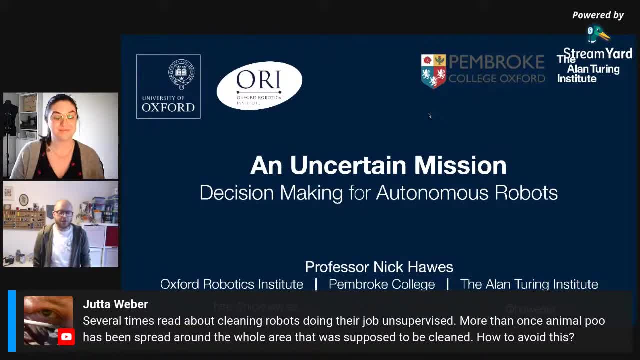 Does it need to know about Lego and cats and children's toys and you know all these other things, And so typically, designers of autonomous systems will draw a line somewhere, It seems. in this case, maybe who was you know it drew on the wrong side of the line. drew the line on the wrong side of that. 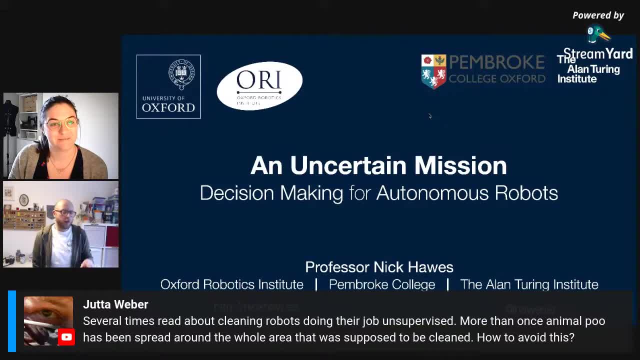 But there's this problem of modeling the world for an autonomous system. Is this massive? It's a massive open-ended challenge And the more complicated your model, the harder it is to produce a behavior policy in any finite amount of time. So this is a tradeoff between modeling, complexity, behavior production and also the sensors you need. 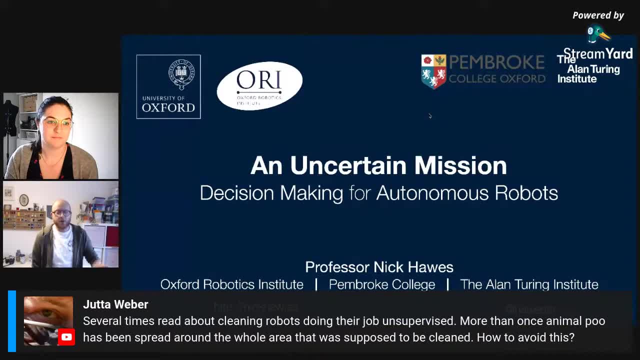 I mean, you know you need sensors then to detect animal poo, you need sensors to detect Lego people's feet, et cetera, et cetera. So yeah, Thank you very much. So we have a question from Neil. 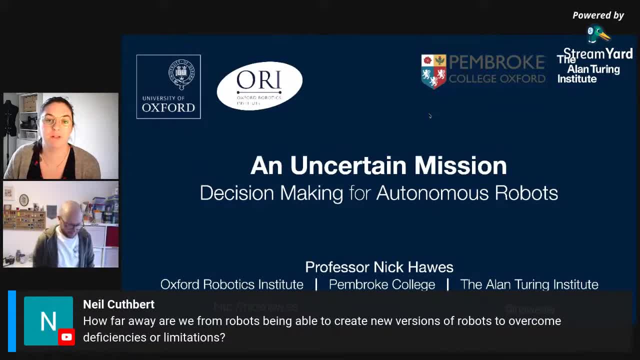 Neil, who asks: how far away are we from robots being able to create new versions of robots to overcome deficiencies or limitations? There's a sort of there's a very trivial answer to that and a longer answer to that. So the trivial answer is: we have it now in that even the robots that I talked about in that video, every time they run, they run. 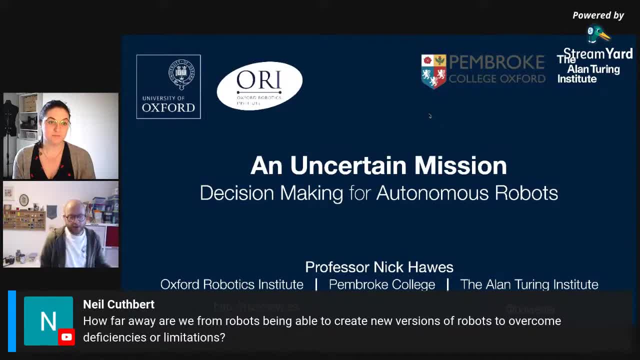 They run, They're gathering statistics. So I talked about quantifying uncertainty. We actually get those measures of uncertainty, those models of the way the world behaves, by gathering data as the robot acts, And so they are creating, and then effectively what happens is they go to sleep, they run some statistical processing and build new models for the next day. 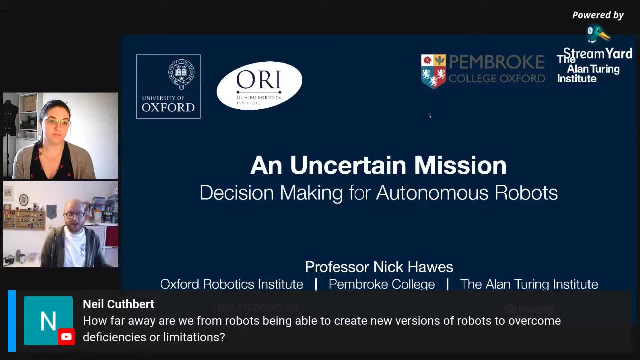 And so they are creating new versions of themselves that act the next day with a little bit more information about the world behaves, the way the world behaves, and they'll be a little bit more reliable or a little bit more robust. So, Absolutely on a on a kind of incremental- I mean it feels like trivial, but it's quite a powerful way of thinking about it. 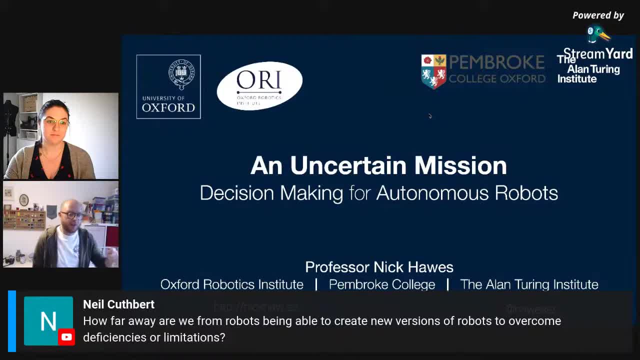 These robots are gathering statistics about their own behavior and improving themselves day by day, And there's lots of different versions of kind of AI methods that do that, different types of machine learning methods that do that, in terms of, of, of maybe the way your question was kind of angled around them kind of more sci-fi. you know, a robot detects a, you know, a limitation, that it can't solve a particular problem. 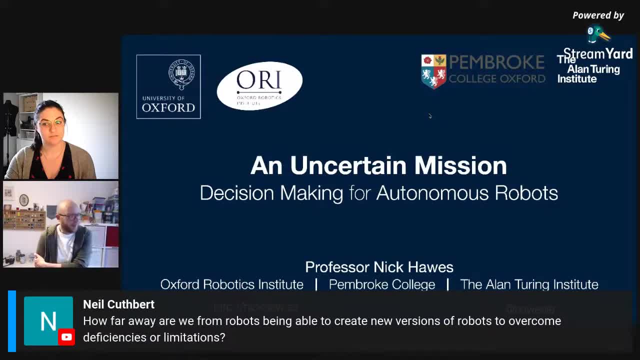 So So it reprograms itself or, you know, build a new limb or something that that has this massive problem that Donald Rumsfeld- Donald Rumsfeld made kind of popular about like knowing the unknowable right. So for a robot to be able to maybe detect that it has failed is fairly achievable. 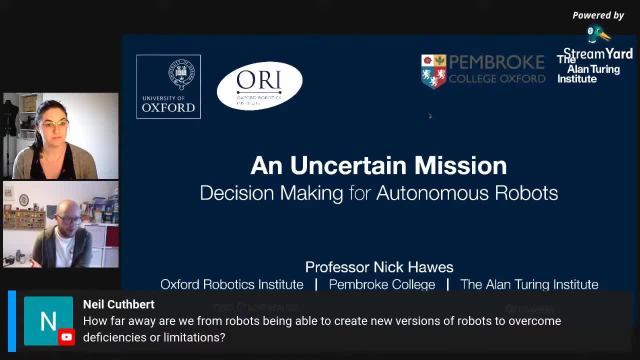 Being able to understand the reasons by which it failed is a completely currently unsolvable question. So you can- actually you can- take it back to the the problem of the animal poo right. The, the robot, the robot is is day after day is happily cleaning the floor. 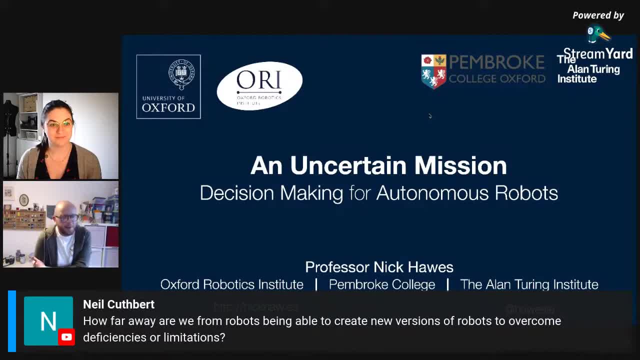 Then one day it gets switched off and told you're never keeping the floor again because it's it's, it's smeared poo everywhere. How is it? you know, what does it need to have in its software to understand it has made a mistake? 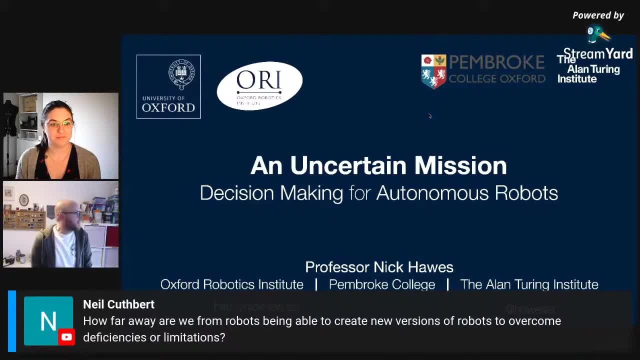 Yeah, And the and, and, and. then to have a robot that could understand every possible cause of every mistake in the world Is is beyond the. I'd say it's not even a well-founded problem in computer science to even formulate that. 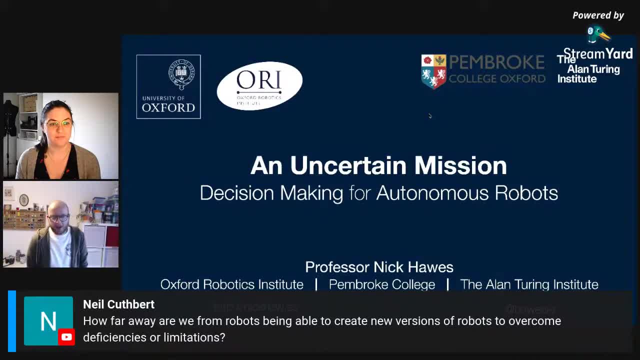 We don't. we don't know how to do that, And so that kind of that's typically called. there's a set of problems that are called big AI or strong AI, which typically means that you, if you, can't solve any of those problems without 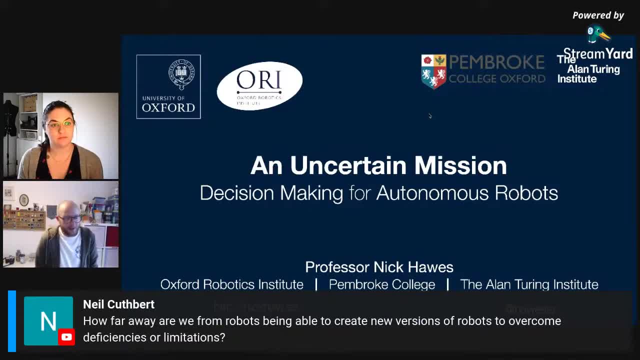 without creating kind of human level intelligence. And we, yeah, we, we're a very long, we're a very long way away from that. Yeah, Thank you very much. So we have a question from Bob who asks: are they using these AI solutions on the? 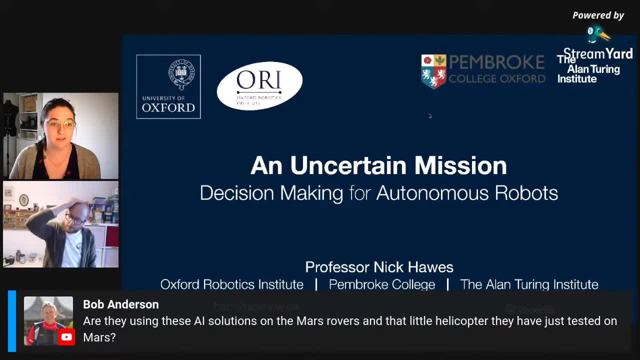 Mars rovers and the little helicopter that they've just tested on Mars. Yeah, Yeah, To some extent, So I don't know for sure what, what they're, what they're running on on the helicopter. That'd be really interesting. 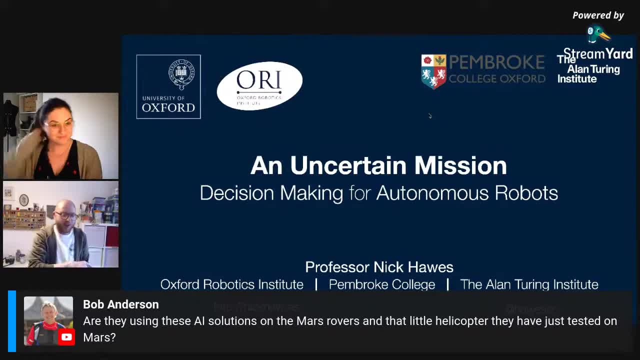 So I see someone I worked on one of those robotics projects, worked on the helicopter, So I've got a slight connection to to, which is exciting- The Mars Rover itself. It's absolutely modeling is is planning its behavior and executing its behavior in that kind. 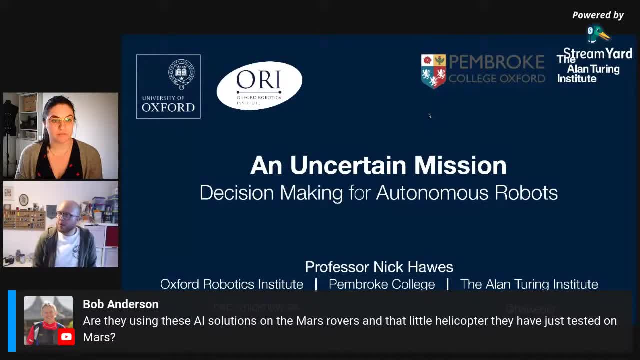 of model. I'm not entirely sure it models the uncertainty that explicitly and it doesn't at least. so I'm not sure what the current Mars Rover. So the pre-spirit and opportunity, the way, the way they worked is they would come up. 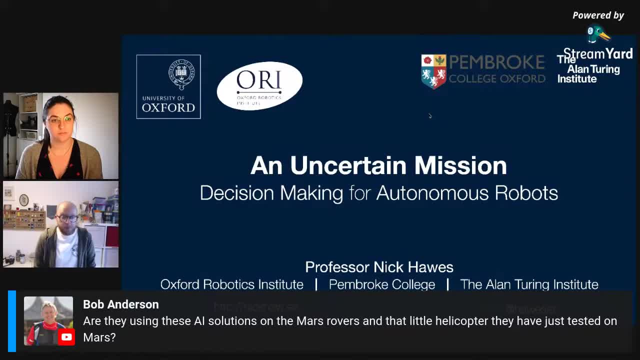 the effectively ground-based software would come up with a mission plan for the day. So there would be a model of the robot's capabilities and a, a, a rough model Of the Martian landscape and things like that, And some AI software on on planet side would come up with a plan which would be: here are the 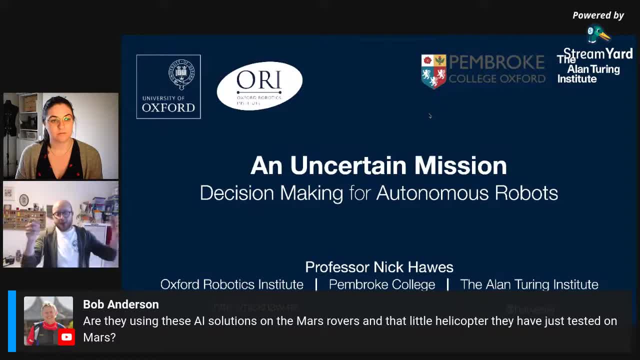 actions the robot's going to perform, And then it was. it's basically it was put in front every day. It's put in front of a room full of scientists who are both kind of robotic. scientists understand whether that's safe- the robot and NASA, planetary scientists, biologists, whatever. 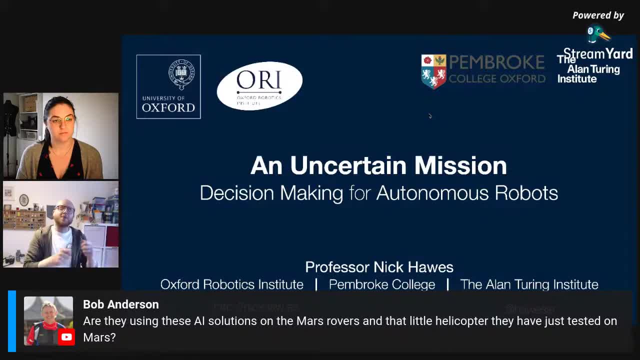 And they decide, if the robots make, if, if that algorithm has made the right choices in terms of the science, And then the humans tweak the plan, then it gets uploaded to Mars. So absolutely this kind of general approach of modeling the environment, coming up with 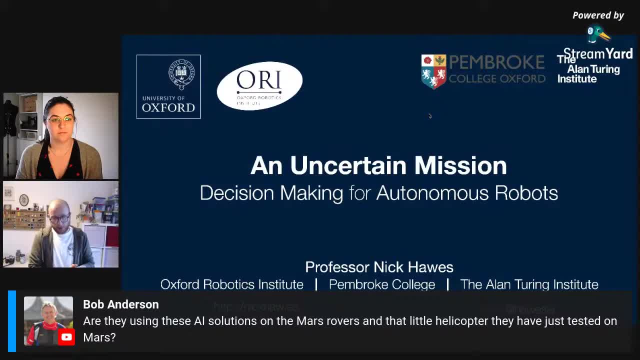 plans that executing them is is being performed on on those kinds of, on, on the on the ground Rovers. I suspect the aerial Rovers are following a much simpler pattern. So if you've got a very, if you've got a reasonably straightforward system, you can, you can effectively. 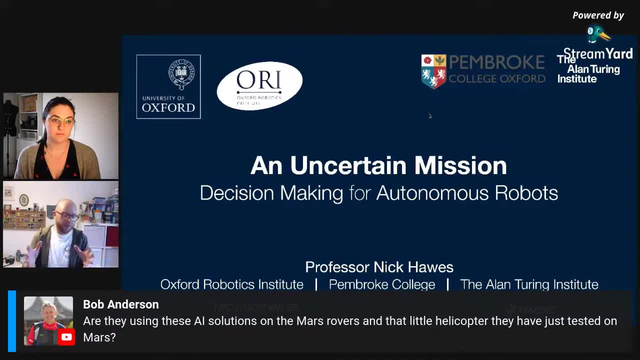 just write a fixed plan that works forever, which might be much easier, Which might be just fly up, fly left land, take a sample, come back And you don't need to know about your environment too much, And then they'll have some, some controllers that stabilize them and things like that. 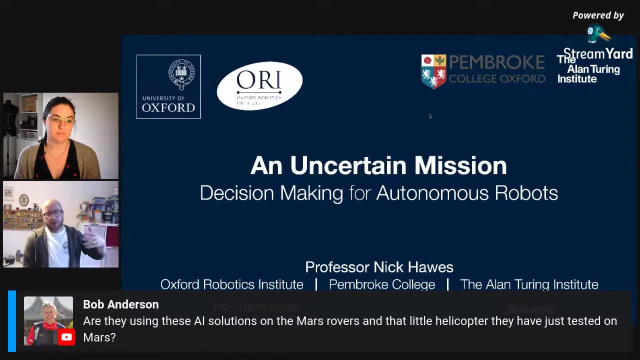 So I would say that certainly the grain Rover is which has got to deal with long-term autonomy, has to be like long transits across Mars. We'll be using a model of its behavior and its objectives, but with a human in the loop deciding whether that's actually safe and the right thing to do, because these things are. 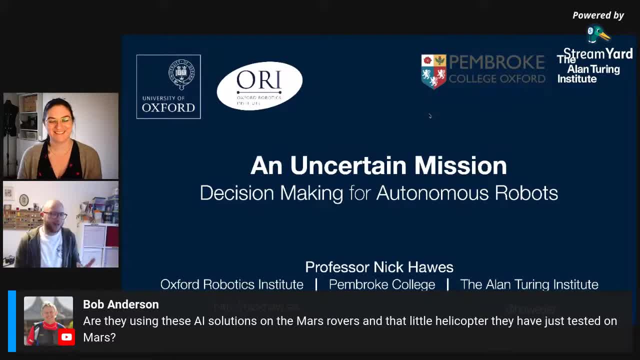 super expensive. You don't want to mess up. And then The, the, the little helicopter. what's the helicopter called? It's got a cool name. Sorry, I put you on the spot. Is it perseverance, or is that the Rover? 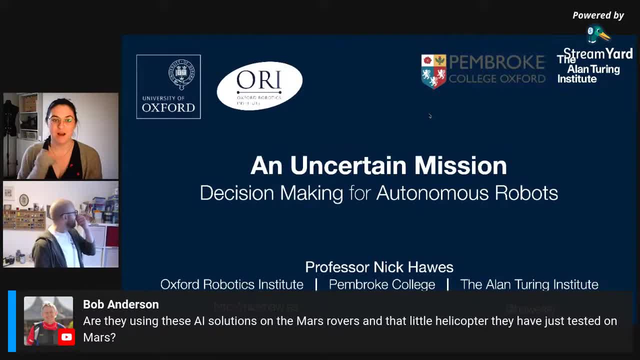 Perseverance is the Rover. I'm sure one of our audience members can remember what the? Yeah, Someone can Google it while we're talking. Anyway, I suspect that the helicopter is using a much simpler behavior structure. Okay, Thank you very much. 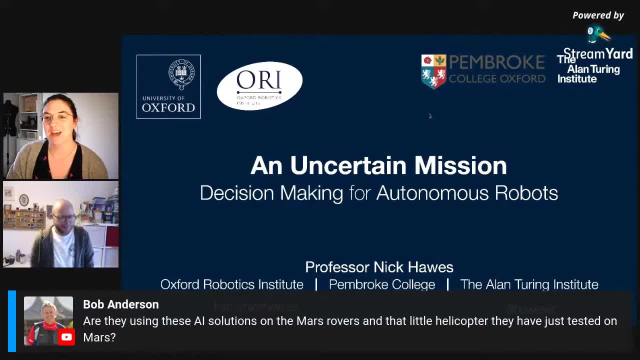 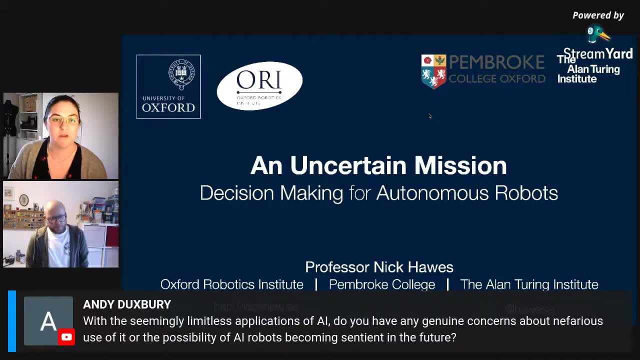 Yes, Ingenuity, You have to confirm, Okay. Thank you very much. We've got another question here from Andy, sort of links back into what you were discussing previously. So, with the seemingly limitless applications of AI, do you have any genuine concerns about? 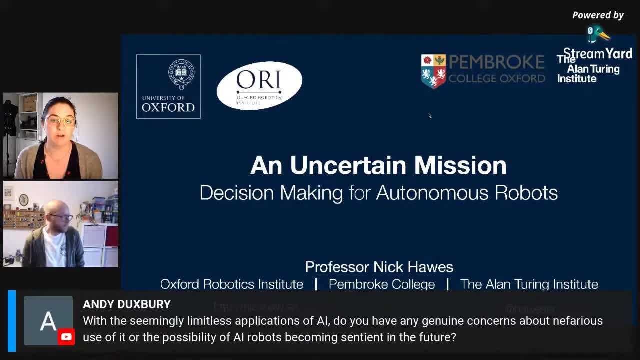 nefarious use of it or the possibility of AI robots becoming sentient in the future. So I, I, I mean the I- I- I have genuine concerns about nefarious uses of AI because it's happened already. right, There's, there's lots of. 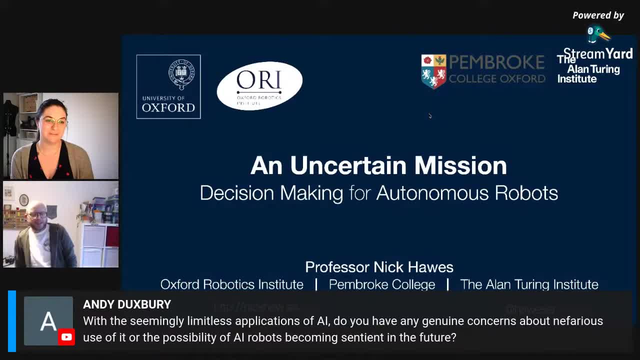 Evidence of maybe, maybe, maybe not nefarious but damaging uses of AI. So people have been using kind of machine learning systems that are racially biased. There are sentencing systems that are biased by the data you give them. So these are systems that are not nefarious in themselves, but they're being used by humans. 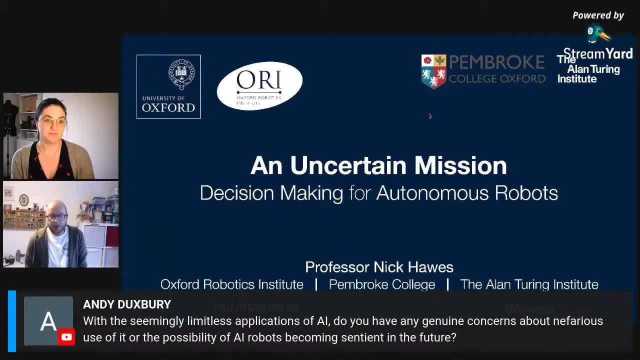 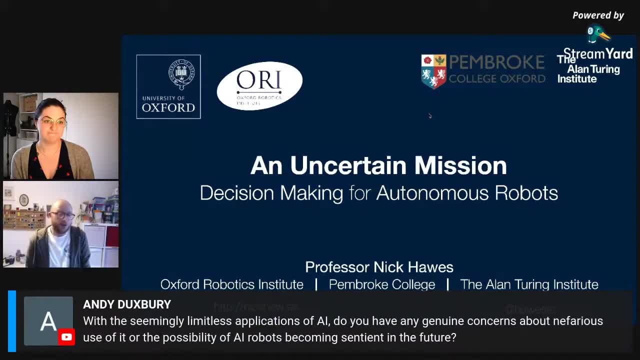 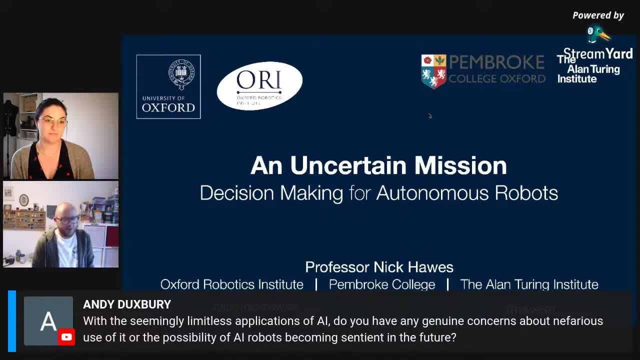 Yeah, Yeah, Yeah, Yeah, Yeah. It's like I have genuine concerns about nefarious use of AI, because you know it is happening and it should be legislated against. whether that's AI or whether that's just technology in general, I think is is an open question. 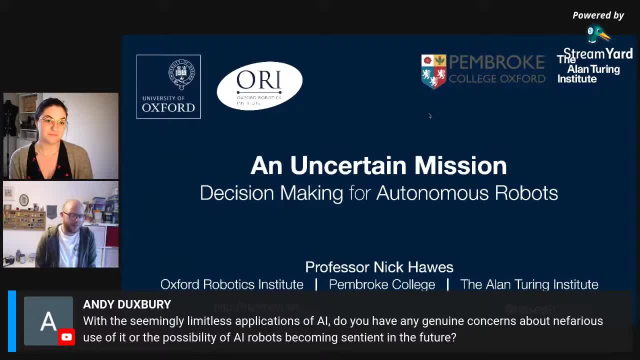 And AI is part of that suite of things around big data and connectivity. That's enabling some nefarious behavior, Um, So possibility of AI robots coming into the future? I'm much less worried about that. I think that's a red herring. 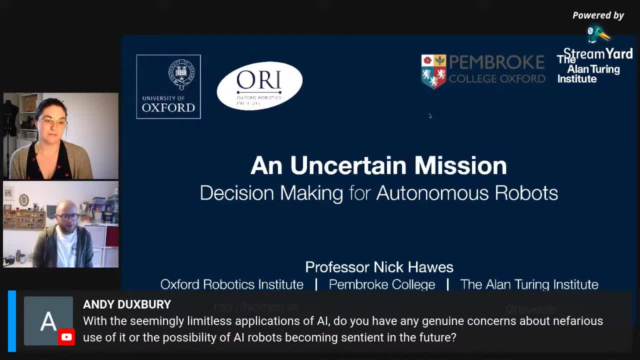 It's just that there's no. as someone that spent my life programming dumb machines, I just don't see that. I don't imagine a world in which you suddenly write one more line of code and the system changes from being kind of this dumb input-output thing to something that is more than the sum of its parts in some way. 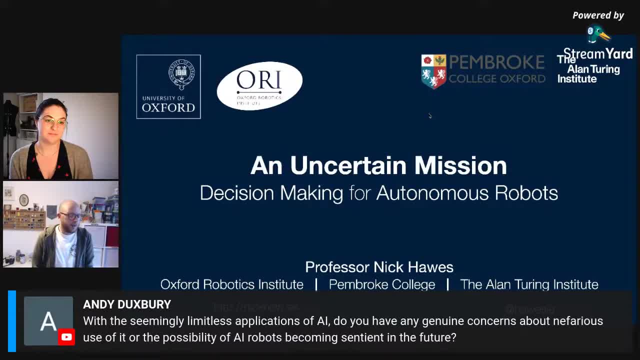 I also take humans as an existence proof that an engineered system can be sentient. So you know, it has to be possible for this version of, at some point, machines just sit there for long enough and then become sentient. I'm not sure. 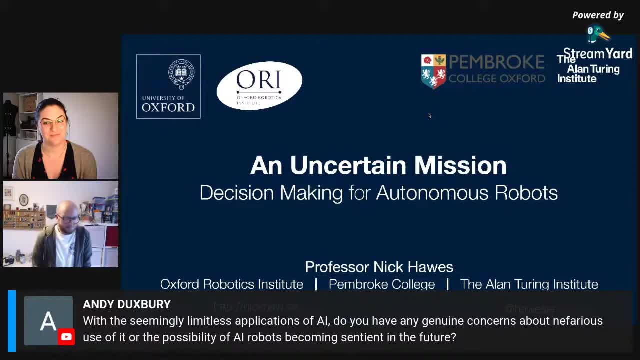 And I'm not sure how we get there by engineering either. Maybe we'd need a more thorough understanding of our own intelligence before we can start implanting it upon other things. I would say we need both that and a more formal definition. We need a more formal definition of what we consider sentient. 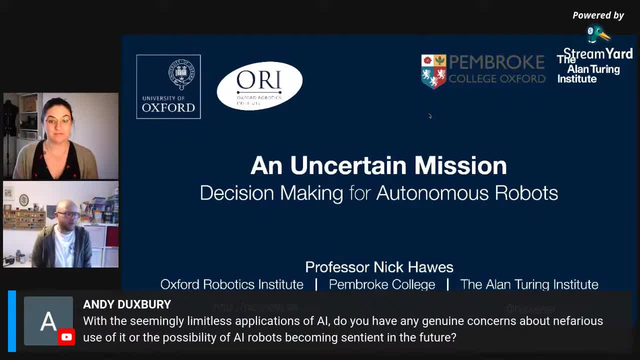 So I think that we like for things like consciousness- we don't necessarily have a good definition that we could- then we could reproduce in a machine and be satisfied with, And people are actively working on that and there is progress in that direction.